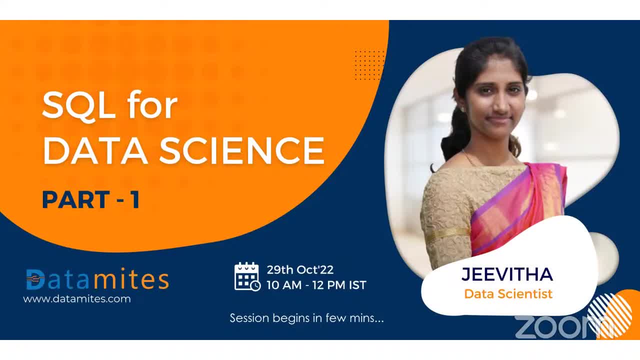 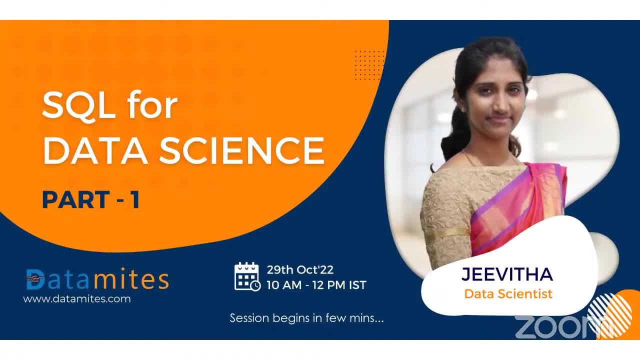 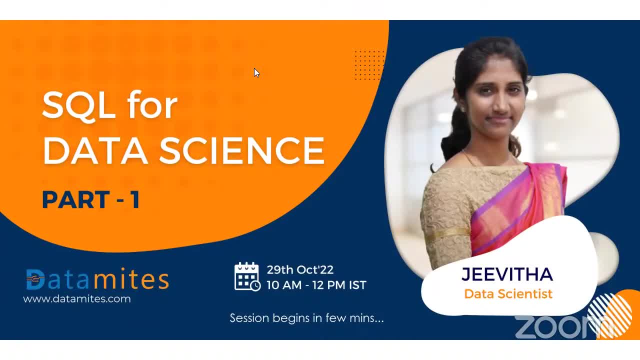 hey, good morning. apologies for a couple of minutes late, all right. so today we have uh um jivita presenting sql for data science. this is going to be a a four-part session. uh, two hours each, so eight hours together today and tomorrow and then again the next saturday and sunday. um jivita is a data scientist with rubix. he is active. 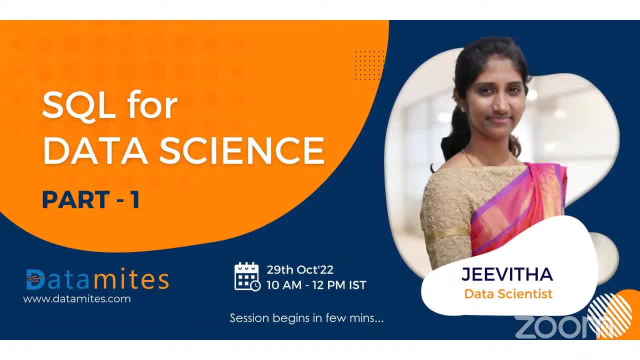 in many projects as a data scientist and also delivered sessions for data science sessions for more than uh 200 people and um a very active enthusiast in in data science research as well. we have jivita today to uh to deliver this session. sql for data science. before i hand. 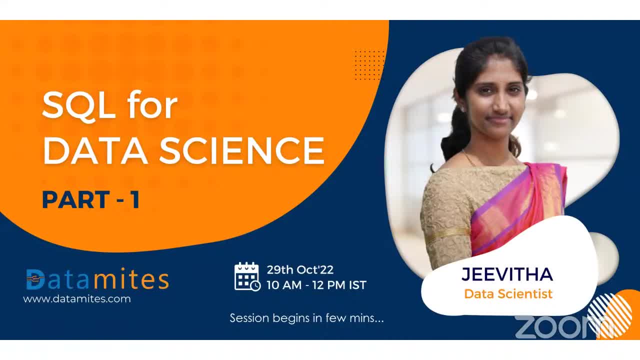 it over to jivita. um, a bit about sql. you know sql is a structured query language. it is the language, or the um, you know, basically a language we, um, we use for, uh, talking to databases. so when you look at the um, you know data science has a data as a, as a main part. so it's all begins. 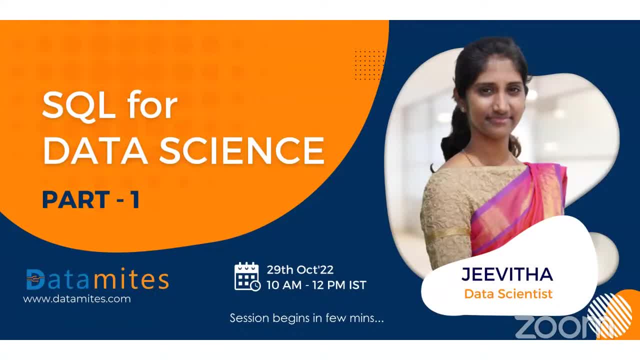 with bringing the data into our- uh, you know, into our project. about 70 to 80 percent of the business data right in any industry, any, any company, is actually stored in a structured format, which is sql format, and we use relational data science to deliver data to our projects. so this is a very 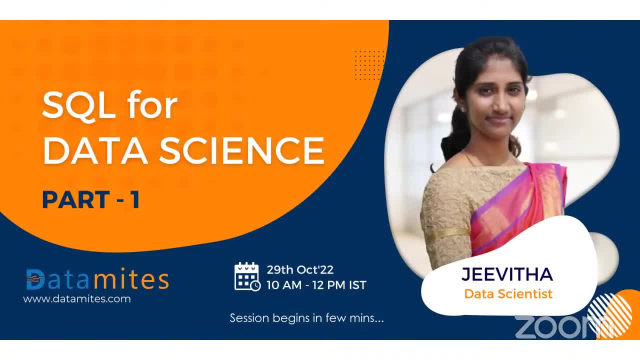 database management system to handle this data well. popular ones are Oracle, SQL, Microsoft SQL, well, my SQL, open source as well. so these are the kind of databases you deal in in a business project, usually all right. so, um, it's really important to know the sequel to to, to, to get. 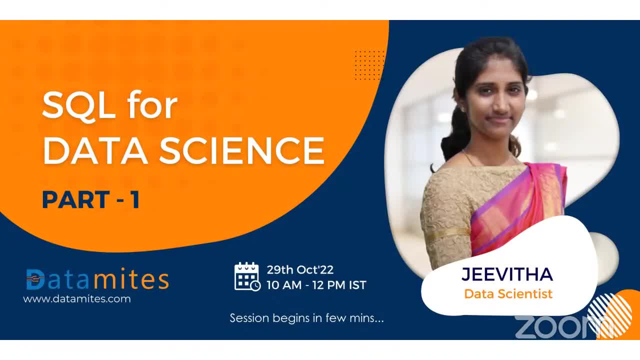 this data into your, into your pipelines and to to do the data science work. in a typical data science, in typical database management, you, you do crude operation: create, read, update and delete. as a data scientist, you are mostly concerned about reading, because you really don't create the data, the data. 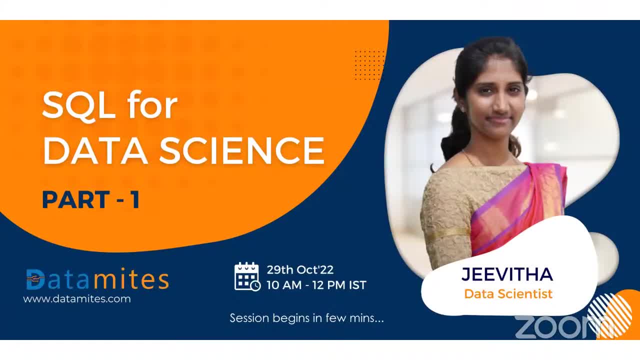 is already there in the databases, right? it is put in there by the business applications, right, updated by the business applications. what you do is read them and do your. you know your project, right? maybe a predictive analytic model, Etc. etc. so we are mostly focused on reading the data. 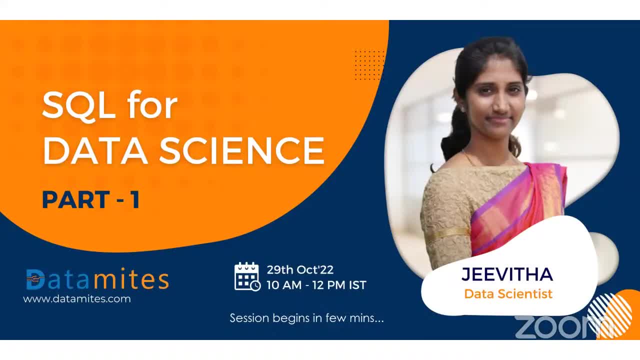 and more precisely, effectively reading the data, the data you want, with all kinds of, you know, the filters and the conditions and the and aggregations, Etc, Etc. so this session is going to be mostly focused as sequel forина data science perspective, So we'll be also discussing about other operations. 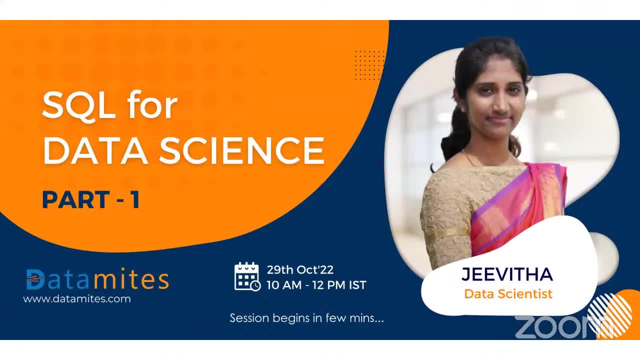 but 80, 90%. focus is how to connect to the databases, how to bring in the data to our pipelines, data pipelines- and then how we will basically apply different conditions and bring in the data- different joints from different tables- bring in the data. 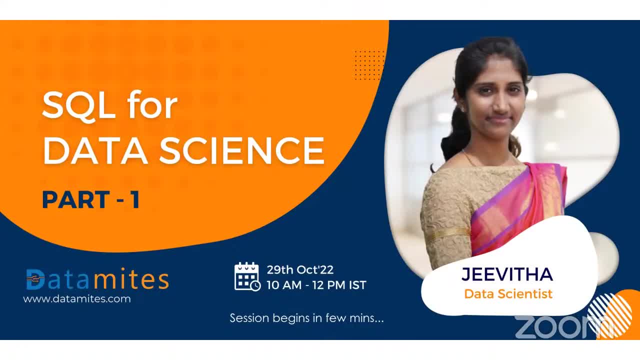 to for our data analysis purpose. So that's going to be a session. I thank Jivita for taking time And, yeah, all the best to everyone in this learning SQL for data science. Over to you, Jivita. Thank you, Sho. 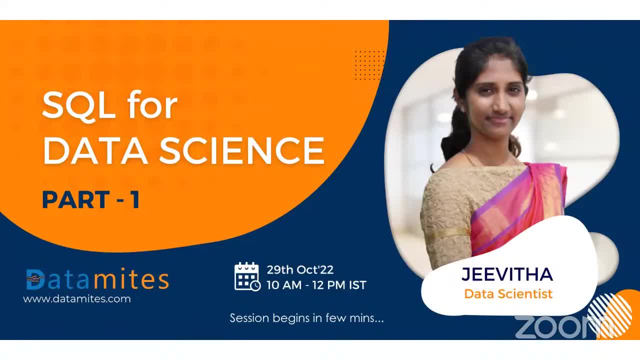 Hey everyone, Good morning. Welcome you all for the SQL for data science webinar. Myself Jivita. as Sho said, I'm working as a data scientist as well as data science mentor in Rubik's company, as well as the partner. 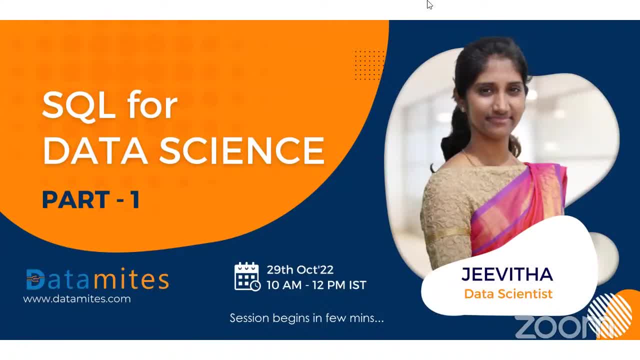 of the company of Rubik's that is DataMinds. Are you the one who is aspiring to become a data scientist? Are the one who has learned all the skills related to data science, but still you lack in data. I mean, still you lack in SQL skill. 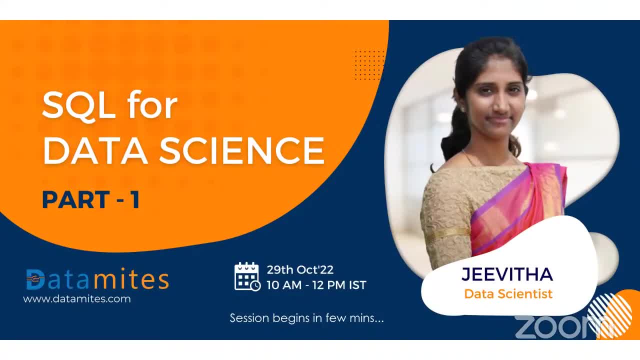 Then this webinar is basically for you. You know, nowadays SQL is one of the most popular in demand skills in the market. I don't know whether you know it or not If you see recent job postings on LinkedIn or probably in different job portals. 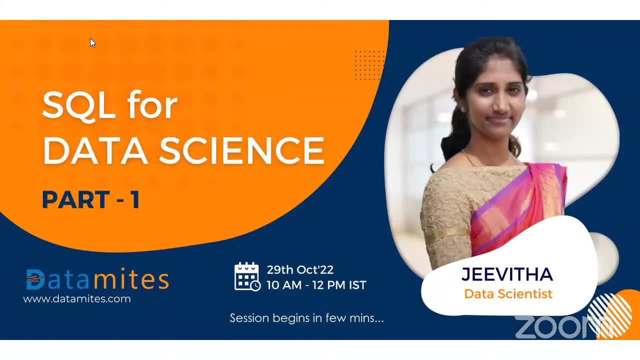 like in the now Cree, You can see every Job. sorry, every job posting will be mentioning a skill related to SQL, But sadly, you know, SQL is one of the under-depreciated among the top skills that is required by data scientist. 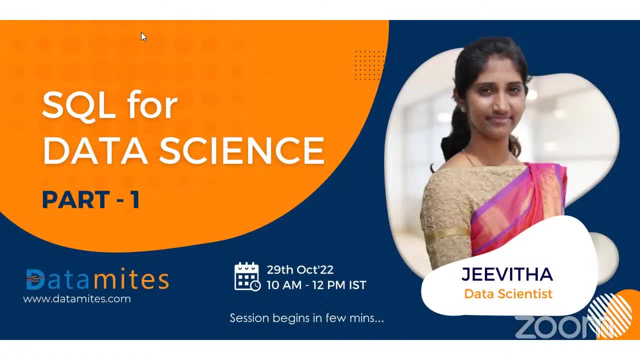 not just in India, even the worldwide. That's really an insane thing And you know we could see many are aspiring to enter into our data science domain. many, many people from different domains minds are getting into this domain And the thing is people just only focus on learning. 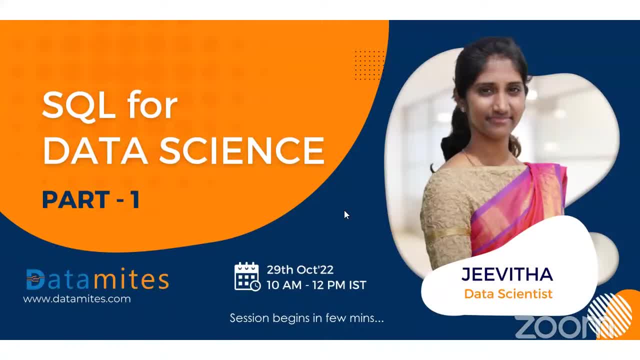 things related to machine learning and just the Python. They think these are the only two skills in order to become a data scientist, but that's not the real thing When you see your data. as long as you see data, the SQL will always be an important thing, and you. 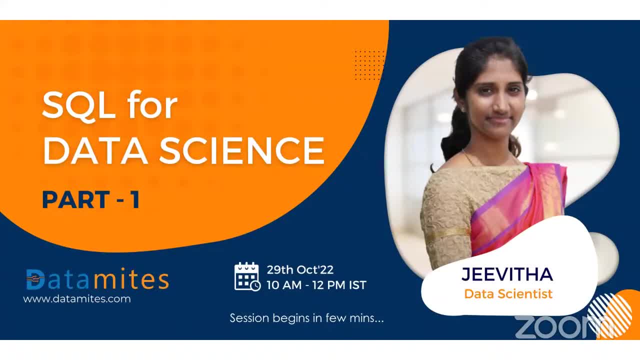 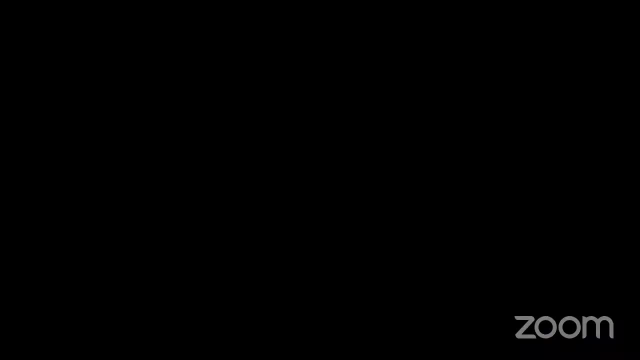 have to learn the skill. Okay, Jivita, could you share the screen? I think still is my screen. Try to share your screen. Yes, I'm seeing I can still see mine. Okay, Can you see my screen now? 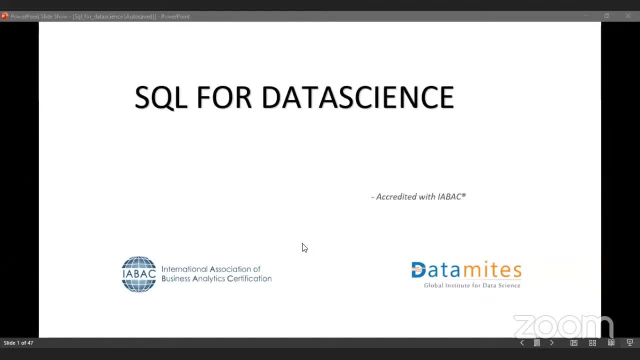 One second, Yep. All right, Good, Thank you. Thank you, Yep. So let's begin the session. So this webinar is basically happening for eight hours. We'll be focusing more on the things that are relevant for data science And also some topics can. 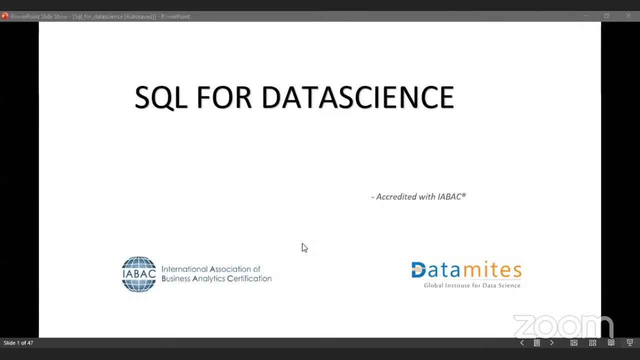 also be used by the people who are looking into a data analysis thing. So, firstly, let's discuss a few things like how data has evolved, how database has evolved, all those things. So for this entire session- I mean for two minutes- I'm going to be talking about the 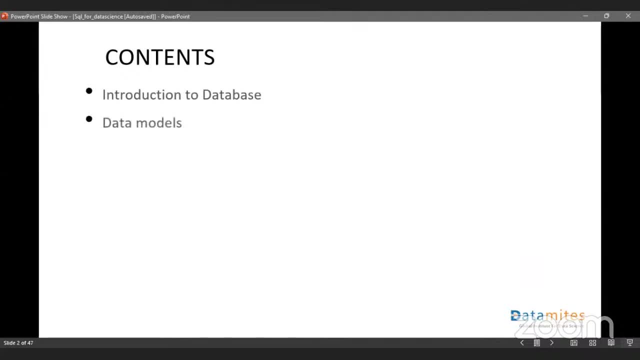 things that I'm going to discuss are like introduction to database data models, RDBMS and its types, And also I'll be giving an introduction to SQL, And then let's see how to do installation of MySQL Workbench, And then let's see how to create a database, and 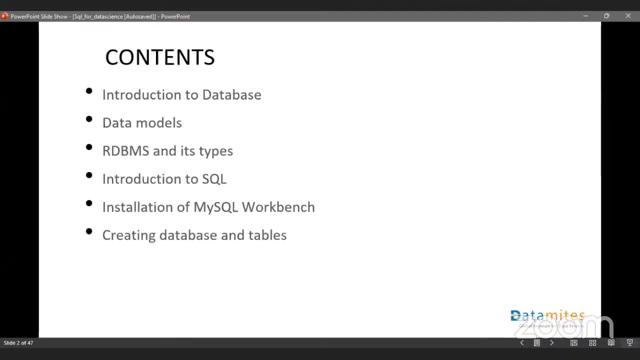 tables. Yes, this topic is not that important, but still it's good to know, Okay. And then, finally, let's see how to alter, how to modify tables. Okay, So these are the topics that I'm going to discuss for this. 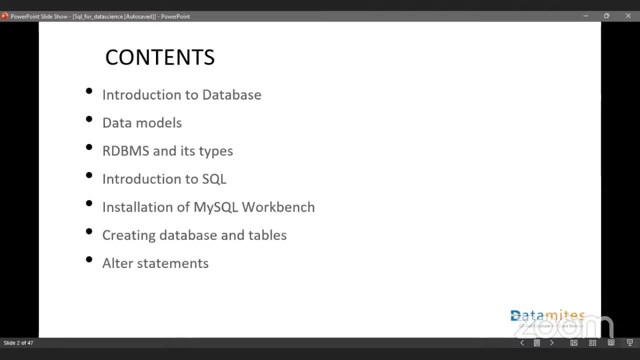 So let's start with the content. So I need to start this question with: sorry, I need to start the session with a question. as we know, data, So data science is all about our data. So data can be of a different types. Yes, data can be a text, data can be a number. 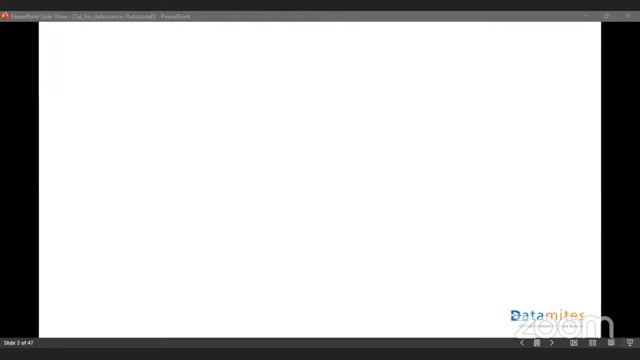 data can be images. data can be video, audio. yes, okay, we have different data and we can take all these data from different sources. let's imagine, uh, somewhere around, like you know, 50 years ago, how data was collected and how data was managed, any idea? so, like 50 years ago, if you think about like, if you have seen or if you have? 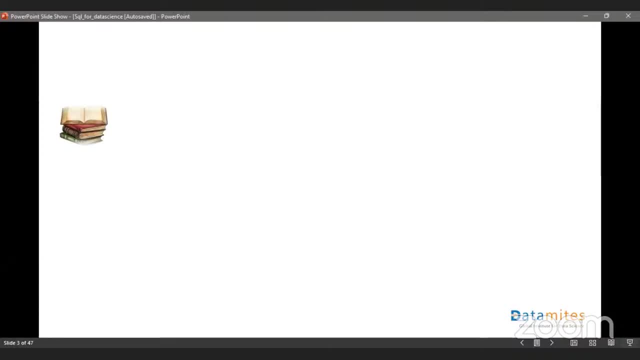 read in books like, basically data was collected, like there was no technology, there was no, you know, smartphones, there was no internet. during those days, people used to collect a very simple data, like it was not much data. they used to collect data and the basic and the traditional. 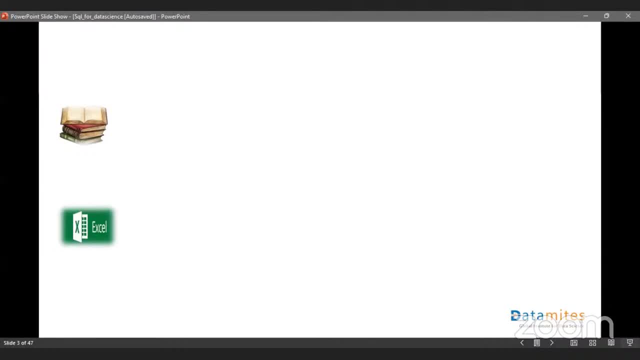 method of storing data was, you know, by storing it in a box. and the second method, the advancement of this, was like excel. you can ask your mom and dad, like 50 years ago, somewhere, like you know, like if you take an example of a university, all the details of students were stored inside a book. 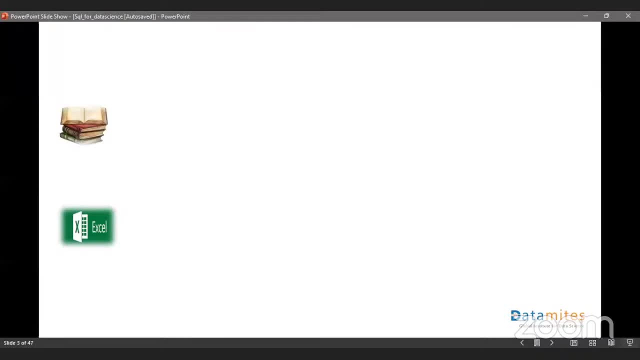 now we have all advancements, like we store everything in our computer and we have different databases. yes, no, so this was a traditional method, uh, which was used by the people of you know, like people like before five decades, like they used to store data in a box and excel sheet. after that, when the emergence of technology came into an existence, that means 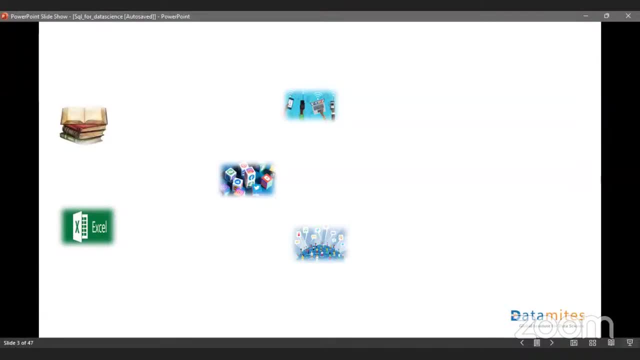 when the concept of computer, when the concept of mobile phones, internet, social medias, so when these concepts have been evolved, when all these you know technologists, when they came into a market, people started using them, and then the real challenge just started. what is that real challenge? it's basically, you know, when people started using internet, people from different. 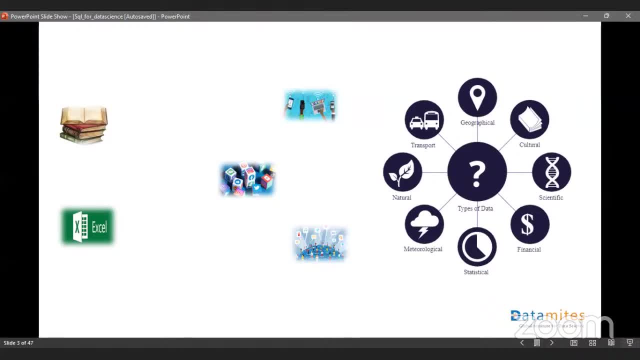 domains. like you know, starting from sales, starting from business to mine, to our medicine level- people started gathering information from different sources. so when they collected massive information, they faced a challenge, like you know, how to store that data and how to manage that. even security is one of the important thing, so people have 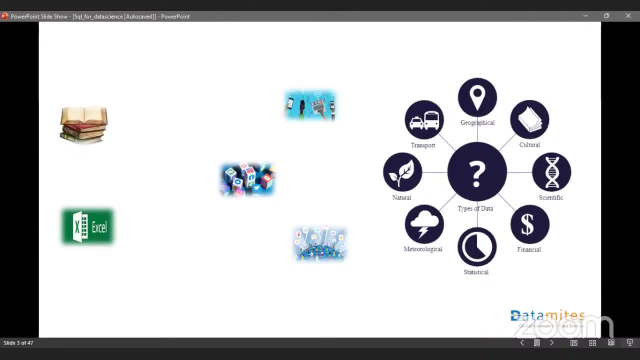 invested their time in collecting the data. once they have collected it, now it's a question like how, how that will be stored and how that data will be managed. so how do you do so? all those massive data can't be stored inside of books. it can't be stored in excel or a spreadsheet. so then the 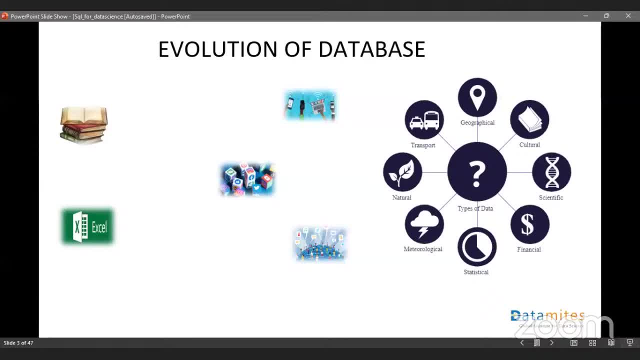 concept of database has come. so people looked at like you know what to do, how to manage these things, how to store. so then they started working on, you know, creating a framework in order to store data. we called it as a database. so this is the concept of a database. so this is the concept of a database. 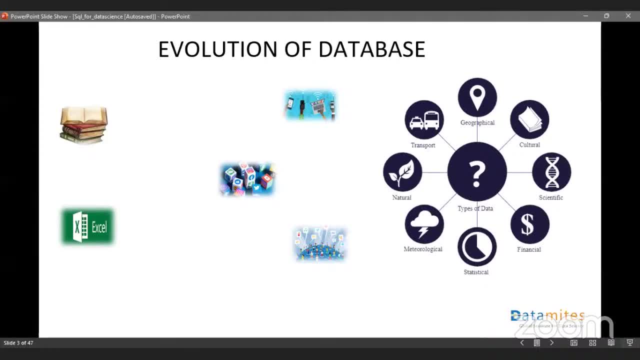 is how evolution of database took place in 1960 itself, when computer, as when the uh, when the technology of computer came into an existence, the people started storing data in single file. and then uh, that advancement was done by ibm, so they've started one more. and then again. 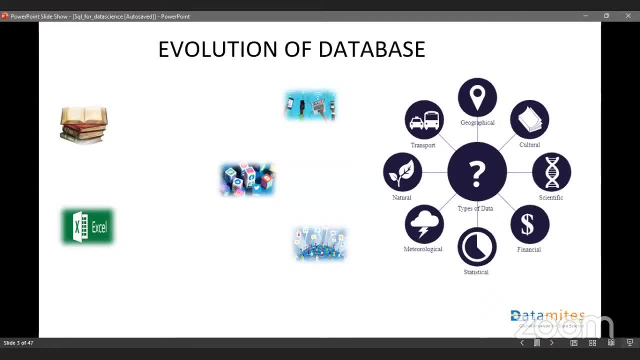 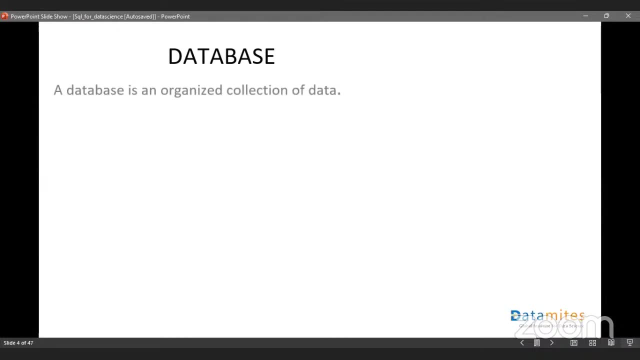 continuously, gradually, many databases were invented by people, and- and there are many databases in the current market as well, so- which are basically used for storing data. all right, so now, what is database? you know, database is basically an organized collection of data. what do you mean by that? 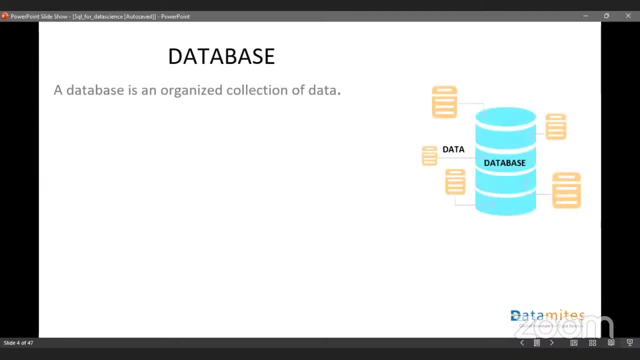 so database basically acts as a container in order to store data. for example, let's take a university. if i take a university, universities basically collect information related to our students, related to our faculties, admins, staff of different colleges. if i see a university, there will be hundreds and thousands of colleges under that university. 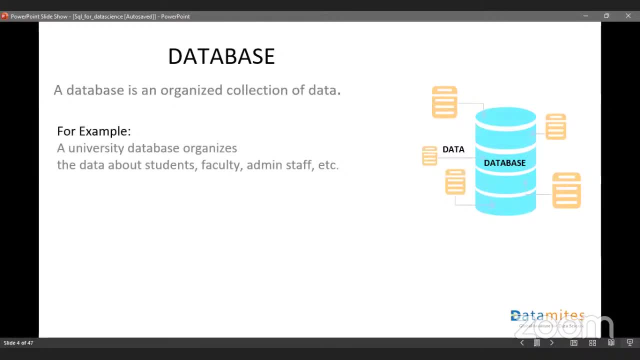 right. So that means it will have a massive data. yes, How that entire data will be stored, Like, if you think about, like 50 years ago people used to store entire data inside of books And now it's not that very small data, it's a massive one- can't even imagine about. 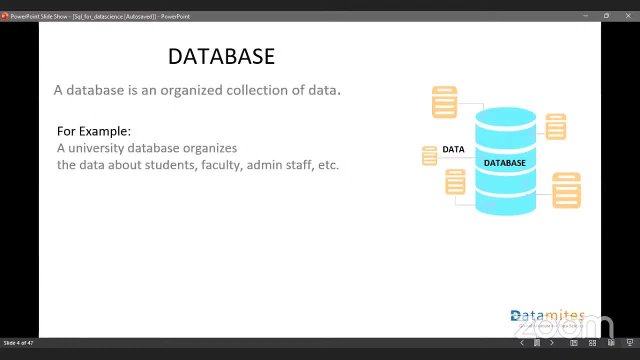 that you know data things. So then a concept of database was introduced where you can store all the data in a structured way. Clear about your database. Database is basically a place where you can store data. It's an organized collection of data. Okay, database it basically. 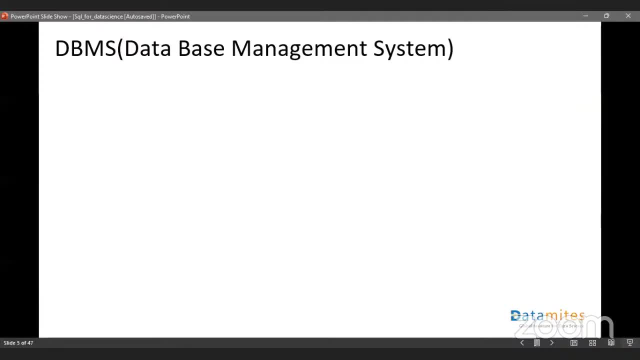 acts like a container where you can store data. Okay, that is fine. Now the question is: like, how do you store, Like something has to be there, right, In order to store that data, in order to link that, in order to link data and a database? there should 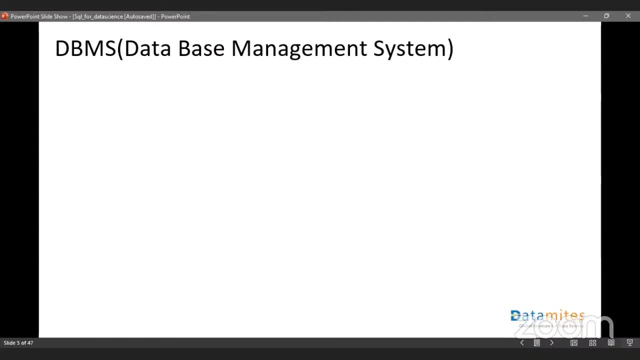 be something You call it as a software. Yes, So technically, DBMS. basically it stands for database management. It's a software which is used to manage databases. Basically, it helps you. in order to create a data, you can store data And once you store data inside a database, you have to use that. 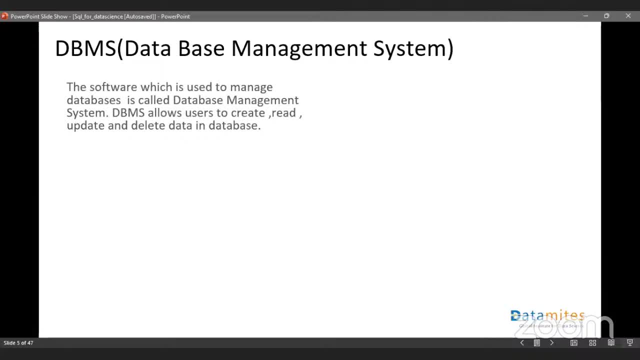 whenever you want it right. So what you can do is you can read them, you can update them and also you can delete data in database. So these operations or these modifications could be done using this DBMS. So it's a software which basically helps in storing data inside. 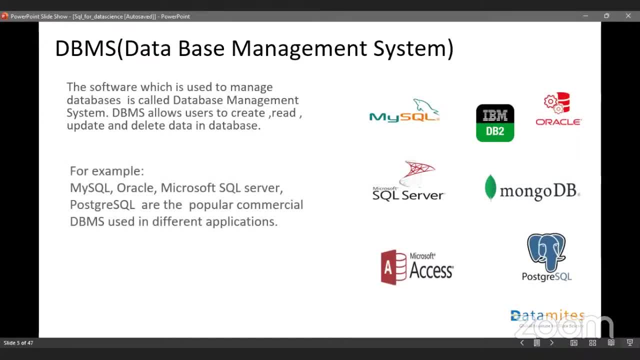 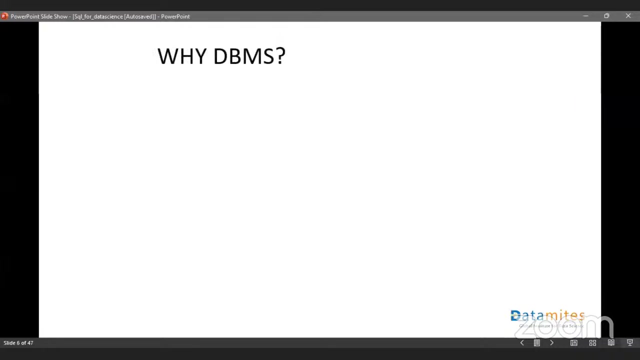 our database. Okay, So there are different DBMS softwares like MySQL, IBM DB2, Oracle SQL Server, MongoDB, Microsoft Access and PostgreSQL. So these are the popular commercial database management systems used in different applications in different companies. Okay, Okay, now the 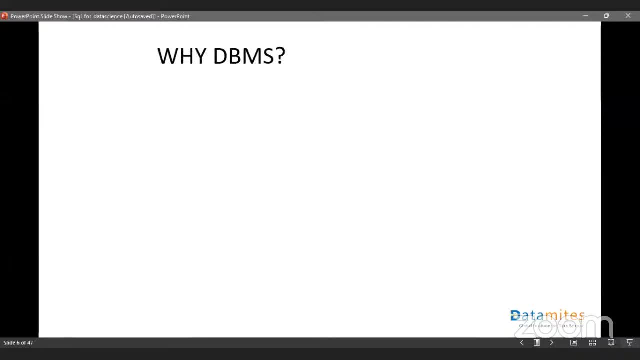 question is like: why database? Okay, we know database is like for storing data and DBMS basically helps you in linking data to a database. Okay, it's a software. Now the question is, why DBMS? So the first application is like it can store enormous data, like you know. 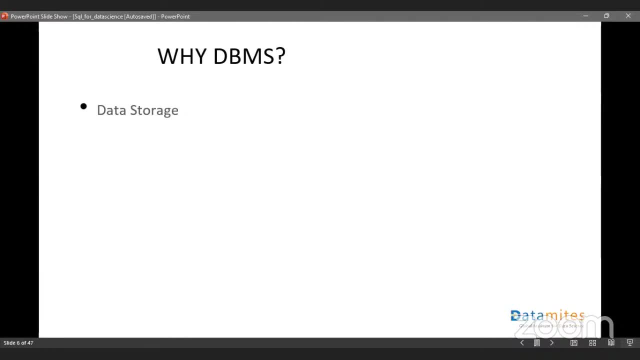 millions of data. Data storage is one of the application of DBMS. It basically helps you in storing data into our database. And the second application it's a data abstraction. So what do you mean by that? So when we have a data, so basically we will have some sensitive data, like when we collect. 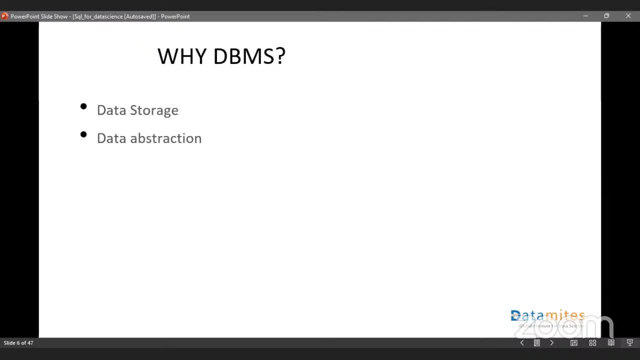 data from different organizations. let's say so we are collecting data related to a Google company. Okay, so details might be like employee details, project details. So project details are all like a sensitive data, right? So that can't be revealed to everyone. So that has. 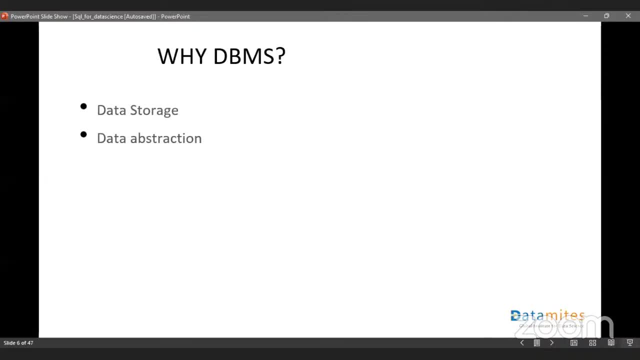 to be, you know, public, sorry, privately maintained. So there comes the concept of data abstraction. Data abstraction basically hides the complexity of the data. Okay, so that's the first one. The second one is like, how do you store data? Okay, so the first. 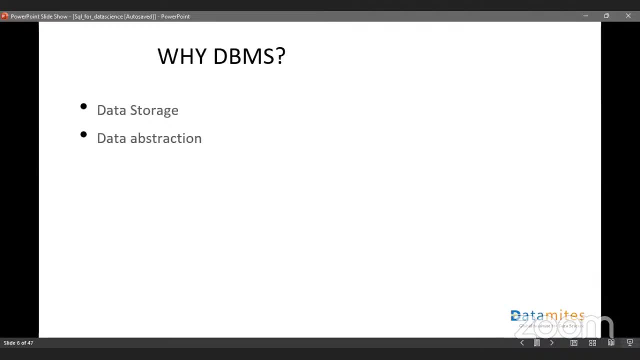 one is like: how do you store data? Okay. so the first one is like: how do you store data? Yeah, This database management system. what it does is it basically shows, like what is required for the users. it will hide all sensitive data, Okay. And the third one is basically: 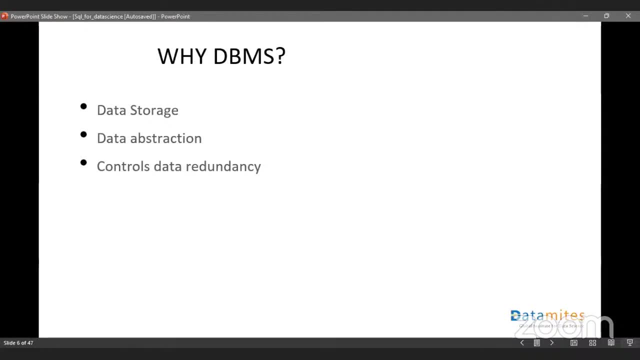 controls data redundancy. So that means when we collect the data, data can have, you know, repeated data. I mean repeated records. sometimes you might have a repeated file size will. So how do you control that? like if he, if you store repeated data, like you might you? 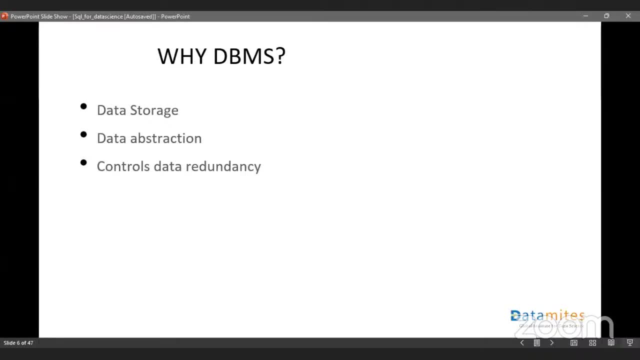 might face, you know, storage issues. in order to overcome that, what you can do is database management system basically controls that data redundancy. okay, so that it will save a storage space and also it will increase the speed of red travel and updating kind of things. okay, whatever you do with a data system, it will. 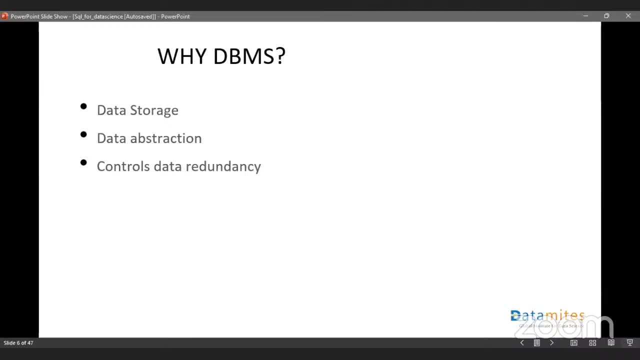 be a database. it will be very easy when you control the data redundancy, when you have a unique and distinct records, all right, and the fourth application is multi-user access and waves. okay, let's say, um, so we have a database for our company, let's say for robic's company. we have 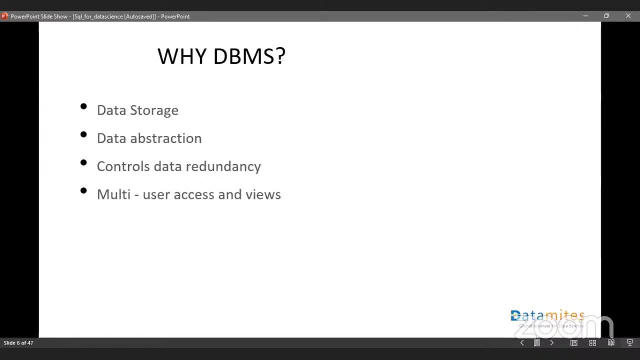 our own database. so, basically, we are using mysql and we'll be storing all our all data related to our company in our database. okay, so let's say i have my client from america. okay, let's say my client is in us and what i want to do? i want to give an access to them regarding the data that. 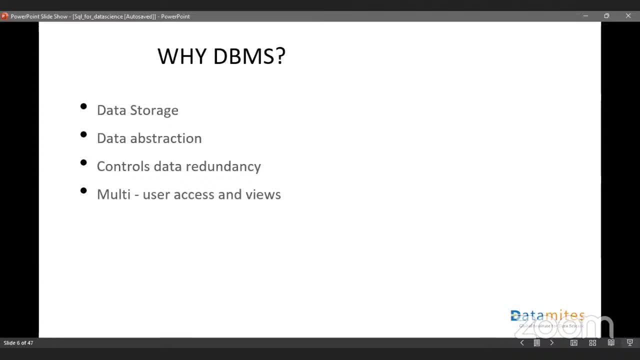 have collected. so, what you do, you need to give an access. yes, it's not that you have to give an access for only one person. you can give access, access to all the people over the world, like you know, or like you can give access to people who is in us, people who is in uk, people who is in you know germany something. 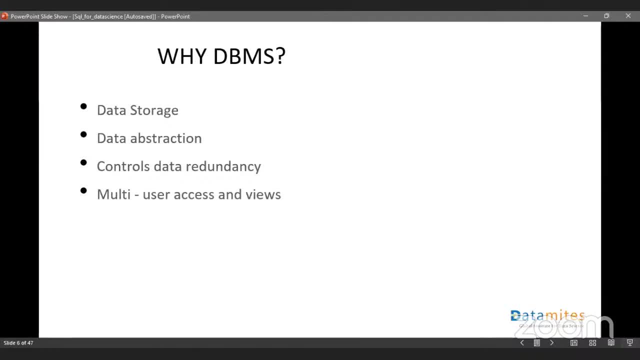 like that. multi-user access means multiple people can access, access that data and they can work on that and we've sold, so we've basically just restrict to weaving, like you can just look at, like what is happening, what has done. so these things are basically done in database management. 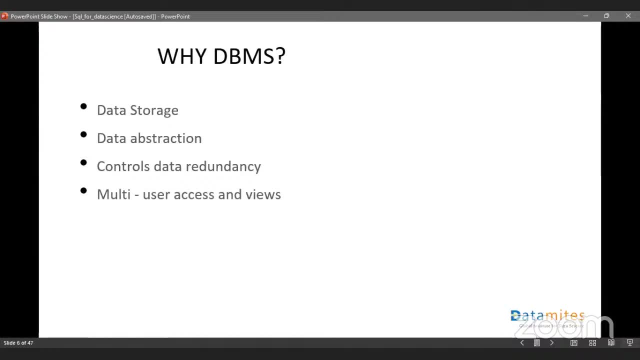 system. okay, we called it as multi-user access. even at the end of this session, i'm going to be giving you the username and password for the database of a company where you can look at the database that i've created and also you can see whatever operations or whatever sequel operations. 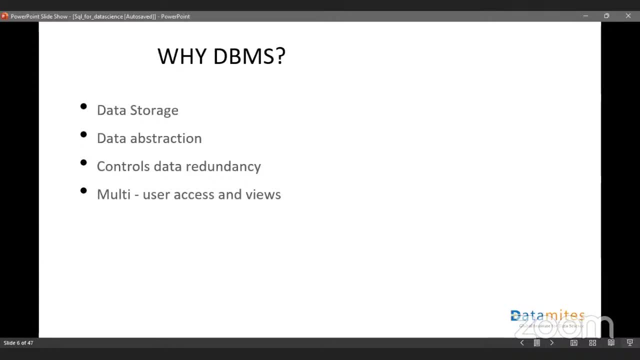 i do. you can just look at it, you can just see, like, how things are happening and you can't do any modification because we will be restricting that access just for weaving. okay, these things could be, these controlling actions could be done using database management system. okay, and you can see, here, this is a data storage thing and your people can access, like, 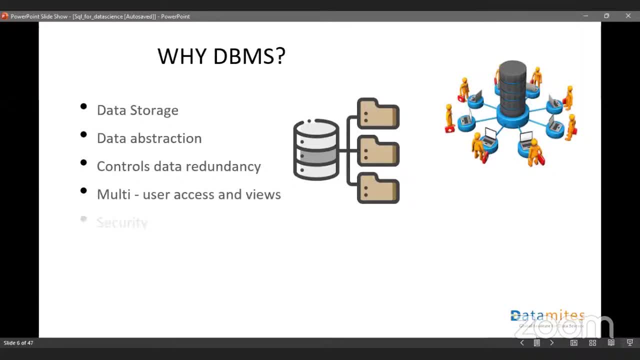 from different places, multi-user access and also multi-use user views. okay, and also the final one is security. so security plays a very important role, right, because data is very important for any business domain or business organizations. so when we give access to more people, there is a. 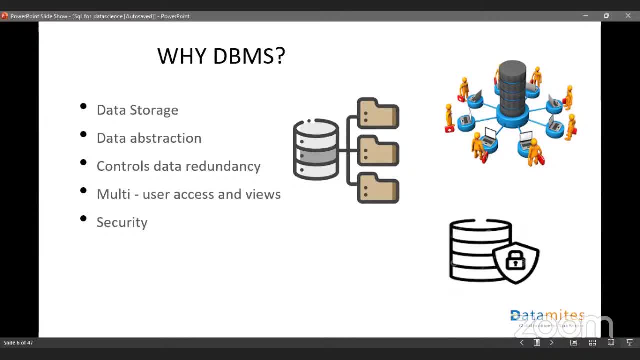 high risk of security. yes, high risk, in the sense people can store, you know um your data that might, you know that might indulge in a loss for a company, so which will be very huge loss. so you have to focus on the security when you give access to multiple users. so that is basically done with. 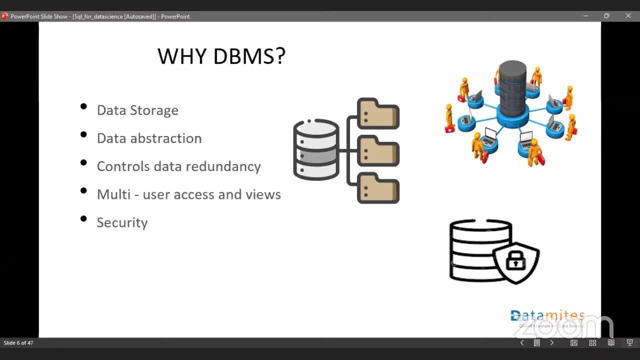 this dbms. okay, so these are the different advantages, these are the different applications of dbms. if you store your data in spreadsheet, anybody can access your- uh, you know spreadsheet, somebody can you know what- hack your system. they can take all your. you know important data sets, important content. 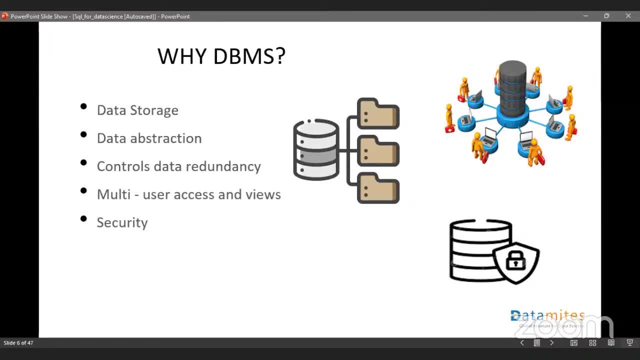 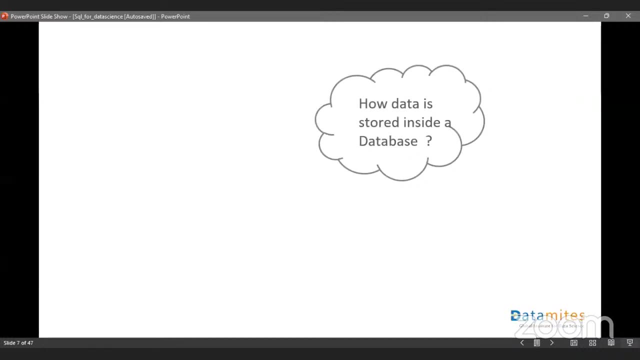 information so that can be predicted using this dbms. that's why database database management systems are evolved. yeah, okay, so we'll learn. like. what is database? it's basically you're storing data and dbms, basically it's a software which helps in storing data inside our database. 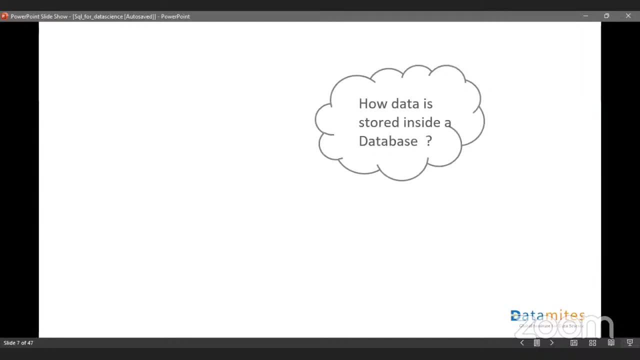 now the question is how data is stored in inside a database. how do you store that data? data can be anything right like. data can be image, data can be text, it can be a structured one, it can be unstructured one. so how do you store all those data? any idea? 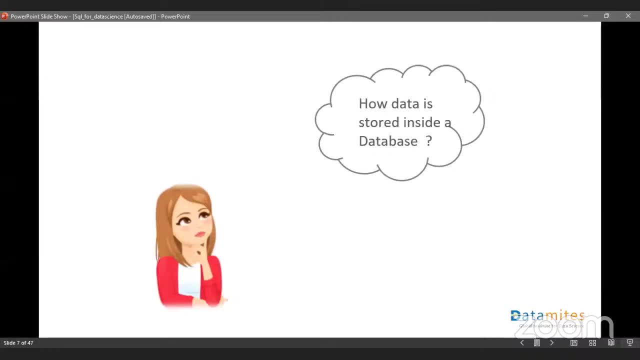 so in order to store data inside our database, like it basically tells you like how data is stored, how different tables are related, how different tables are linked. so all these things basically done with data models. so we have a concept of data models. so these data models define how the logical structure of databases model it. 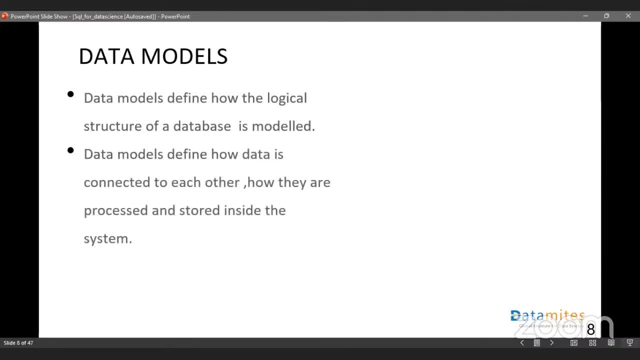 basically tells you, like how data is connected to each other and how they are processed and also how they are stored inside the system. so these things by data models, okay. so data models basically defines, like how data is connected to each other and how they are processed and also how data is stored inside our system. so there are basically different data models. 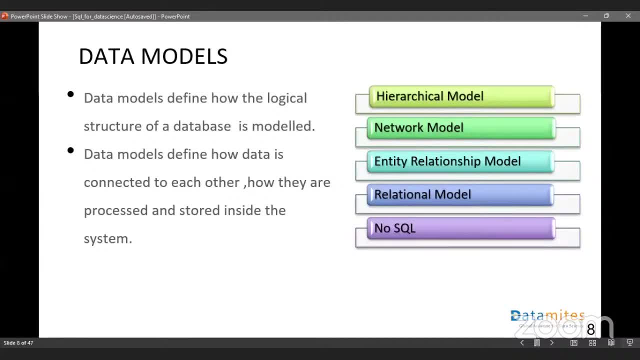 like hierarchical model, network model, entity relationship model, relational model and no sql model. so these are the different data models and there are few more, but we are basically focused on these five in that, mainly our focus- being a data scientist, being a data science engineering engineer, being a machine learning engineer- we have to focus more on relational models. okay. 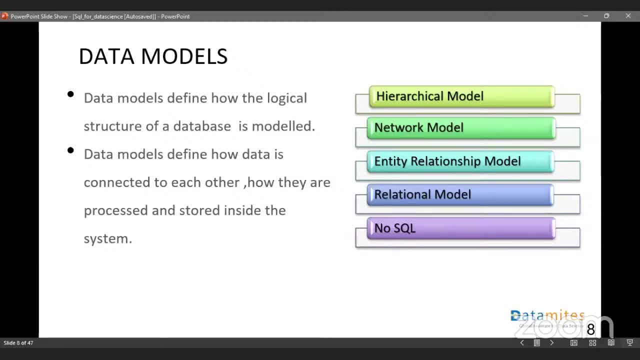 so any idea like about these models. the first model is like hierarchical model. so this hierarchical model, basically what it does, is it basically organized data in a tree form, in a tree structure form. it just creates, you know, like a node. uh, it will create a root and then it. 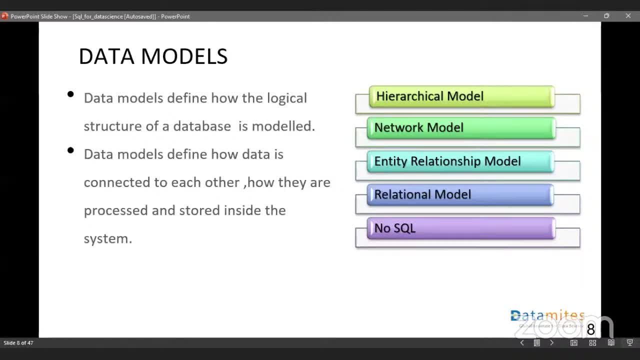 will create a node. it can be a parent, it can be a child, something like that. so tree like structure, data can be stored inside a hierarchical model, okay. and then we have a network model and we have entity relationship model. so basically, uh, in entity relationship model there will be entities and also you can connect that with attributes. 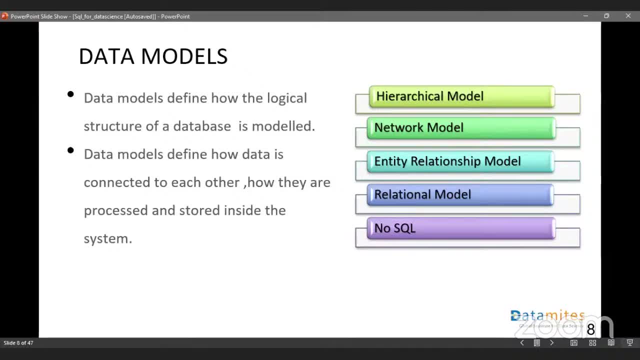 so entities are basically? it could be a person, it could be a location or even an idea. let's say, for example, if i take a school management system, it will have an entity, such as teachers, students, courses, buildings, departments. yes, and attribute means it's a property that exists in an entity for. 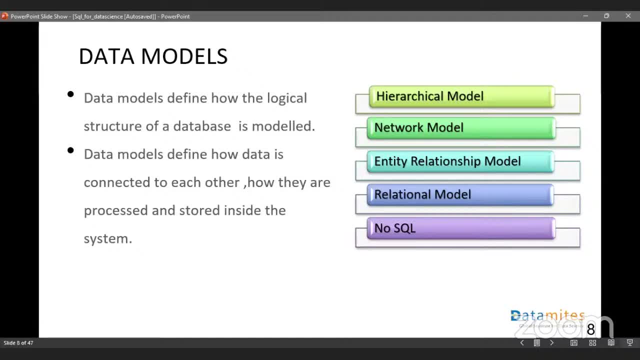 example, if i take, um, you know entity- as a teacher, what will be the property of a teacher? properties will be like, uh, like a salary, like probably our age, our id number and our qualification, whether she has done masters or she has done just a graduation, something like that. so these are the 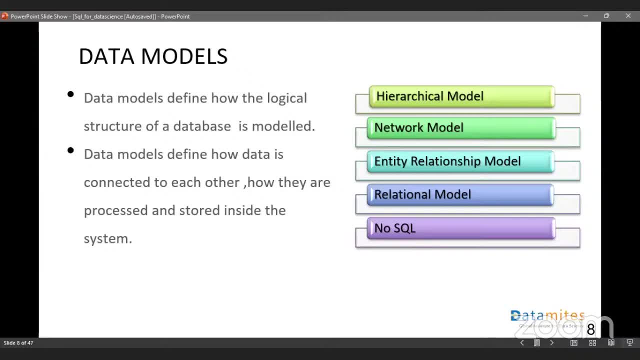 attributes that are basically the attributes of the entity. so that is basically attributes. so relationship is like relationship between two traits. that means, for example, a teacher, teacher works for a department. or or i'd say, if i say professor, professor basically works for a certain department. that basically represents our relationship, okay, professor. and let's say 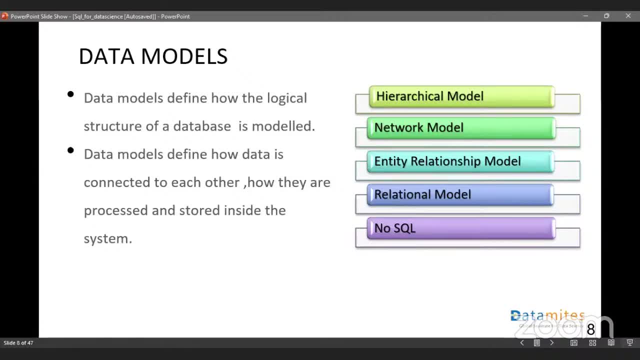 maths department or, let's say, professor in a computer department, so that particular professor has to work for the computer science department. so that is our relationship, yes, so all the things that are related to our relationship. so entity relationship, basically it's an it, it relates entities, objects and the relationship. 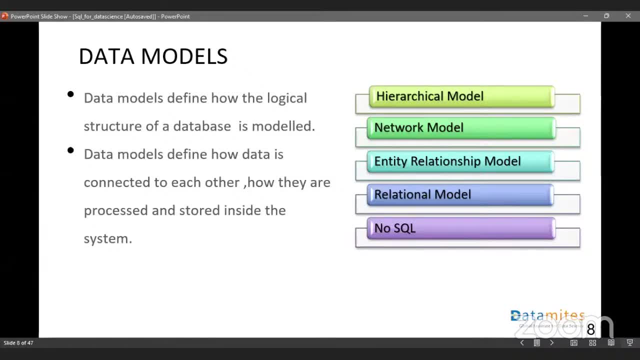 okay. and the final one is a relational model and there is also no sql. so first i'll speak about a no sql model. no sql model is like it's basically used for unstructured data. let's take an example. yeah, i'll come back to that no sql after i finish relational model, so that you'll understand it in a 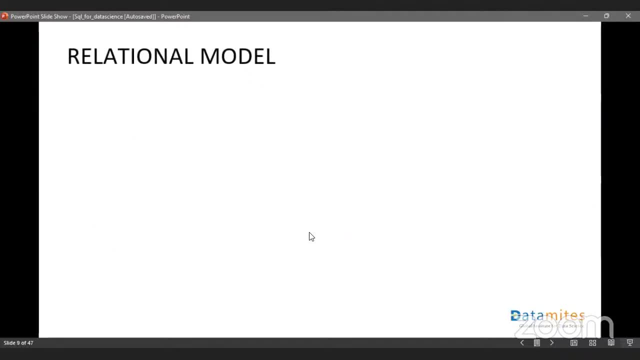 better way. okay, data models, all right. yeah, so our main focus is basically our relational model, and most of the companies, most of the companies who are doing projects based on- uh, you know, data science or machine learning, they are using relational model. i'll tell you why. so the 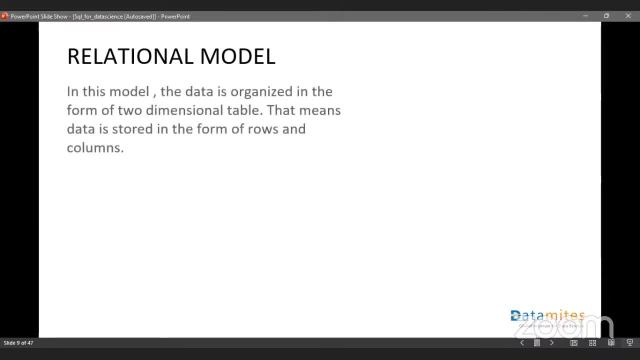 first question is: what is relational model? you know, in this model, data is basically organized in the form of two-dimensional tables. so what do you mean by two-dimensional table? people, in the sense, what comes to your mind? so you just virtualize. when i say table, so you should remember that, you should imagine that a table will have rows and columns. 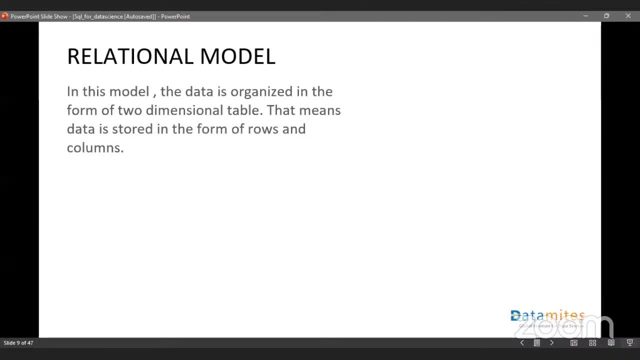 yes, so that means when i say it's a relational model, data will be stored in the form of rows and columns, and you remember, if you have done course on a data science, so you might have done few projects where you have used csv format files, like where you had a data frame. do you remember? 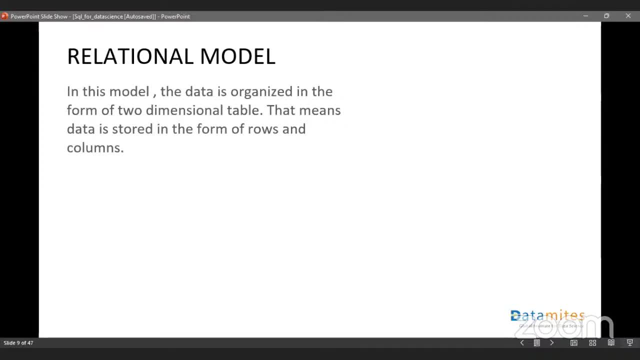 so we use the pandas libraries in order to handle that data frames. data frames are basically a two dimensional table which has rows and columns. so since we deal with our a data frame kind of- i mean, uh, in order to do any machine learning or data science projects, 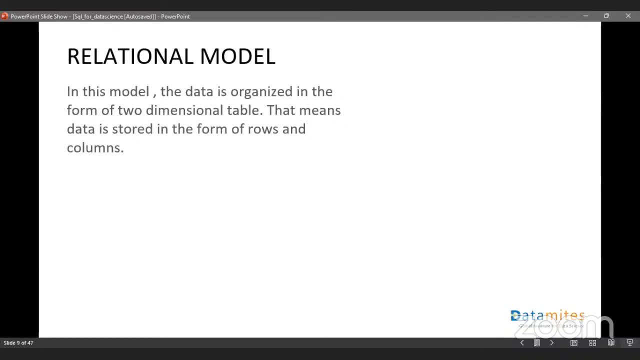 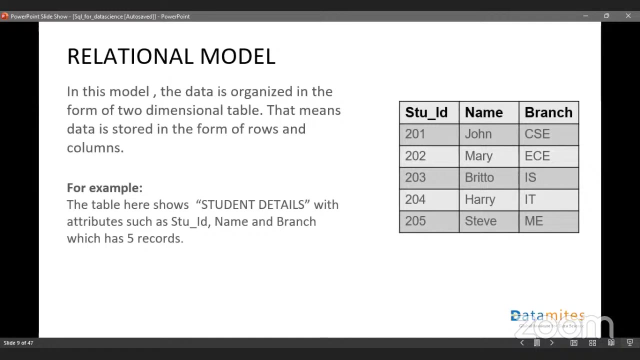 what we do, we use data frames. that means our tables. so that's the reason why we are using relational model. even relational model basically stores data in the form of rows and columns. for example, you can see here i have taken a table which basically gives you an information related to a student. 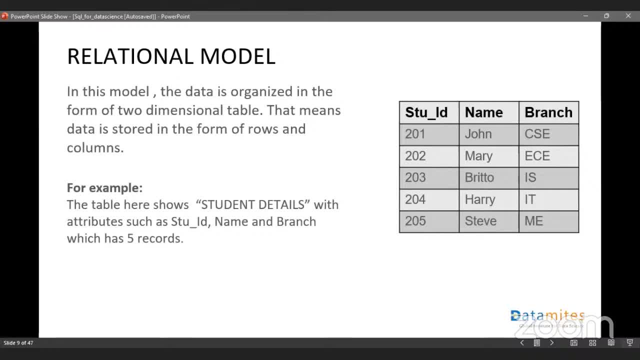 Okay, it's a table or it's a record or it's a data related to a student of an engineering college. So basically, engineering means there will be a different branches and students means there will be different students And also there will be a unique ID for students. Here you can see student ID name and a branch. 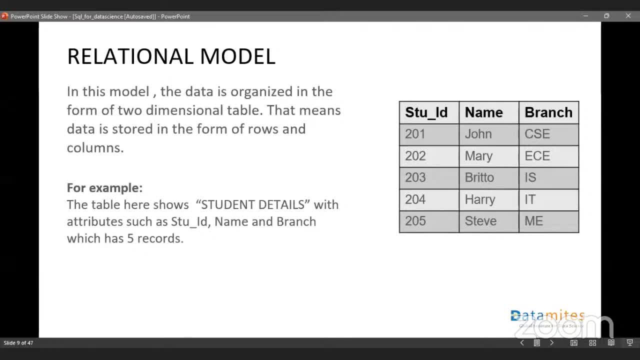 Okay, so basically what is that? You can see rows and you can see columns. Columns are basically student ID name branch. So basically columns are basically called, as you know, attributes, And whatever rows you have- like 201, John CSE- they're all like a record. 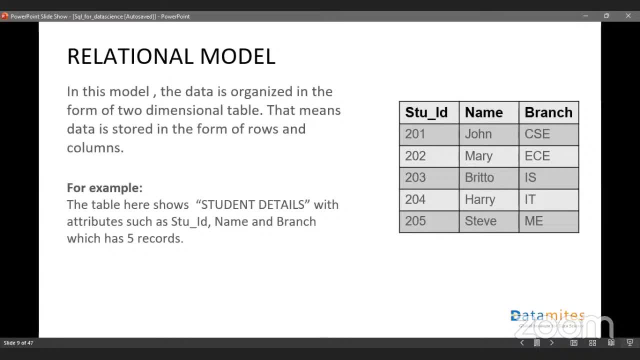 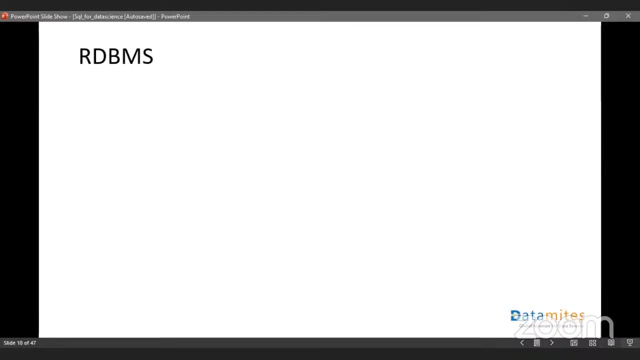 Rows are basically a record and columns are basically attributes. Okay, remember, relational model means data will be stored in the form of rows and columns, Pure Okay. okay, So we got that idea Like how- Okay, let me come back to this. So this is a relational model. 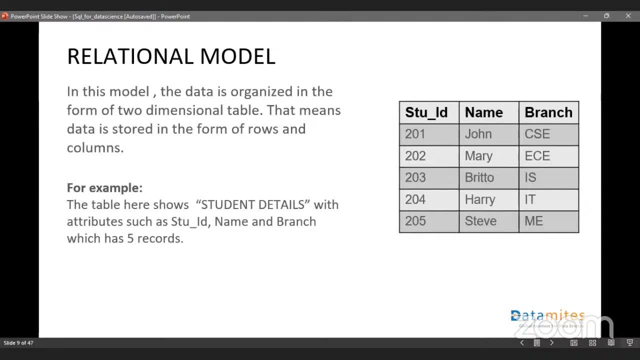 And there was one more model, right like NoSQL model. So NoSQL model is basically, you know, it's used for unstructured data or in order to create a key value pair. I just want to say the difference between a relational model and a NoSQL model. Let's take an example. 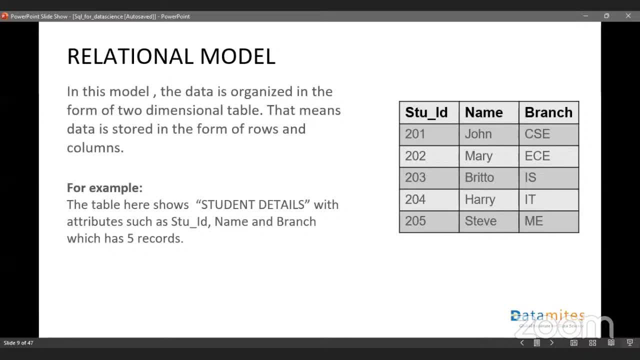 Let's take an example of you know a Flipkart sales data. So let's say so: when Bali comes, sales will be very high, like what we people do. we, being our customers, we purchase many things. So because there will be many offers, we go within offers and we try to purchase things. 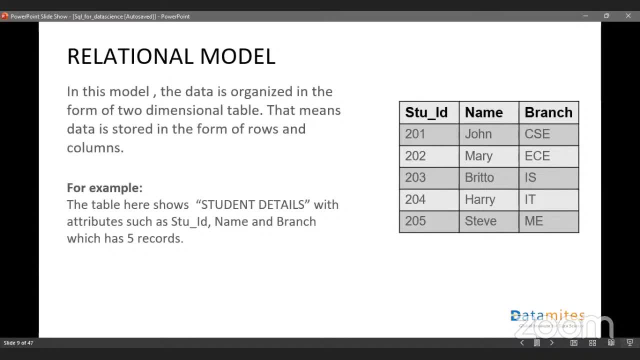 So what, what we do. let's say I'm Jeevita, So I just want to purchase few things. I want to purchase laptop, I want to purchase mobile and also I want to purchase some- you know- clothes as well. 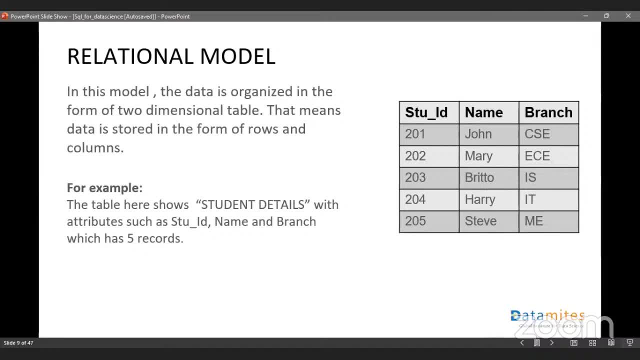 So what I do? so today's my first day. okay, I'll purchase laptop in the morning. Okay, so when I purchase laptop in the morning, my data will be stored inside our database. So when I purchase laptop in the morning, my data will be stored inside our database. 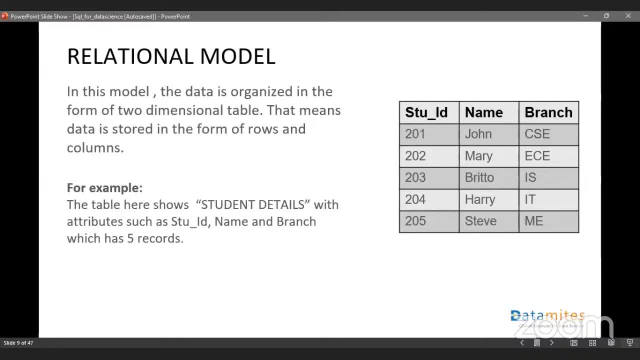 So when I purchase laptop in the morning, my data will be stored inside our database. so, basically, what companies do they collect the information, right? so when i want to purchase this laptop or a mobile, what i do i'll just log it by giving my details. yes, i'll give my details, like. 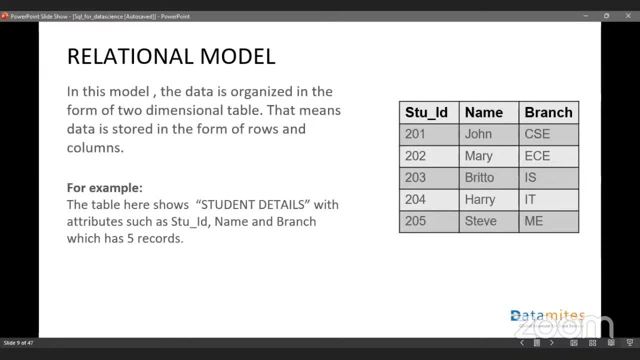 name, my phone number and also i'll give address, yes and also. so basically what i'm purchasing in the morning i'm purchasing laptop, okay, after that what i do. so i'll be just looking at the what flipkart app and i'll see, you know there will be an offer for laptop. so again what i do. 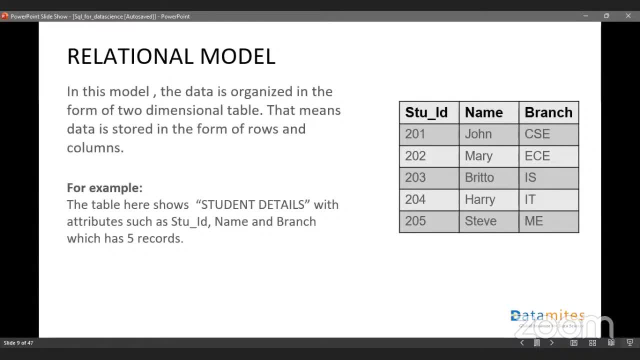 so if i have enough money. so because of that offer, what i do, i plan to purchase that laptop in the afternoon. so initially my record will be stored in the first row. yes, so in the first row. when i do the shopping in the morning that record will be stored in the first row again, if i do. 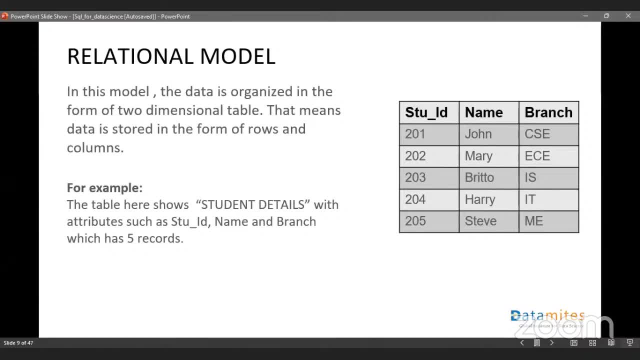 shopping in the afternoon, like i'm basically purchasing laptop. so again, it will store the details of mine in the second room and also, if i do, if i again purchase it in the night. okay, let's see, probably in the night i'll look for some. okay, i'll look for some accessories, like i like that and even if price. 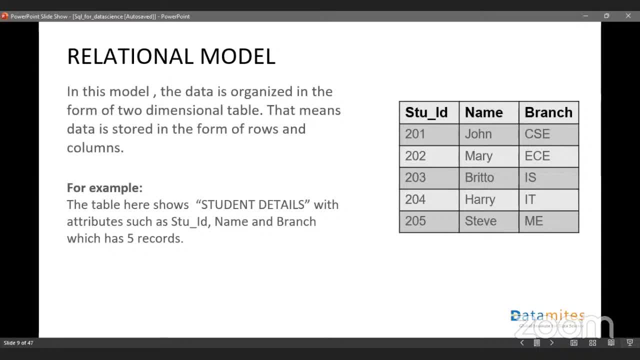 is reasonable, i'll go for shopping. so basically what i have done: i have purchased three items in a single day. so that means what relational model will do? it will store data for every attempt. i mean for every purchase when i do, when i, when i purchase new items in a flipkart. 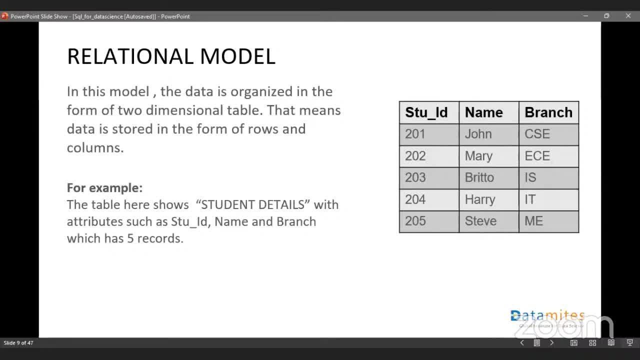 it will store records in every room. okay, so that means it has created three records. imagine, if i do a flipkart and i have purchased three items in a single day. okay, so that means, like, if the same thing is done by different people, like there are millions of people who 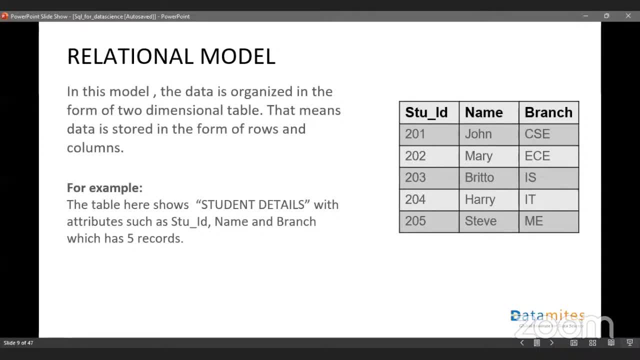 are looking into a flipkart and who is doing online purchasing. so what happens here? data is increasing like. like there are three rows for individual people. like if it's for five people, it will be like five threes are 15. like there are duplicates, right. like we are taking the same details, like 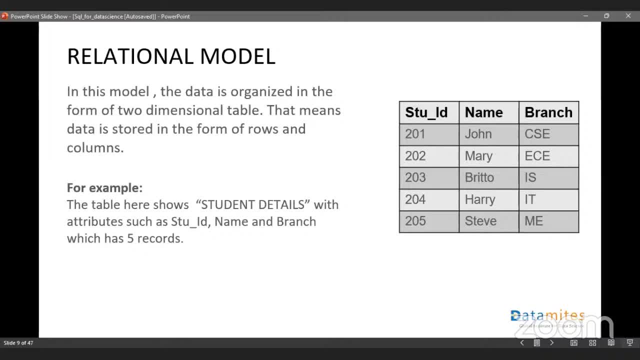 name same thing, phone number same thing. address: same thing. only that changes product name. yes, so this is how data is stored in our relational model, don't you think that's right? so that means records are repeated. so instead of this, they have developed a concept of no sql, but where what you 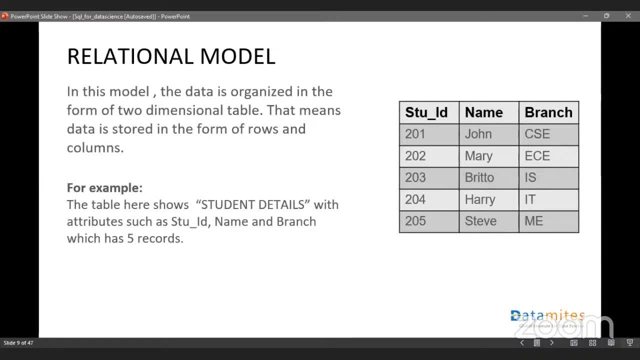 can do is, instead of printing three records, instead of recording- you know that purchase details every time- what it does, it will just create one record for you. it will create one record in your name, so one record will be created in the name of g visa. so what, what it does is so. 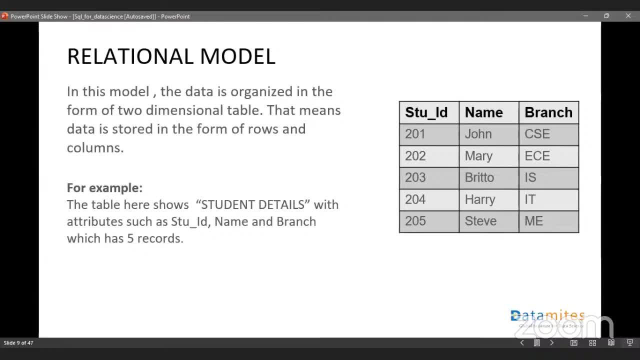 if i purchase in the morning, whatever product i purchase, that will be entered in the second column. if i do shopping again in the afternoon, that will be entered in the second column, okay. and then if i do shopping in the night, same whatever product i purchase, that will be mentioned in the third. 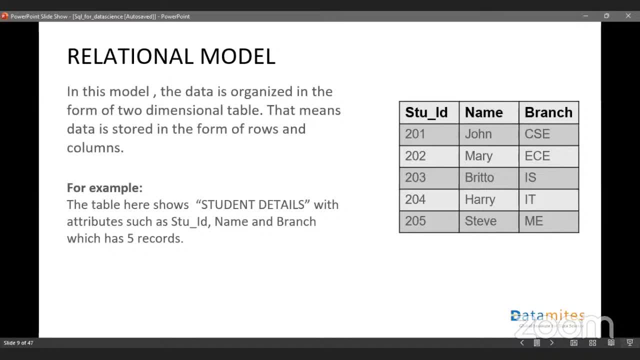 column. so what is happening? i'm reducing number of rows and i'm increasing a column. so we call this as a key value pair. do you remember a dictionary? so what we do in dictionary dictionary, do you remember like it's a python data structure where you store 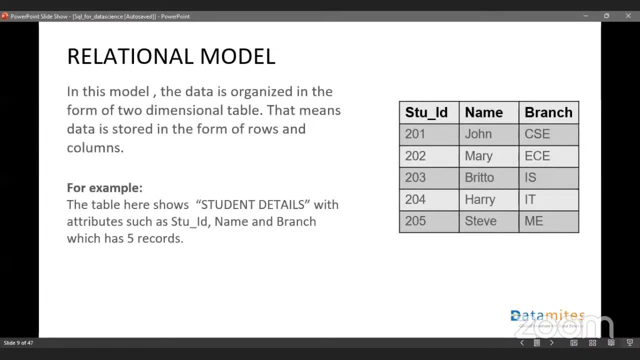 i mean where you store data in the form of key and value. keys and values: here the key is jivita and, sorry, here the key- yeah, key is jivita- and values will be like your product names. so basically, instead of printing my details on three rows- what no sql database will do- it will just print in a single row. 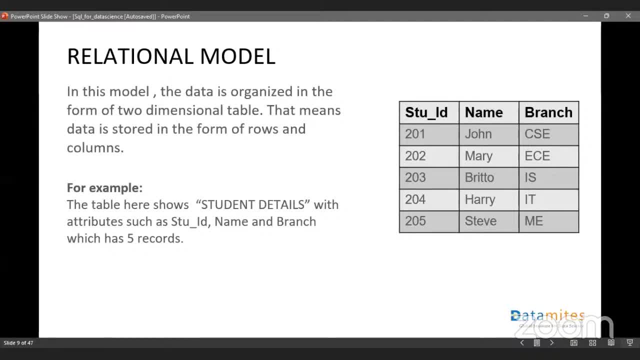 okay. so that's how no sql database works and uh, this no sql database basically uh introduced. it's a model. no sql model uh introduced in the year 2000 and this relational model basically introduced in 1970 itself. so it's an advancement and it basically, you know, one of the advantages. 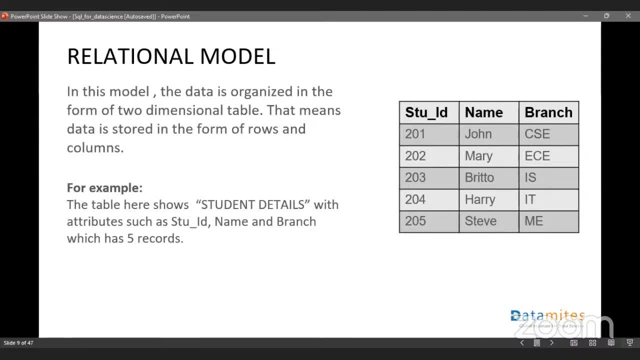 like, uh, we can save storage space and also it will be easy for us to extract the records, and i know too, um, it doesn't follow any structured one like key value pair. and also one more thing: is like most of the companies, like top companies, such as facebook, instagram, uh, google- that using this, 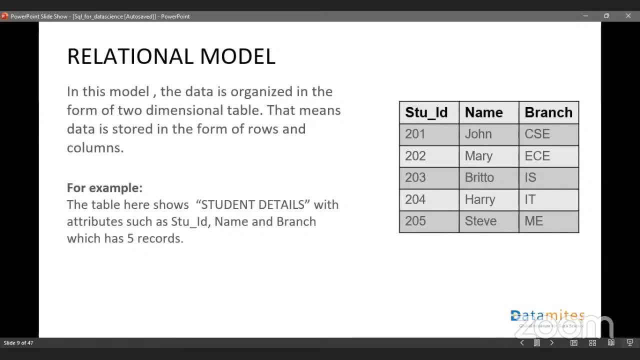 no sql database, even linkedin, because, like, every time when we log into our facebook or when we log into our linkedin, it creates, it generates our data. yes, do you know, like why facebook, instagram, whatsapp they're making so much money? it's because of you. you people are using it, like. 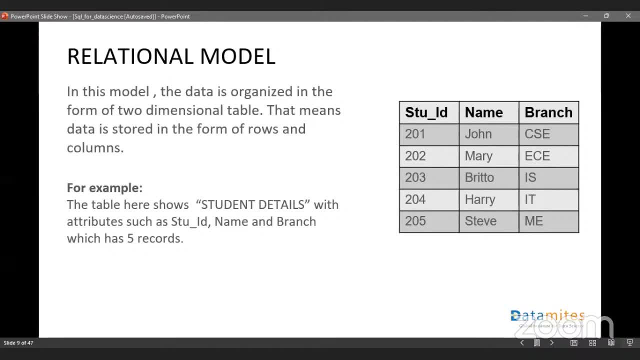 all the 24 hours you'll be in front of your mobile and you'll be in social media. i don't know, like, whether you are grabbing something that from that or not, but you're profiting for the companies like google and- sorry- facebook, and for linkedin. yeah, linkedin is a best platform where you're learning. 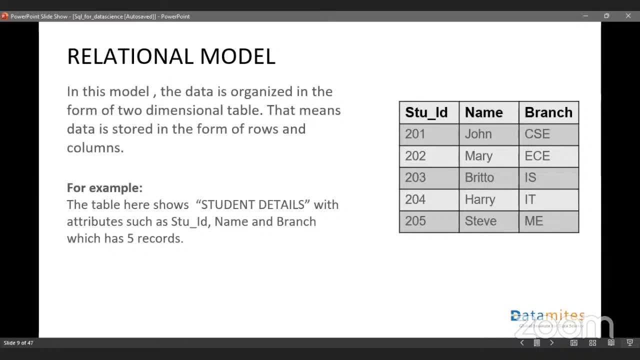 but just think about your instagram, facebook and also whatsapp. like it made you to communicate with the people, but still, like you're communicating and the company is making. like you know, like can't even imagine about the profit that people are making, uh, in these companies. okay, so this is. 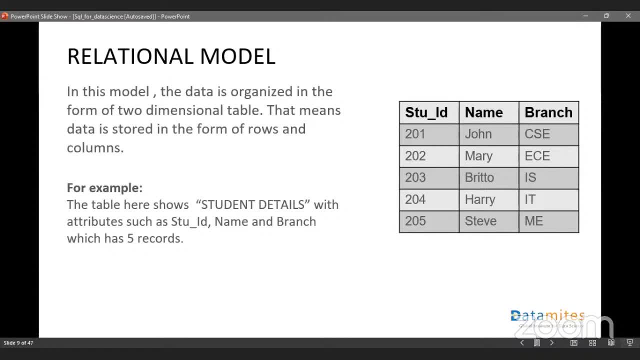 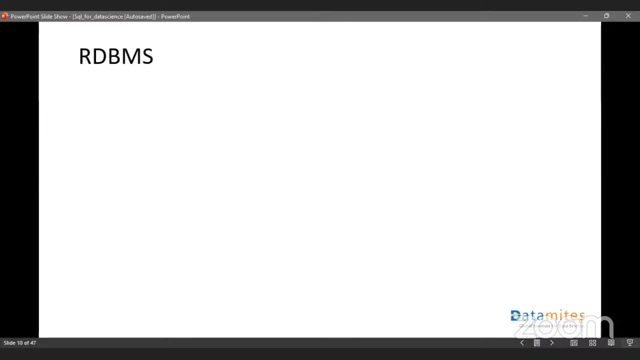 the difference between relational model and no sql model. is it clear? yeah, so we learned. like you know, a relational model means data will be stored in the form of a table, that is, rows and columns, and so, in order to store that data in a form of rows and columns, 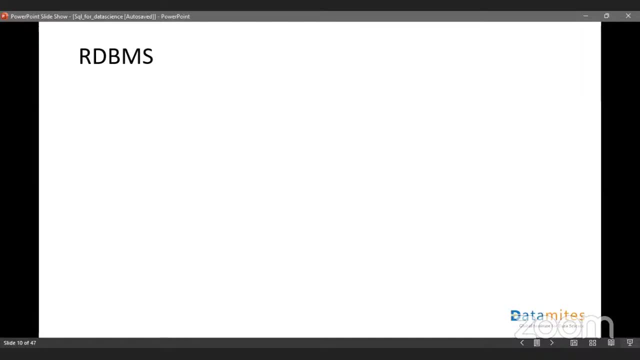 we need some software, right. the way we got dbms in order to store data in our database, so we need one more software in order to store data in a form of table, that is, rows and columns. so we call that software, as you know, rdbms, so we can see the program or a software which is 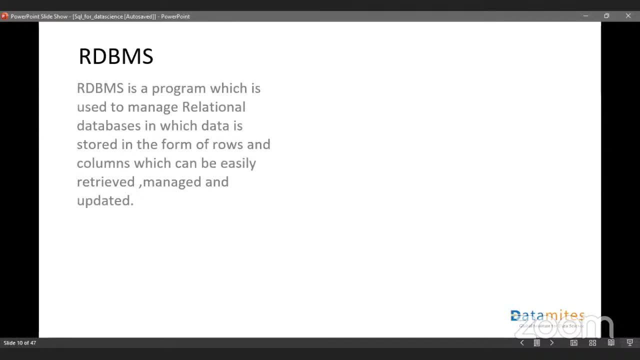 basically used to manage relational databases in which data is stored in the form of rows and columns, which can be easily retrieved, managed and updated. see, uh, when we store data in a form of a column. sorry, when we I'm sorry, yeah, so when we stored our data in the form 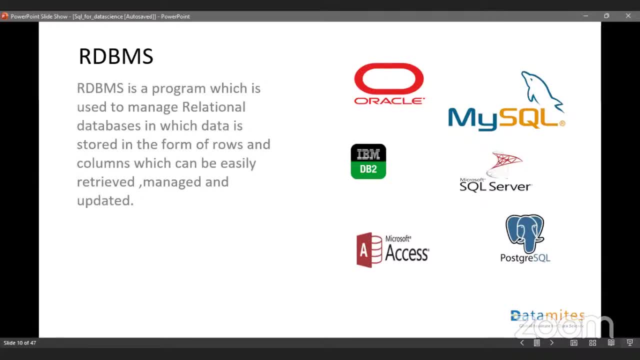 of rows and columns. it's very easy for us to extract. do you remember accessing? you might have studied, and that's in slicing. when you study python, what is the purpose of doing indexing and slicing? we started from strings. we took a string and we started extracting characters and then we moved on to the data structures, like let's double set there. we. 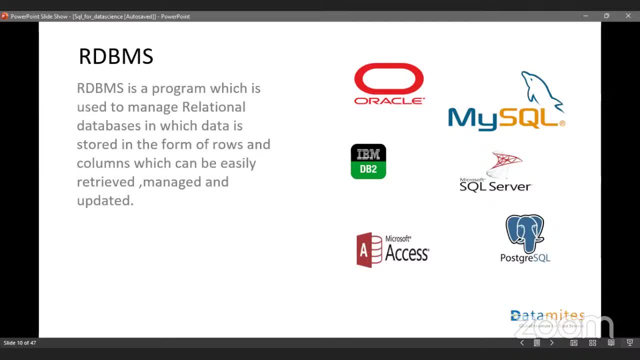 started extracting elements. then we moved on to the numpy array: array, basically stores and elements. so there also, we started extracting values. yes, no, extracting elements, extracting range of characters or range of elements, and then we came to a pandas. then what we did? we extracted rows, we extracted. 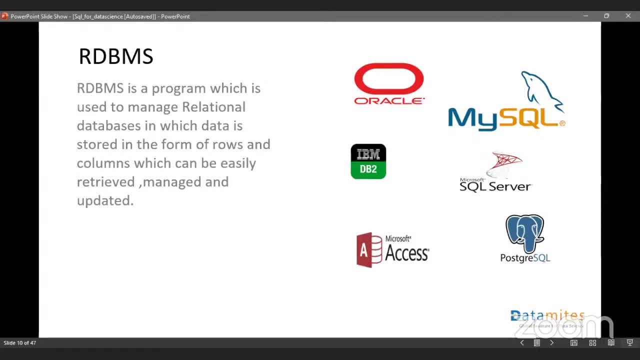 columns. yes, so it was easier for us because of this structured format, because of this relational model, because data was stored in the form of a table. if it was not in the form of a table, it would have been really hard for us to extract the data. right, but it would. it would have been really 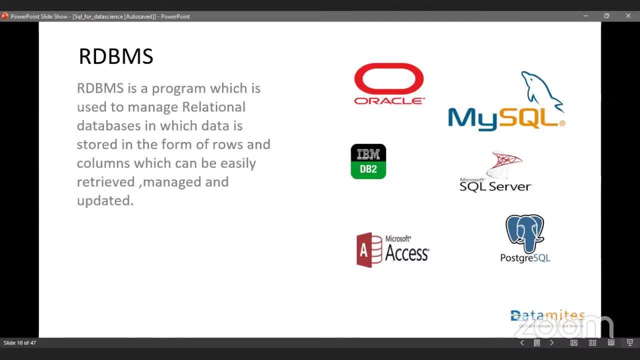 hard for you to apply slicing or indexing part. okay, so that's why rdbms is a program which basically manages a relational database and which data will be stored in the form of rows and tables. this software, or this program, basically helps you in retrieving, you can extract the data. so 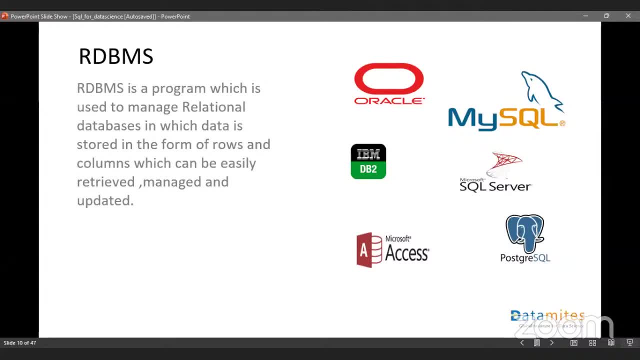 whenever it's required to you, you can manage, you can extract the data. so whenever it's required to you, you can manage. and whenever, if you want to make any update or like if you want to make any modifications, even that could be done using this rdbms. okay, so you know about the different databases, like 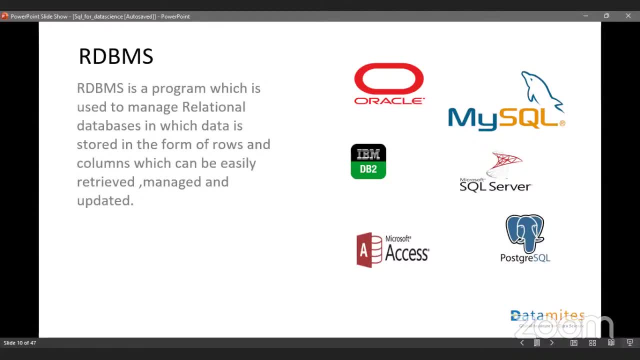 they are mysql, oracle, uh, microsoft taxes, ibm, sql server, postgre sql, and i have mentioned mongodb, mongodb and also, uh, cassandra. i forgot to mention that. they are also our databases, but can you see the list of databases here? because these databases are, as you know, rdbms databases. that means these databases basically use release, my model that. 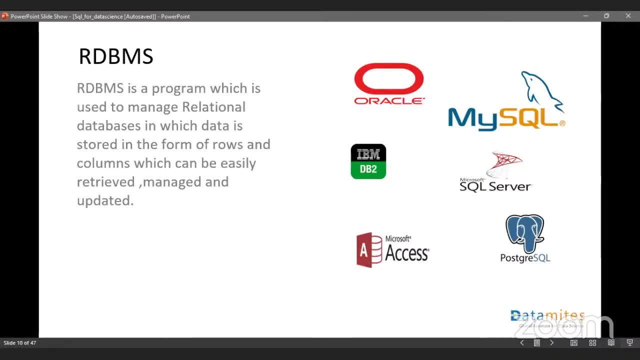 means they basically store data in the form of rows and columns. oracle- these are the like top databases of which companies are using nowadays, so one is oracle and either one is mysql, ibm database 2 and also mysql. microsoft sql server, and there is also microsoft access and there is postgre sql. 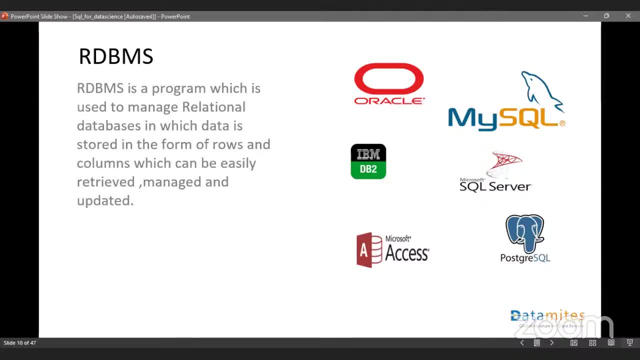 so these are the different uh databases that are used in the form of rows and columns. so these are databases which basically use relational models. that means data will be stored in the form of table, that is, rows and columns. here, if someone asks you a question like what are the difference? 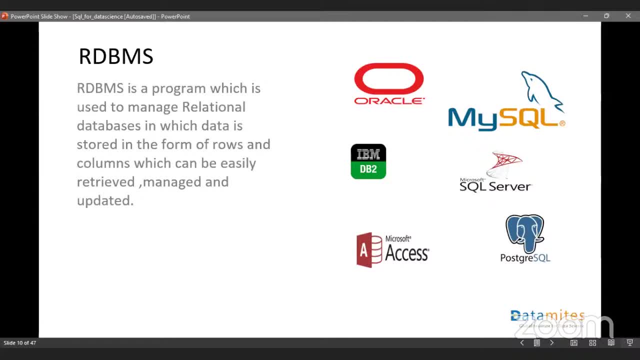 of relational models or the databases which use relational database. so you should be able to answer that it's an oracle, mysql, ibm, sql server, microsoft access and postgre sql. okay, and example for no sql is basically mongodb and also the database which we use as a release model. 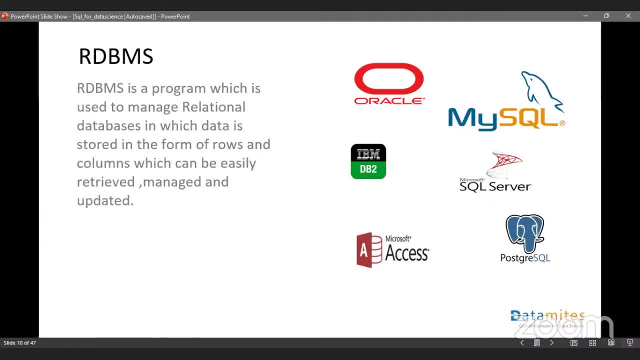 to Cassandra. So nowadays, yeah, people are using NoSQL database as well. There are MongoDB and also the Cassandra. like that. you know like a top place nowadays because most of them started using that, because you can reduce that. you know like repetition The way I gave an example of Flipkart. 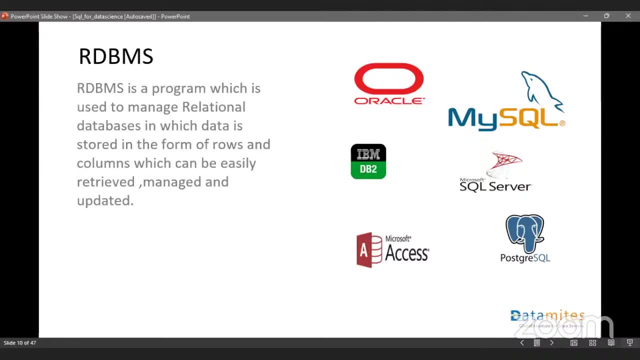 like when you do sales. it will, it will repeat the things, it will repeat your details. Instead of that, what they can do is just they can, you know, create a key value pair, And even it will be easy for accessing, easy for storing. So that's why, So, compared to relational data, 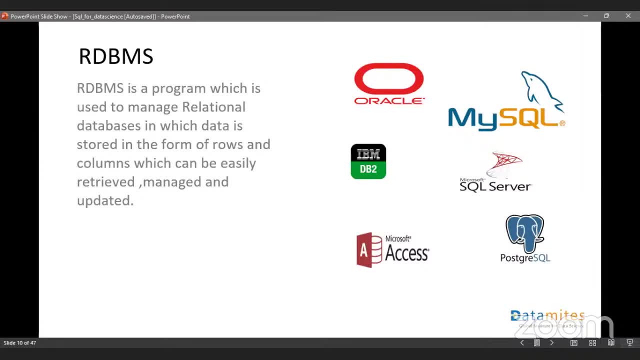 based management system, I mean relational model. NoSQL is somehow good just because of these two reasons And also a recent advantage, disadvantage in NoSQL as well, because it will not have a structured format like the way we have it in a relational model. So yeah, So basically these: 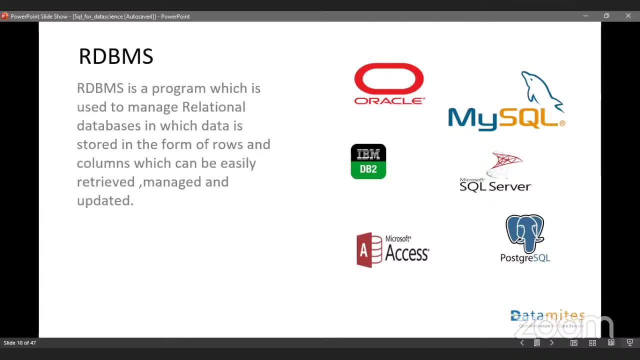 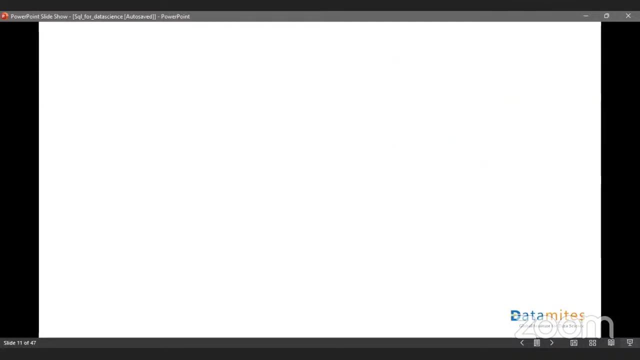 two are used in different ways: relational models in order to deal with a table table comparison. Now, most of the companies who are doing projects on data science or machine learning, they're basically using this: relational models, that is, RDBMS. Getting clear, Are you getting? 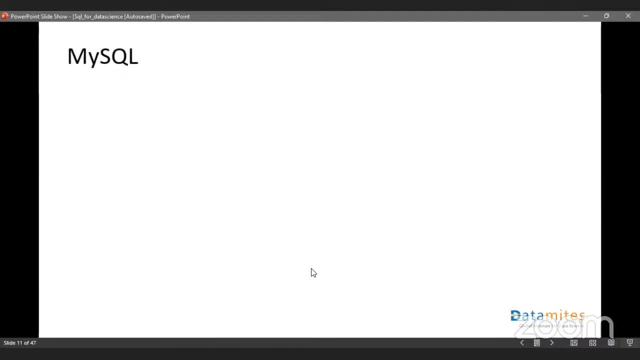 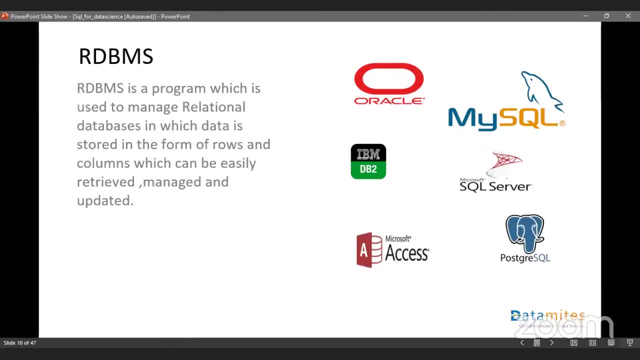 that Thanks So well. so we saw different RDBMS right Like Oracle, MySQL, And for the session and for this entire webinar, I'm basically using MySQL. So that is a reason behind, like why I'm using MySQL. 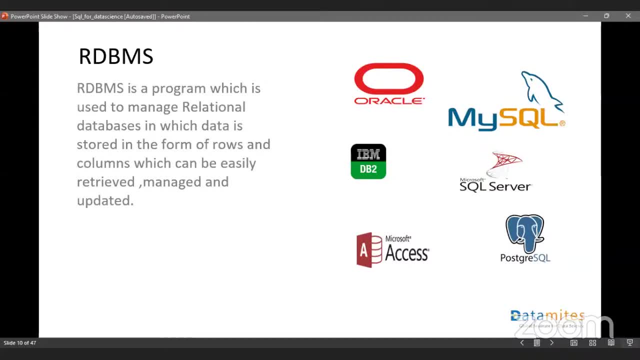 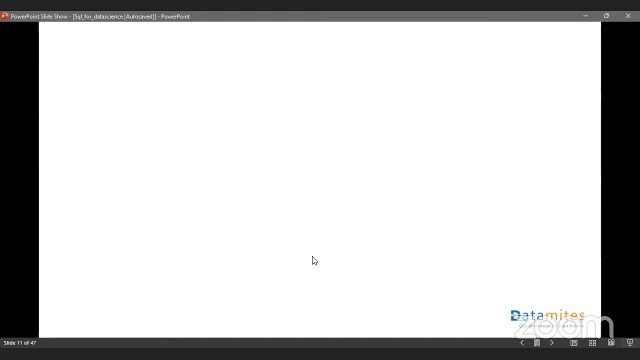 You can also use the different SQLs RDBMS that I've mentioned here, like Oracle, IBM, Microsoft Access and PostgreSQL as well, But I'm showing you like how to work with MySQL database. So yeah, Any questions regarding database RDBMS. If you have any questions, I can just tick out them. 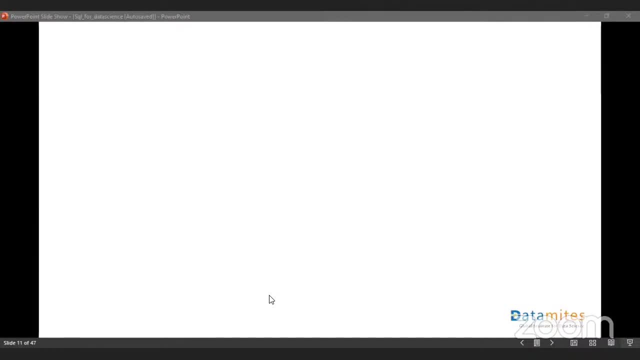 Yes, you can get the recording of the session. It's basically a live stream. It will be available in our YouTube channel. You can post your questions on Q&A. Yes, it's a Microsoft product. Yeah, difference between DBMS database: it's a database management system which is basically used. 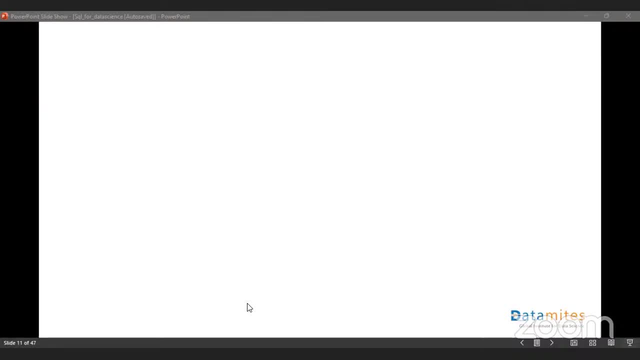 to store data inside our database. Relational database management basically used to store a data of the four tables, a data which follows our relational model format. Relational model means it has to be. a relational model means that data should be in form of table and it should have rows and columns. only then you can store it. That's the difference between our database management system and relational database management system. DBMS doesn't. 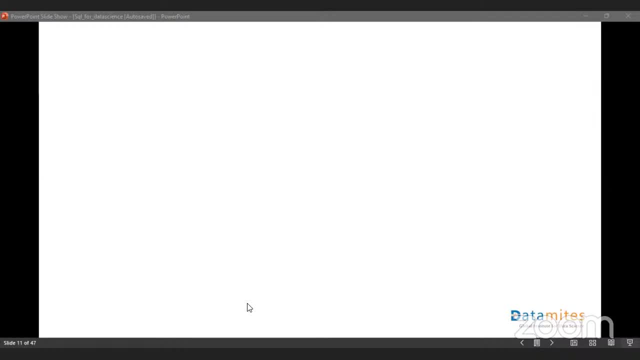 use any of the model, So it's a starting thing. Okay, like it will store data, It will store any data into our database. It's a general thing. RDBMS means it will store a particular data. That means if data follows our relational model, only then that will be stored. Yeah, Any other questions? Let me look at Q&A. No questions? 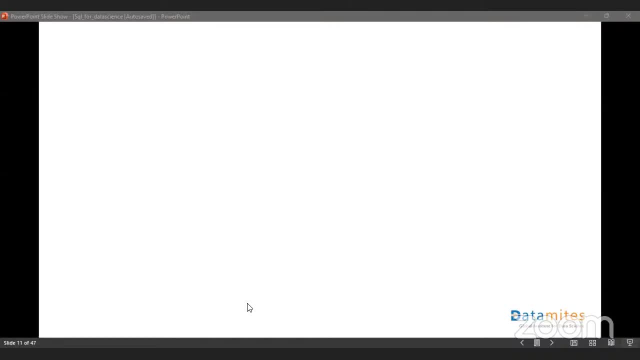 Yeah, Any other questions? Let me look at Q&A. No questions. Let me look at Q&A. Even network model- even it's like in hierarchy model- basically represents objects and entities and also represents in relationship between them. So what DBMS will be used mostly? mostly in data science projects in real time basis. basically we use relational database only. 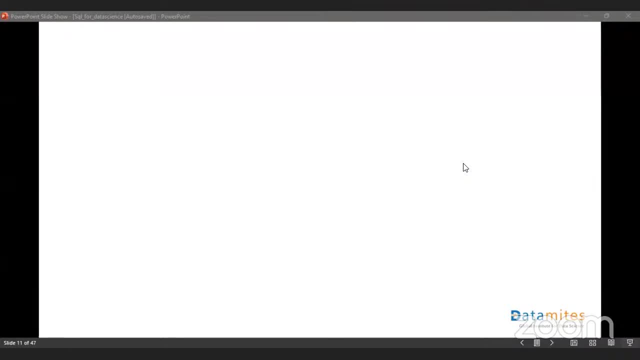 Most of them are using relational models And DBMS. you can use MySQL, you can use Oracle and also you can use Microsoft Access or Microsoft Azure. Do you want to know the advantages and disadvantages of SQL and NoSQL? Not really. 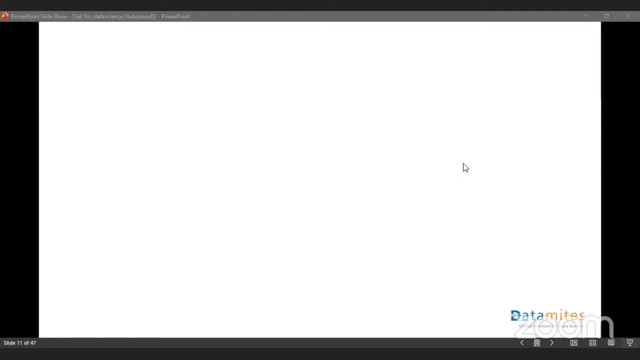 We are not using NoSQL. Probably in the future We might use, But right now we are using just I mean relational models. See differences in our data, In our reality, In our relational model, you basically store data in a table format: rows and columns. 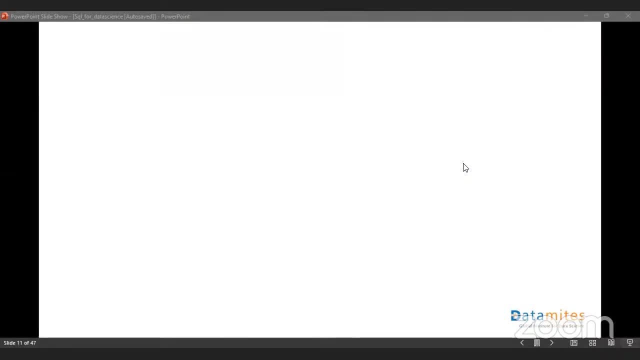 like that will be a structured one, Okay, But in NoSQL it will not be a structure. Like it will have a key-valued page And you can see the difference. like you know, a relational model, it's like a vertical. 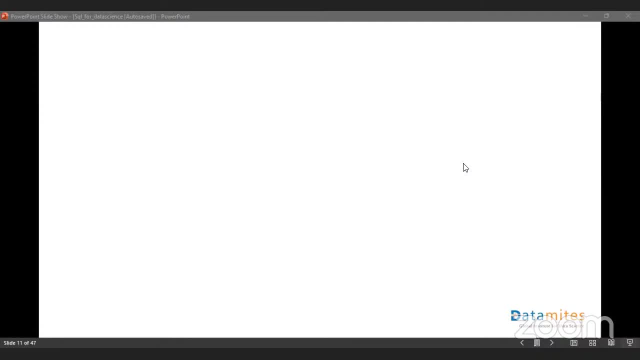 scaling. Vertical scaling means you will store your records vertically. Like you will add values, You will add records one by one. The example- That's the example that I gave- related to a flip card, like purchasing things. Just remember that to compare an example with what is relational and what is NoSQL. 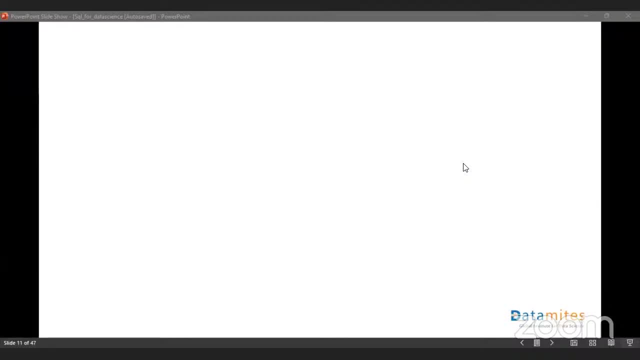 So basically what you do? you keep adding values. That is a vertical scaling. But what do you do in NoSQL? You will add horizontally: Yes, No, So it's in horizontal scaling, NoSQL is horizontal scaling and relational model: it's basically vertical scaling. 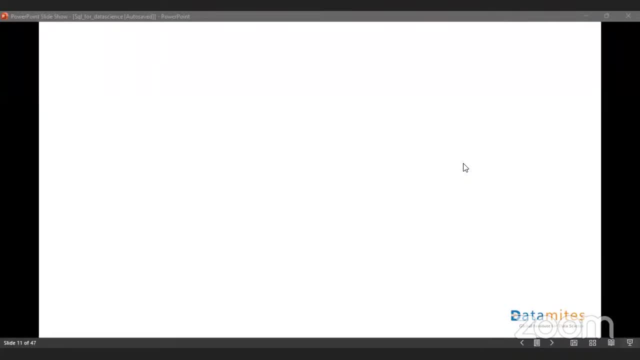 Even in NoSQL it's not always horizontal And I think you can do a lot. I think it's like it's like you know, Even there's- NoSQL can work for large amounts of data. One of the disadvantages is lack of standardization. 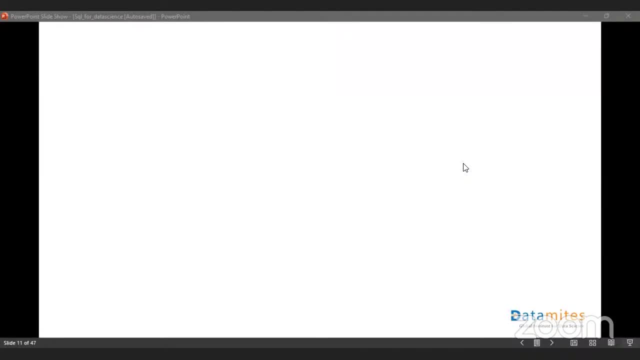 There are many NoSQL databases and there are still no standard ones. Still people are in dilemma like what's to use? Recently it has started and still it to make some standardizations And also there should be some. even in the NoSQL database people have to make some changes. 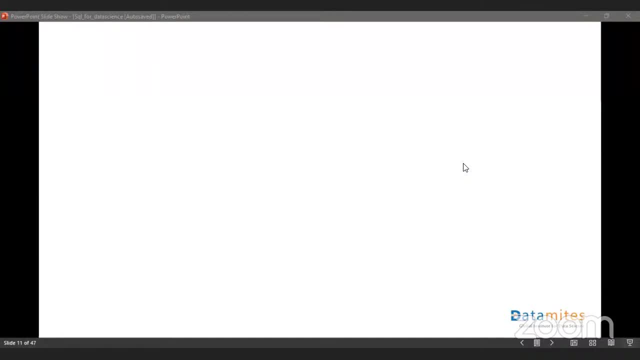 It's basically now working on few platforms, only like few operating systems. It will not run on Linux operating system, so some modifications has to be done. Even it has a poor usability. NoSQL has poor usability because it doesn't have any management. 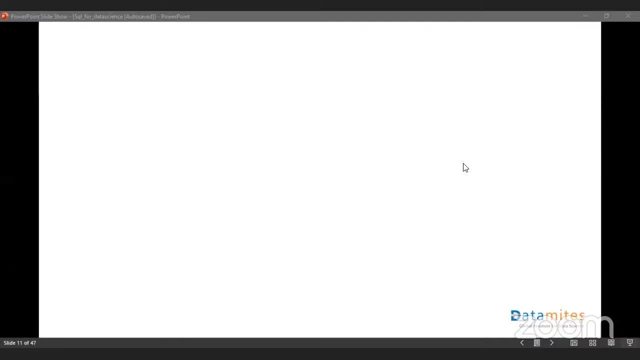 Management tools and accessing all those things. So to explore more on NoSQL: probably after 10 years we can see an improvisation or advancement towards NoSQL. Yeah, but most of the top companies are using. So let's see, DBMS is just a software which helps you in storing data, any kind of data. 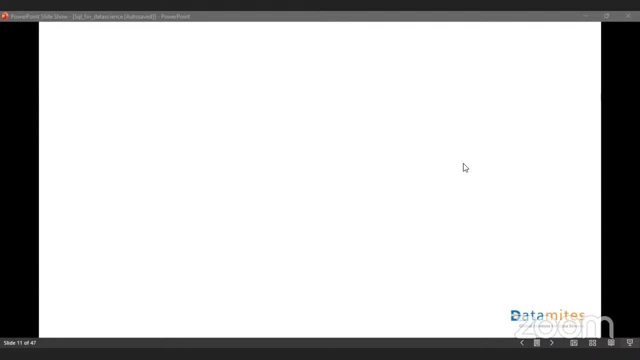 Okay, what DBMS does is it acts like a software which takes your data and it will store. Okay, it can include everything. but the question is like how your data set is stored, like in what format? for that, we have our data models. we have different models, right like hierarchical network. 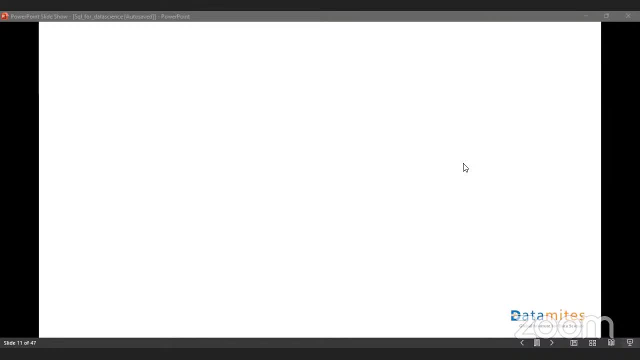 We have entity relationship, we have one more relational model. So if your data is in the form, but if your data follows a relational model, then I can see. oh, then you can use it as a DBMS. With that DBMS it's easy for you to do retrieving. 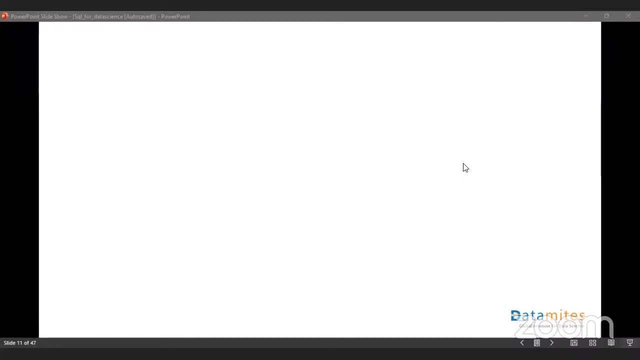 It's easy for you to do manipulations. Okay, How data will be modified, which lies to when data given in dictionaries and data science projects. So it's completely a data science question in a Python question. Okay, but still, I'll answer you. 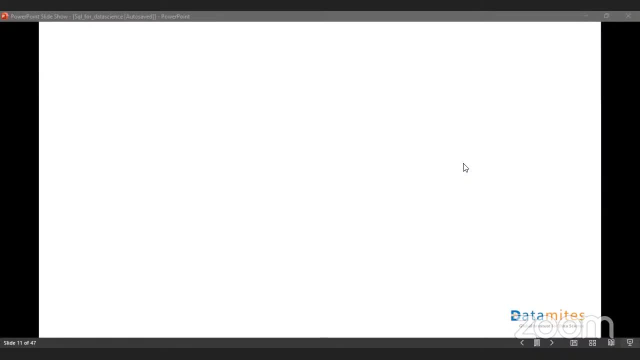 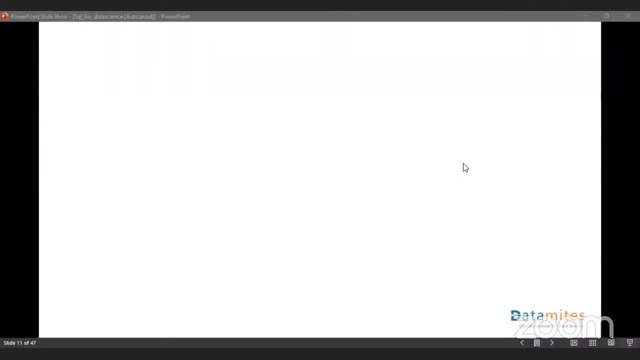 we can't give you know indexing because it's an unchangeable. i mean, i can see it doesn't follow any indexing thing. it's an unordered one. if you have learned the properties of a dictionaries like it's an unordered one, that means it doesn't follow any indexing. if it's not following any, 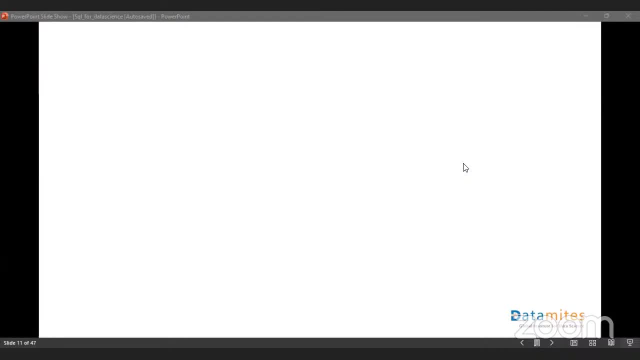 indexing. you can't access it by specifying your index value. what you can do is so dictionary. in a dictionary, values are basically defined in a key value pair. what you can do is you can either extract keys or you can either extract values individually. you can just you can store your. 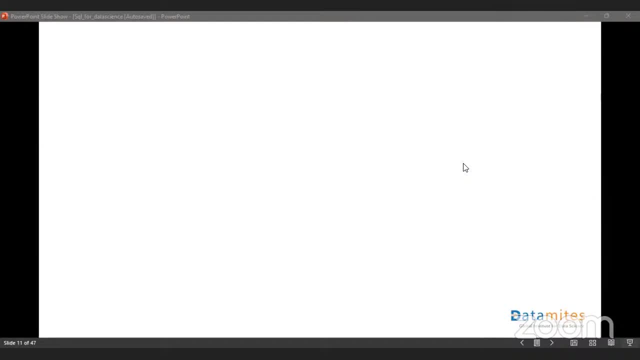 dictionary in a variable and then you can say, like a dot keys, a dot values. so using that you can extract keys and values and also you can extract the pairs as well. okay, that you have to study in python, so that's it. any other questions? which database is mostly used? basically mysql, sorry. relational data model. 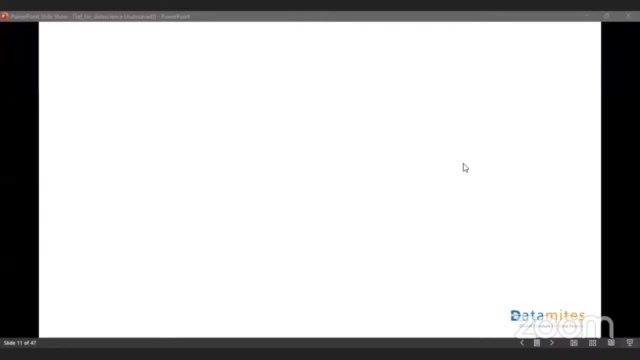 relational data model is basically the most used model and the database is like oracle, mysql, and also people are using microsoft server as well. yeah, anything else, so shall i proceed? so we stopped at models, right, yeah, so so basically, uh, for this entire webinar, or for this entire. 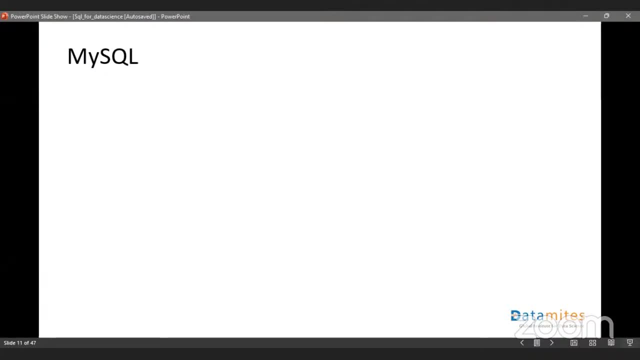 session. so what i'm doing is basically what? oh, we are basically using mysql database and let's see what was mysql and how it works and and many things. okay, so this is a logo for mysql. yeah, and you know, mysql is an open source relational database that uses structured query language to interact with databases. so what do? 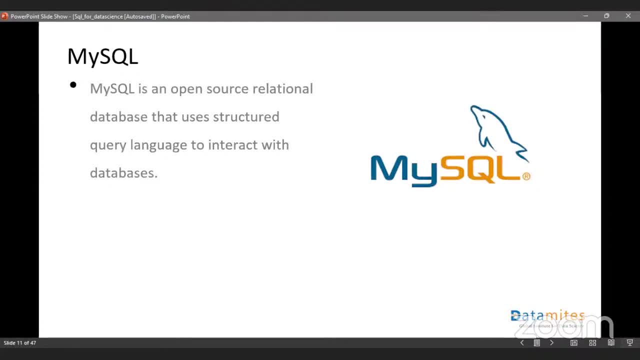 you mean by that? so we are using. what if the advantage of using mysql is it's an open source, anybody can use? that's one of the advantages. that's why we are going worth okay. so it's an open stage, it's an open source. that's one of the advantage of using mysql. 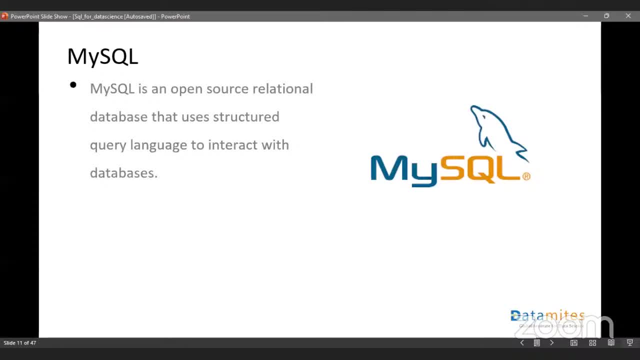 what it does is basically it uses structured query language. mysql is just a database. okay, it's just a database which basically stores our data, that is, relational model data will be stored and further operations like if you want to retrieve or if you want to modifications, then we need some language. that language we call it as a structured query language. 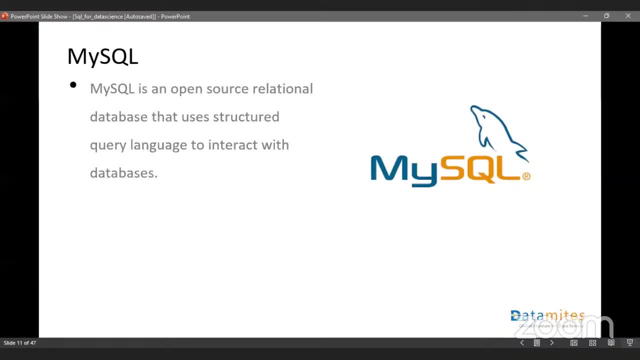 okay, so mysql is an open source relational database that basically uses sql. sql is basically a structured query language used to interact with our databases. so when you have a database, you have to interact with that, right? how do you interact? what will be the mediator between you and a 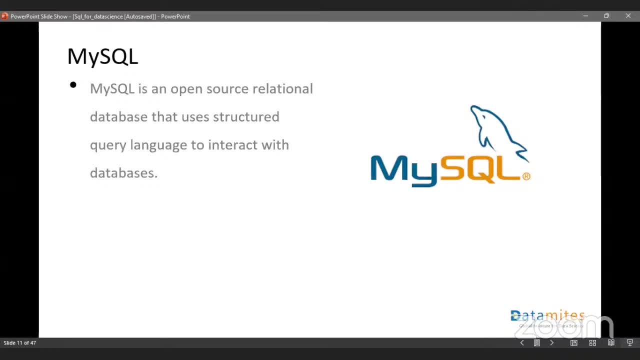 database, so it's basically a sql. okay, it's like a language, the way we use we use programming language like: why do we use python? so it basically does few things for you, right? in order to interact with the computer, like if you ask directly with a computer in your own language, like: add two plus. 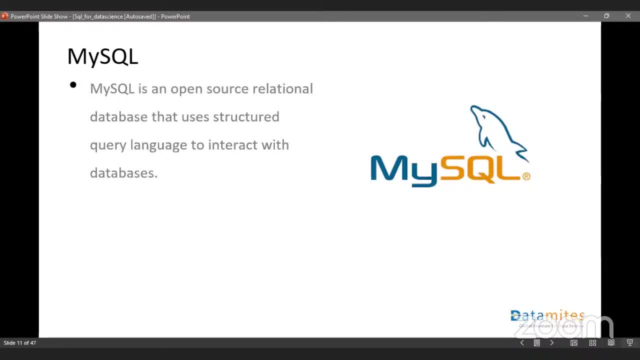 three. so will it add: no right, because computer cannot understand your own language. if you want to make your computer to do tasks for you, obviously you have to learn the language which computer knows. only then you can interact with a computer and computer can help you in finding solutions. 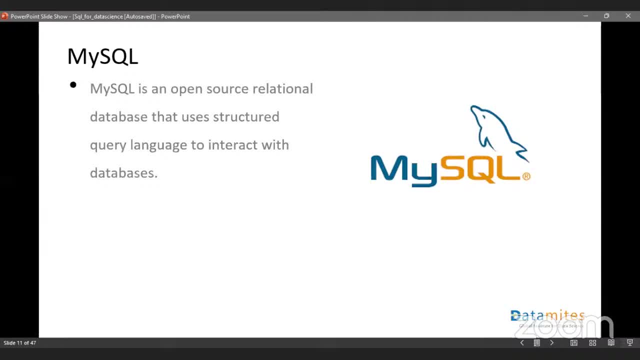 yes, no, that's why there are many programming languages like python, java, c, c, plus, plus. so without knowing those languages, you cannot interact with the computer and it can't give any answers for you or it can't do any tasks for you. similarly, if you want to interact with 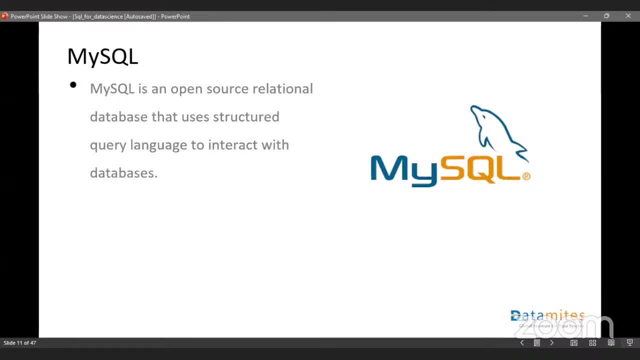 a database. you want some language. only through that language you can interact. that language is basically a sql. okay, are you getting mysql as a database and sql is a language? yeah, so what it does is basically it stores data in the form of table and can be modified using sql. okay, so for storing, it basically stores data. we know that because it's. 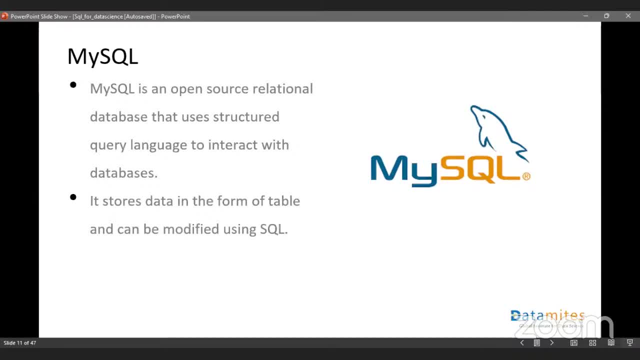 a database, obviously it has to store data and in order to do modifications, what you have to do is you have to use a sql language. okay, so you might get a question now. like there are many databases like website, so go ahead and go toamps, Shine, meta. yeah, there are many data bases. 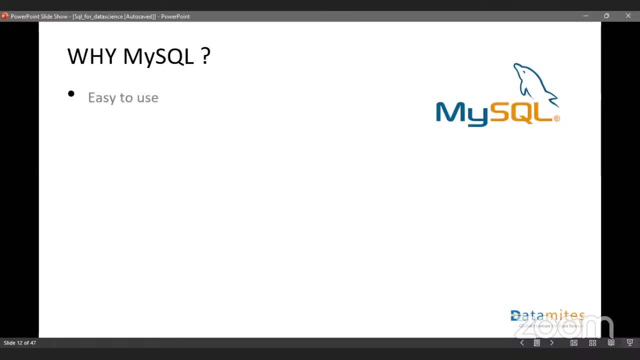 so we saw like five to six databases, right, but still, why are we going with mysql? any idea? first one: it's an open source and very easy to use, but still people see it's difficult but if you learn it's very easy to use, okay. and the second one, the cost effective. it's an open 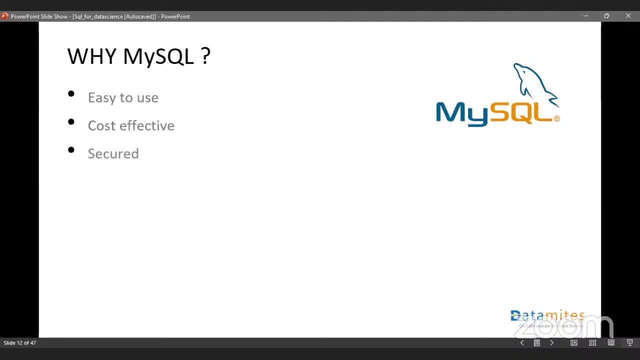 source, the free one. anybody can use that. okay, very important. if we give an access for multi-users, obviously we have to protect some sensitive data. only then things will be in a good way. otherwise a company might be might, might get into a loss. okay, so it's a secured one, platform friendly. what do you mean by that? it works on all the platforms. 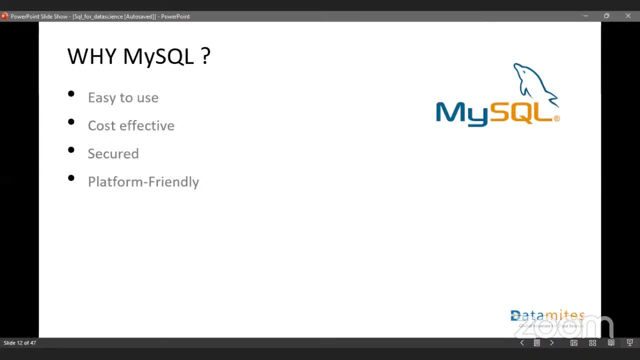 like you know, different operating operating systems such as windows, mac, linux and raspberry pi. that's one of the things, and also, yeah, that's it. so these are the different applications and these are the different advantages why we are using mysql. it's easy to use compared to other. 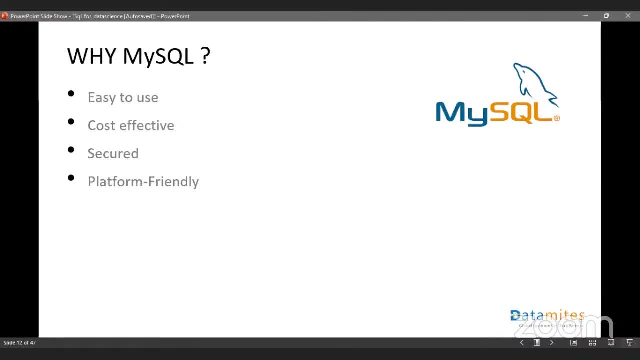 languages. it's cost effective. it's open source, anybody can use. anybody can work with mysql and it's a secured one. it gives you a security and protection to secure things and even our company is using this mysql. and platform friendly. it can work on different platforms like windows, mac, raspberry pi- okay, yeah, and if you want a comparison, uh, you. 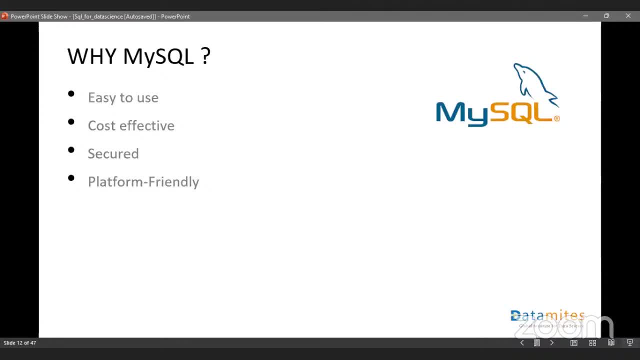 have to do that. you can compare a different databases and you can see, like, how one is different from the other. i want you people to do that. okay, so i think that there is a language in order to interact between user and the database, so that language is called as sql. okay, it's sql. 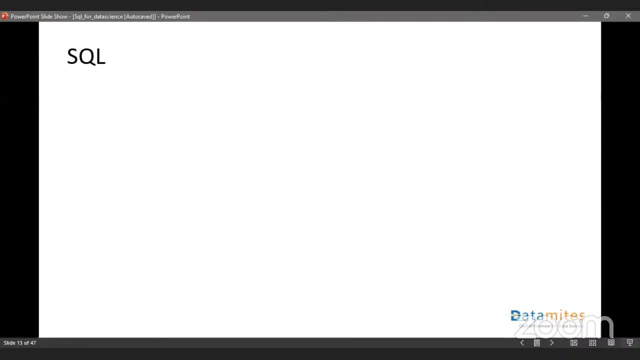 or we pronounce it as sql, sql, sql, okay. s-e-q-u-e-l. it's a sql, okay. sql stands for structured query language, so the expansion of sql is basically a structured query language and, yeah, as i said, sql is basically a database programming language designed for retrieval and management of data in our 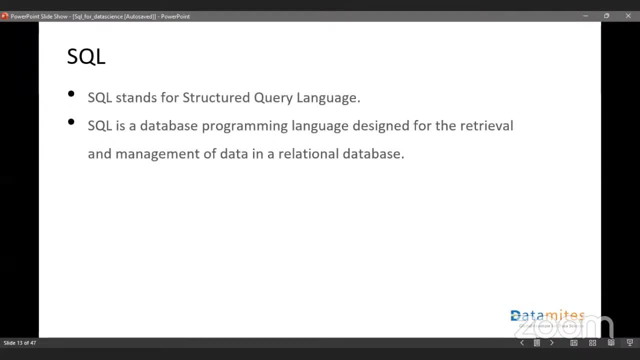 relational database. so, unlike python, even sql is a programming language, but it is a programming language and database. okay. sql is database programming language designed for retrieval. what do you mean by retrieval means? so when you store your data inside our database, you have to use that like whenever it's required for you, right? so how do you do that? that can be done. 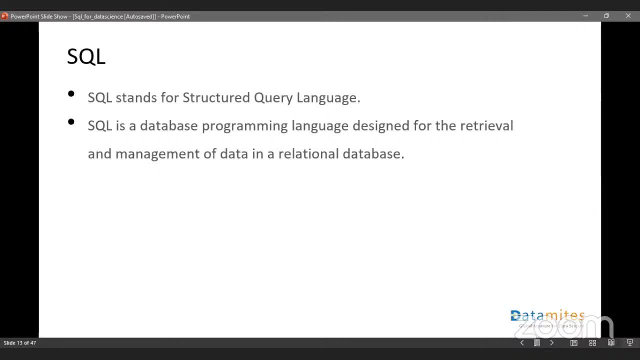 that queries can be written using the sql. okay, without this language, you can't do anything with our database. remember that. and also it can manage data and relational database, because so the database that we are considering is basically rdms, right, so that's why it's called sql, and also, what it can do is not what it can do- basically all relational database. 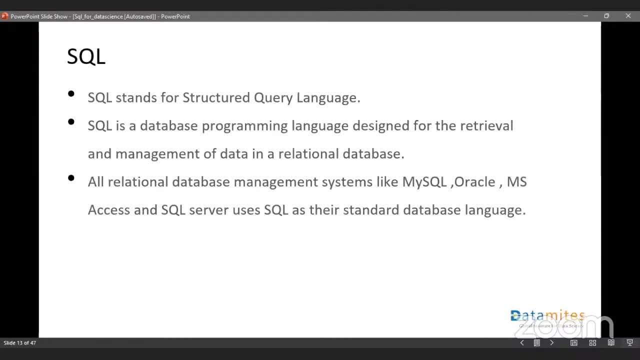 management systems such as mysql oracle, ms access, sql server. so these rdbms- that is, relational databases- are making use of the sql language in order to interact with databases. okay, it's a common language where you can interact with different databases like mysql oracle, ms access and sql server. 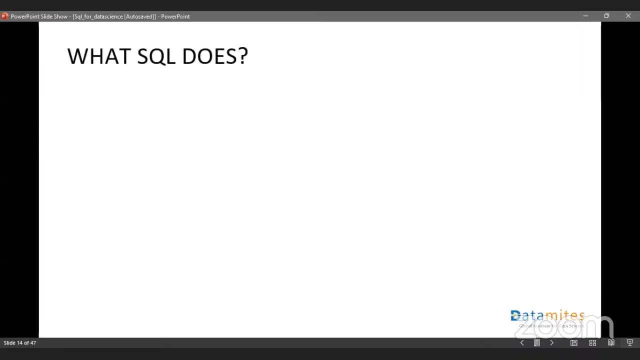 here. okay, now you have a question like what sql does. if someone asks you like what python does, it's easy for you to answer. you can see different things like it can do, uh, arithmetic operators. it can perform logical operators. it can be used to define function. it can also be used to 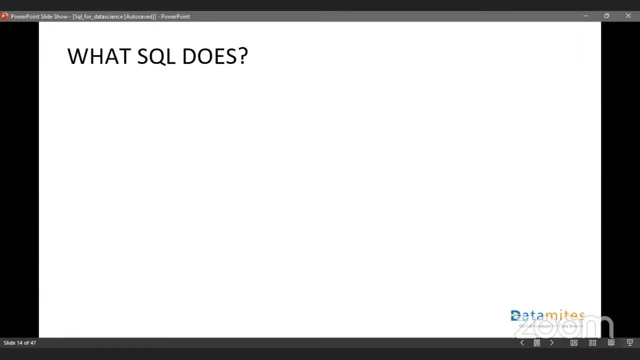 you can look through things and also you can plot graphs, you can analyze data, you can do machine learning projects. but what if someone asks you like what sql does? how do you answer? so, as i said, sql is basically a program, a database, programming language which is basically used to create new databases and tables. 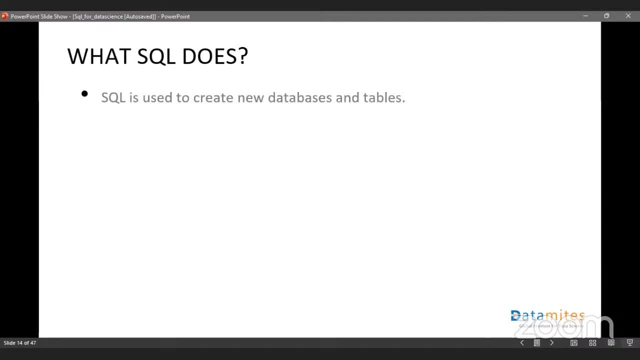 so when i say my sql database, so you will have it. so you have to create a database first and then you have to create a table. so that is basically done with the help of sql store data. okay, you want some structured thing, right, like when you go to a supermarket, supermarket. 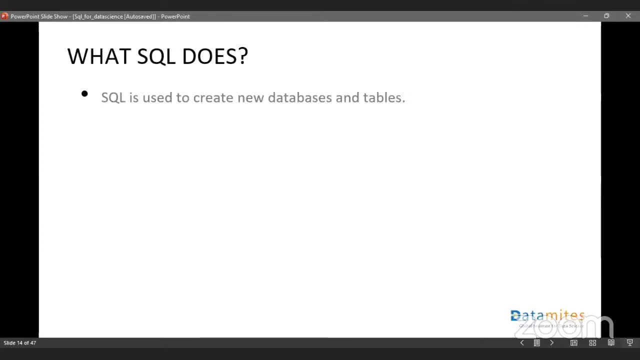 how will you store your things, like whatever you purchase, so you will have a basket or a trolley, right like you'll take all things and you'll put it into that trolley. so same thing should be done even in our database. you have to put all your data into a database. how do you do that? that is. 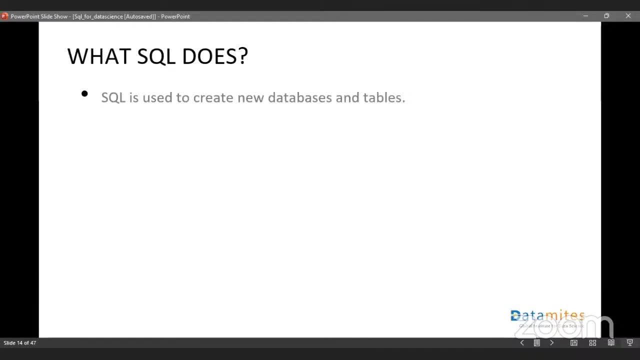 basically done using sql. sql can do. sql can create new database for you and also it can create tables for you. and the next one, sql can execute queries against our database, queries in the sense, like you, it can ask a question and it can get an answer. okay, it can execute queries against our database. 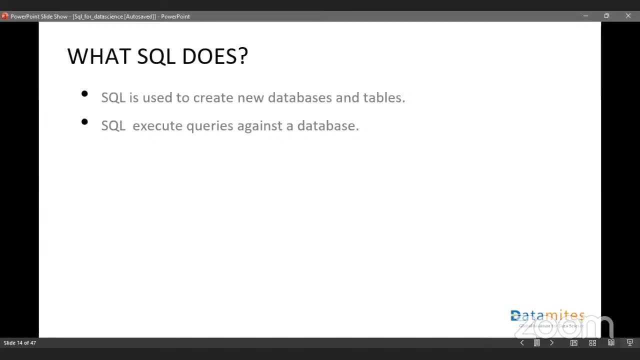 it can ask questions. for example, let's see: uh, so let's say i have a data related to a flipkart. okay, i have flipkart sales data, so i just want to filter it out data like you know, um, which has got higher sales. or i just want to filter it out sales related to bangalore. okay, if my focus is only on a sales. 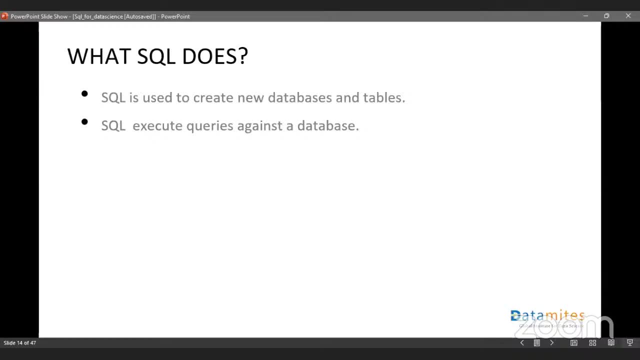 related to bangalore, what i can do. i want to write a query against a database such as i want to. i want a record or i want a data related to a flipkart sales that that is a sales in bangalore. so that can be done using sql. okay, sql language and the next one, sql, basically used to retrieve update. 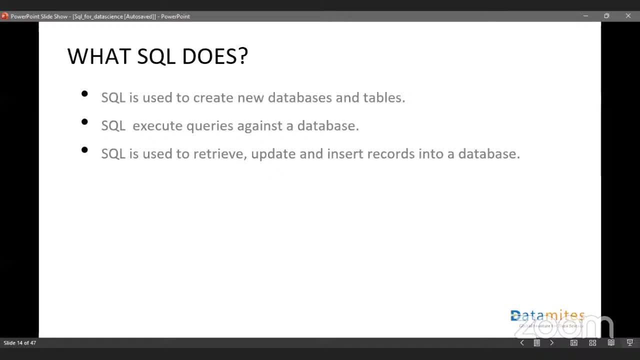 and insert records into our database sql. it's not just you know creating database, it's not just you know creating database, it's not just you know creating database tables or writing queries. by writing queries, what you can do is you can retrieve data, like once you create a database and once you insert, once you dump your tables, or once you dump your data into 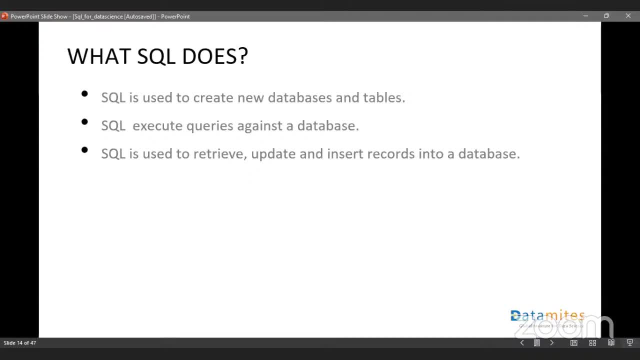 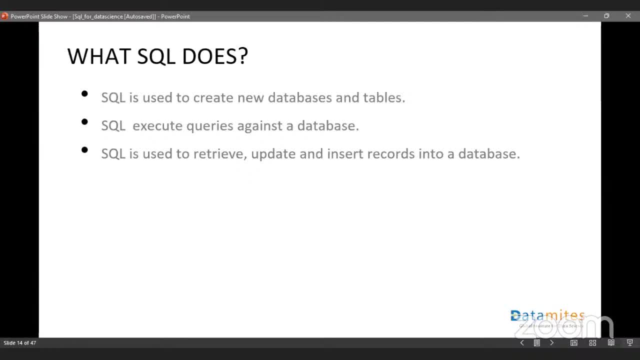 sales has date of mine. okay, so jivita name will be there and also my things, like uh, what details will be, like my phone number, address and the products that i've purchased? what if my spelling is wrong, like if i want to make some changes with that name? okay, instead of jivita, like something is. 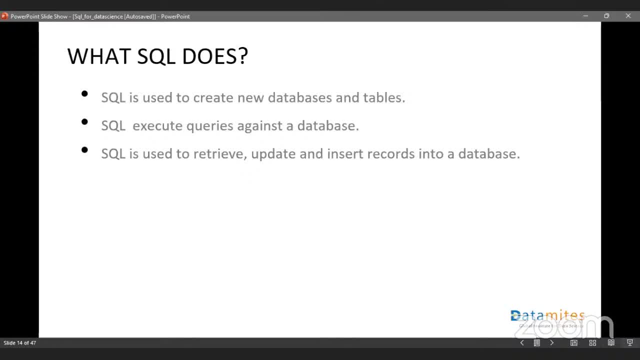 missing, let's say, uh, some words are missing in that name, so that modifications can be done. okay, that is basically done with an update statement and also we can insert a new records into our table. so these things can be done using sql and also it can create stored procedures. 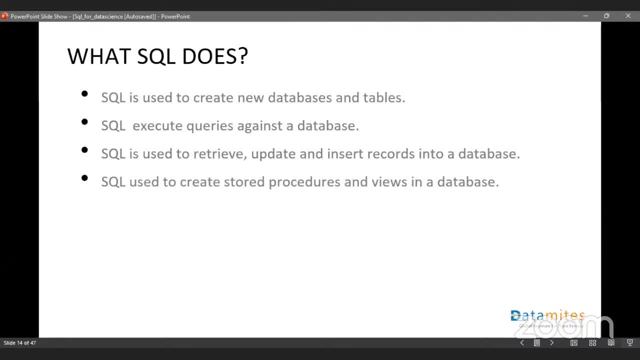 waves in our database so you can give, you can create a waves, and also you can create stored procedures and also you can set permissions on tables, like who can view, who can access. okay, all these things can be done using sql language. yeah, understood about what sql does. 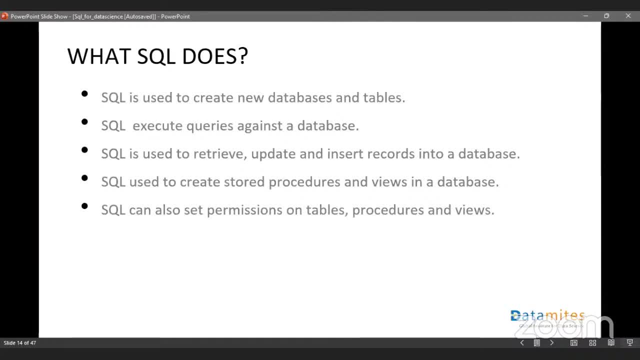 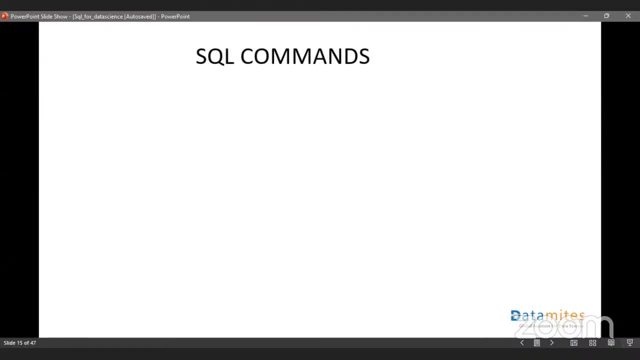 so there are basically different sql commands, uh, which basically serves different purpose, and of database. okay, so basically i told you that sql is a language which can do many things for you, so that many things can be differentiated into four things, that is of we call them as: 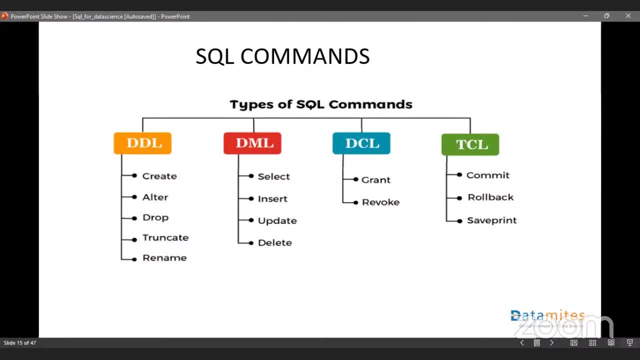 types of sql commands, like whatever questions you have, you can do many things for you, that is, you execute whatever of functionalities or whatever things you do in database. so that is basically classified into four things: one is ddl and the other one is dml, the third one dcl and 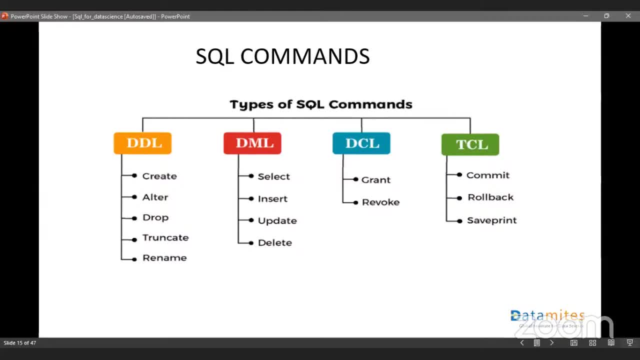 final one is tcl- ddl basically stands for data definition language- where you can do things like you can create a database, you can create table using alter. you can alter like you can add new column, you can delete more. you can delete a column and also you can change existing data type of a. 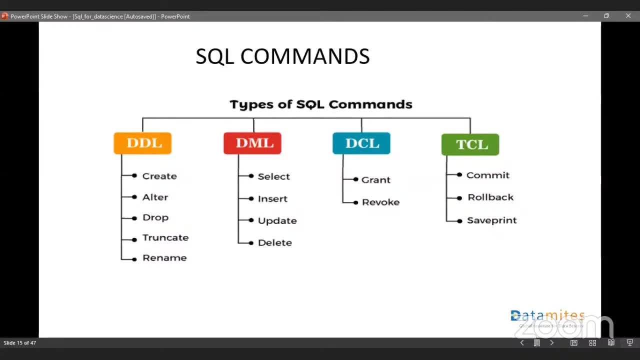 column and using drop, you can drop a database and also you can drop table. truncate means so, basically, you can also remove all the entries inside the table. you will have a table. okay, you just if you want to remove all the elements. if you want to clear all the elements of a table, then you truncate. so don't worry, we'll be discussing. 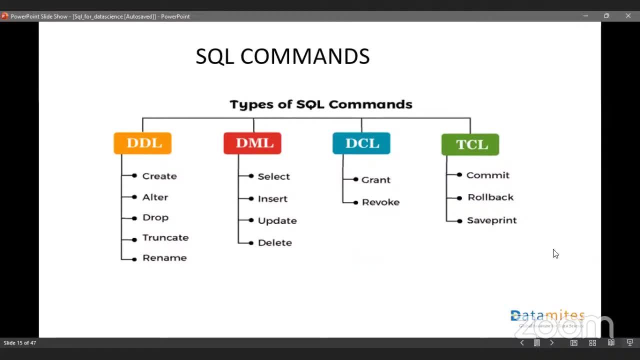 all these functions in the coming classes, okay, in the coming sessions. so next one is data manipulation language. so basically, what you can do is you can select data using select statements. you can select entire data or you can select a subset of data, like subset of columns, and also you can insert new records into a table using insert function. 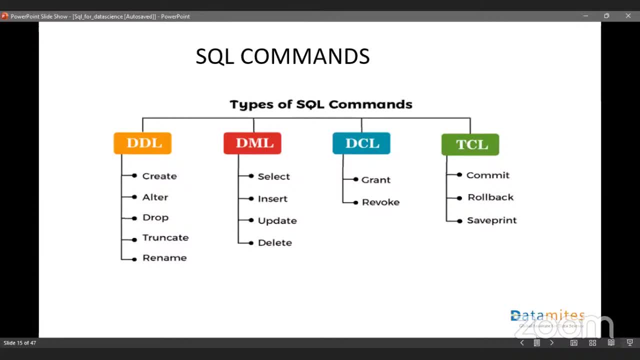 and we have an update where you can update things. update means like you can modify the existing data. you can change and also you can delete the record, like particular record can be deleted. do you remember all these things you did in python, but you did it for like very small data, yeah, like. 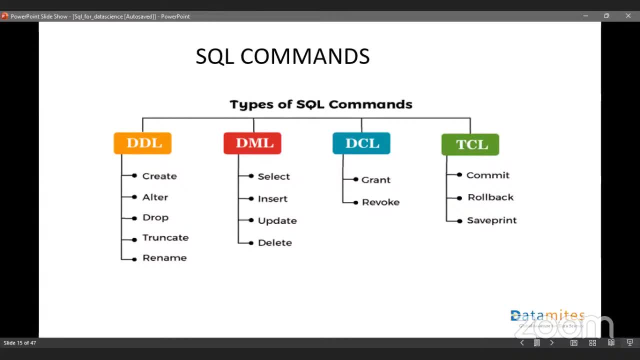 probably in less tuples. yeah, so we, being a data scientist or the people who are working on data science and machine learning project, we just basically focus on data definition language and data manipulation language. so these two are our main focus, and dcl that's basically a data control language. uh, we have two things: grant and revoke. you know what? 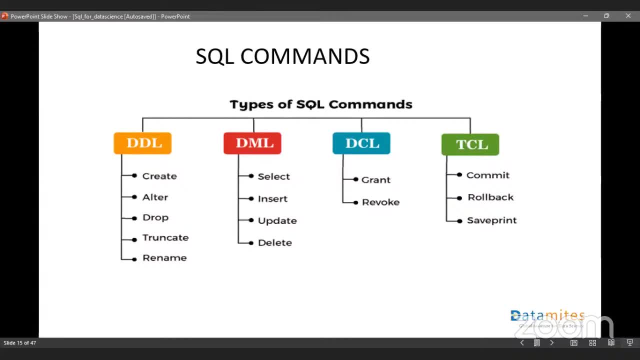 grant does is basically like: uh, we can set permissions like who can be, who can access, who can, who can do something with database, all these things basically done with a grant. grant basically gives permission for doing okay, like it's restriction and revoke. it's quite opposite to grant like whatever permission is. 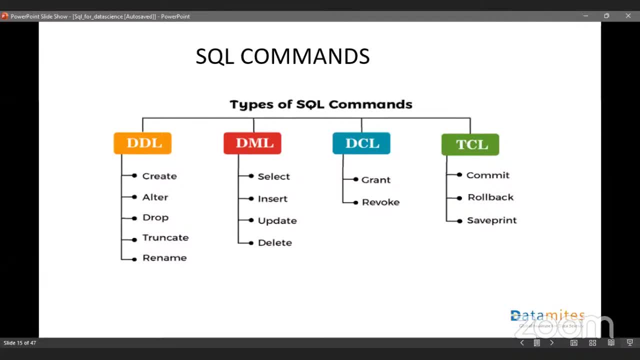 given by the right, that I mean given by the grant that will be removed by the Ethiopian ponytastic- a database. if I use a concept of revo, sorry Revo, I can just remove that access. what is given to the user? okay, and we have our transaction control language. we have three things that commit roll. 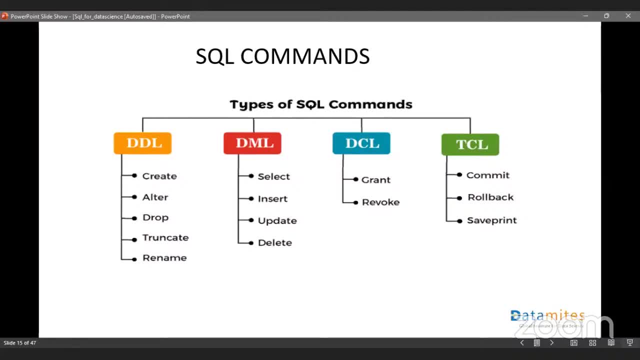 back and see friends. it's basicallyул it like one: you when you do some changes. we use comments. back means like when you do changes, but still you can retract things as it is. so we are not focusing much on dcl and tcl. yeah, our main focus is only on data definition, language and data manipulation. 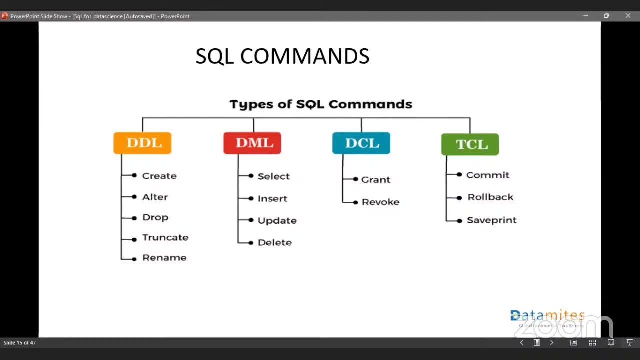 language, okay, and if you want to learn on dcl and tcl, yes, definitely. you're welcome for that and you can learn those concepts. all right, so these are the different sql commands. yeah, people might ask you a question like: what are the different sql commands and what sql commands are basically used? 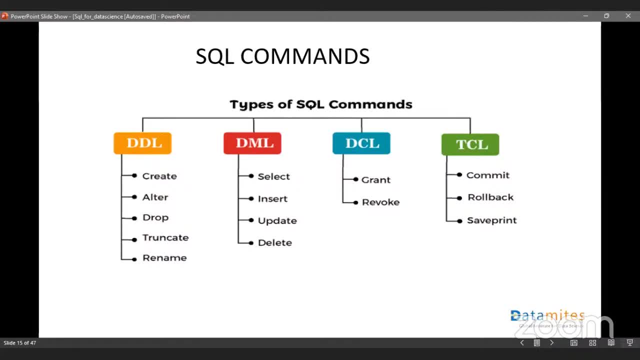 by the data scientist. so we use data definition. it's all about, you know, creating database, creating table of all those things- and data manipulation. we are basically focused on like reading, as i was telling, like we basically focus on reading things, reading data. okay, like we have select, we have insert, update the reach and many more will be saving. we'll be seeing in the coming. 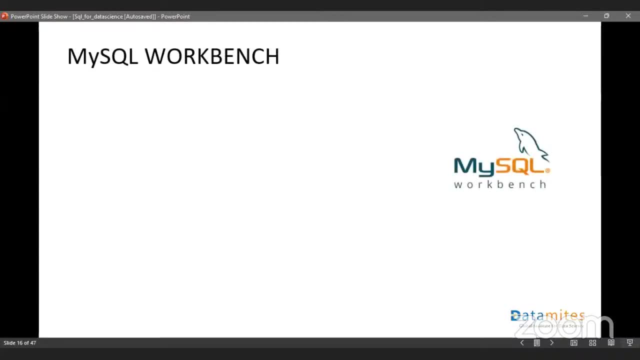 classes. all right, okay, so we learned about your database, we learned about the models and I know also we learned, like so, language in order to interact between user and a database. okay, we, we have a language, but where do you execute that like? where do you like where the program will be? 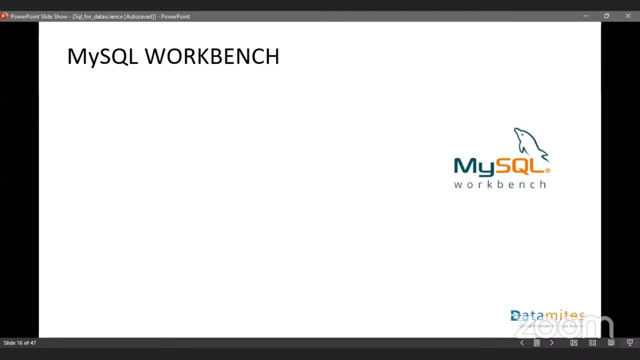 written. where do you write that sql queries? so for that we have a editor, or i would say it's a graphical tool. we call that as a mysql workbench. it's like. it's just exactly like our editor the way. in order to do a python, you have a different ideas. right, like integrated development environment. 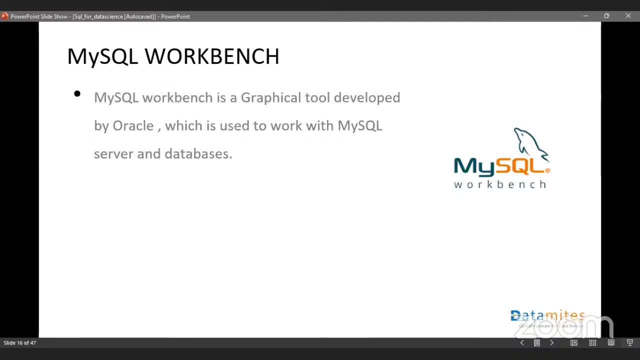 such as you have a jupyter notebook, you have google collab, you have pycharm and you have virtual code. yes, so you have different ideas where you can write your python programming. similarly, in order to deal with the mysql work, i mean with the mysql database, so we have a 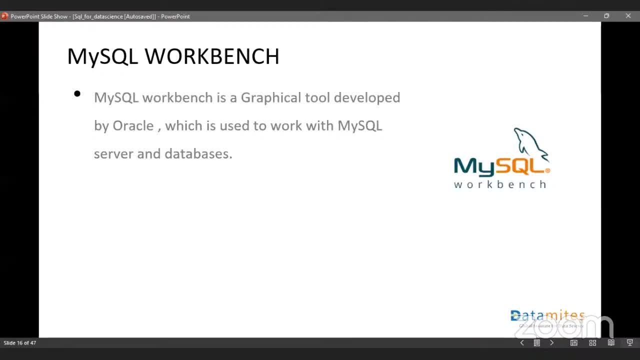 different platforms, like mysql workbench. you can you have a sqlite and also you can use oracle oracle as well, because even it's using sql language. you can use sql language and you can use sql language and you can use sql language and you even. it works exactly similar. okay, but we are focusing on just mysql workbench, okay, which is. 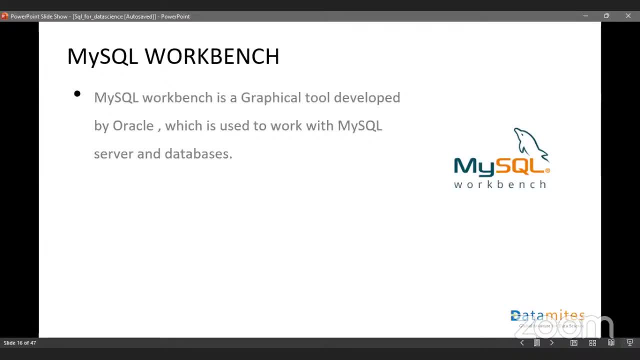 easy to use and, yeah, most of the people are going with mysql workbench. most of the companies are using this, so that's why even we are focusing on mysql workbench. okay, it's basically like a graphical tool developed by oracle. it's developed by oracle, it's a child of oracle company, so which? 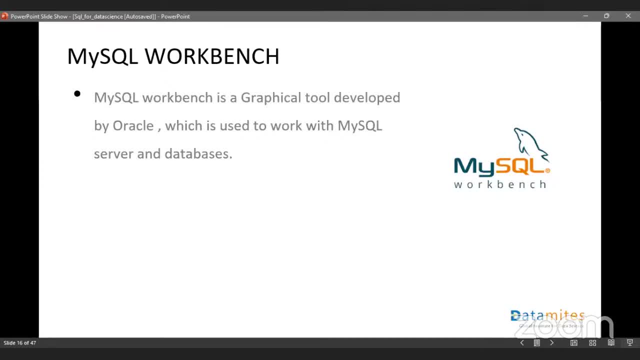 is basically used to work with mysql server and databases. okay, this editor, or, or we would say, a platform or a graphical tool basically developed in order to work with mysql server, basically a relational database. you can only deal with a mysql database, not with others. okay, so just mysql basically provides data modeling, sql development and various administration. 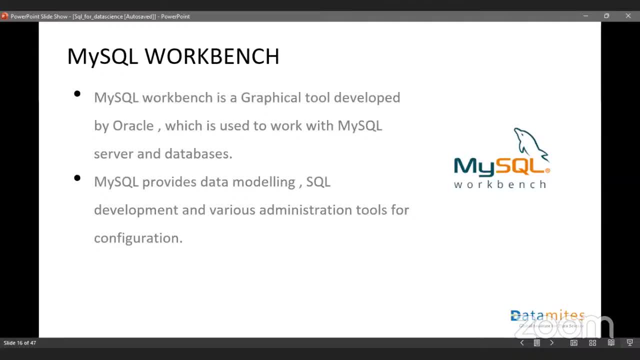 tools for configuration. you can do modeling, you can also develop things there, and also there are a few administration tools or like you can perform, like whatever sql commands i have discussed in the previous slide. all these things, all those things could be done in mysql workbench using sql language. okay, it's just like a platform. 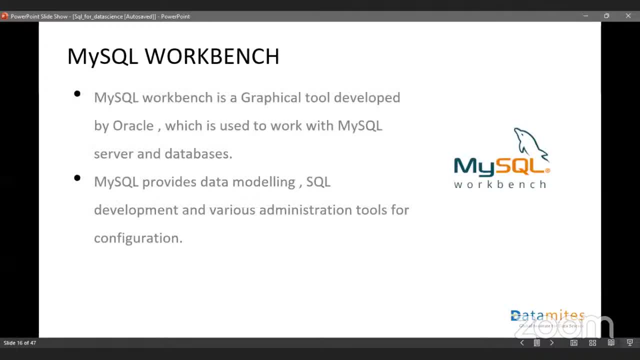 okay, so before moving on to the uh creating database, i just want to show, like, how to install workbench. will you do with me? yes, are you ready with your laptops? do you have laptops with you? so before starting with installation or any questions, so you can just ask me so that i can. 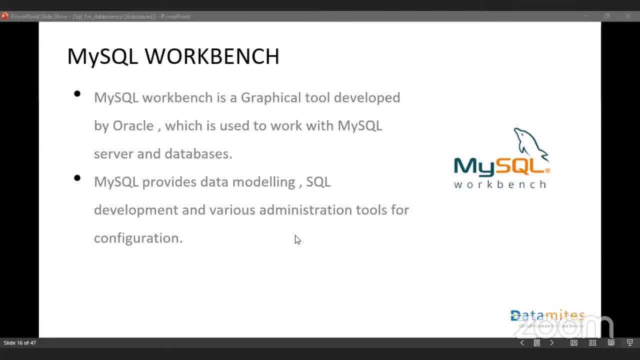 clear it out your questions. oh, ready with the laptop, that's good. people are so excited to learn sql, so that's great. i'm using you can call me tv talk. yeah, you have laptop, that's good. any questions like like whatever slides i have discussed? if any questions quickly, you can ask me so that i can clear, clear and then 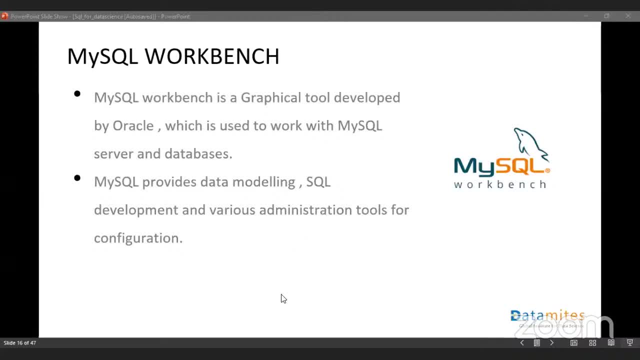 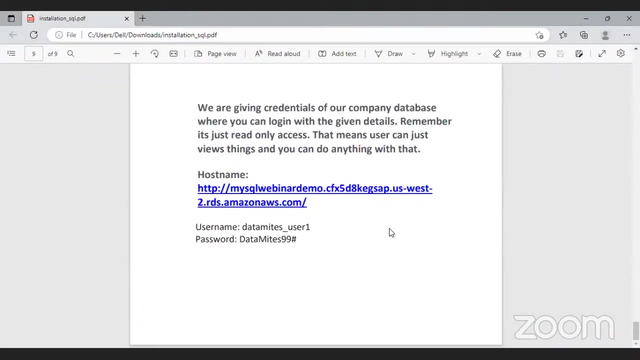 Then we'll move on to MySQL Workbench, No questions. So Yeah, it's here, Okay. Yeah, it's like an IDE, It's like a text editor where you can write a SQL queries. Yeah, you can use Python instead of editor. 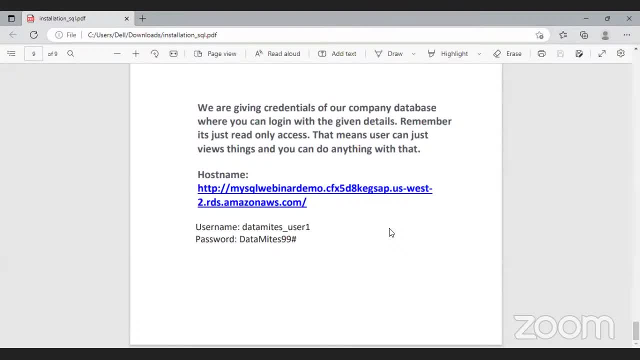 but one of the disadvantages is like you have to connect a database, everything- but this is quite structured work. You can use Python in order to you know like you can read our database and you can do our manipulations, but inside you know when you use MySQL Workbench. 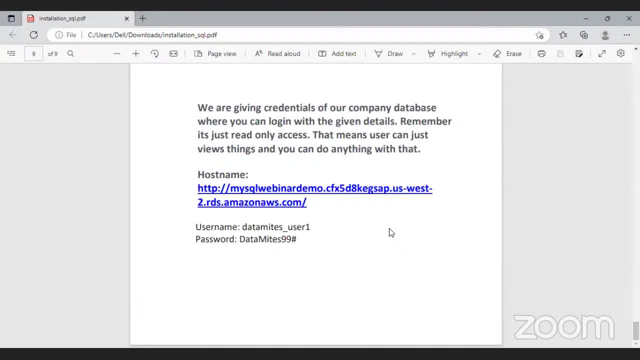 you'll get to know, like how data is stored, how tables are created, How manipulations can be done. You know, using MySQL Workbench is very easy because in Python you do it. you will use four lines of code in order to do same thing. 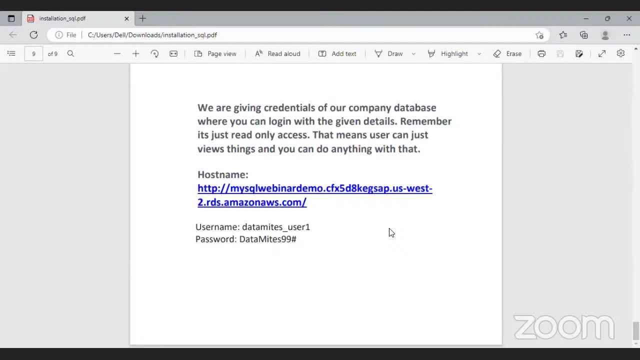 but using MySQL Workbench you can just get your data just in single line query. Okay, that's one of the advantage, otherwise I would have taken Python. Yeah, I'll share the link. So, and yeah, one more thing. 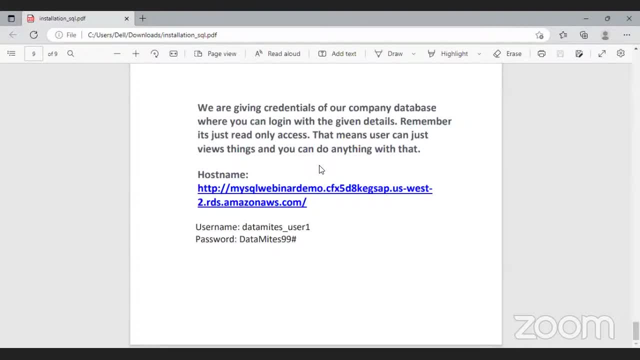 So basically we are giving access for you for our company database. Okay, you can just log in with this username, password and this is a host name. So before that, you have to download your MySQL Workbench. only then you can just log in with this username and password. 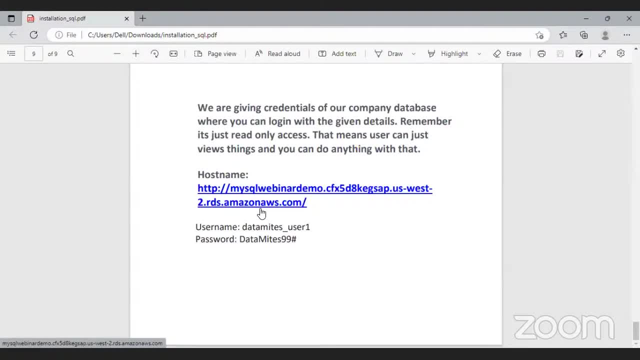 So then what you can do is you can just look at like what I do, Okay, and you can't do anything like you can't try, or you can't do like it's restricted, Yeah, so, yeah. So let's do the installation part. 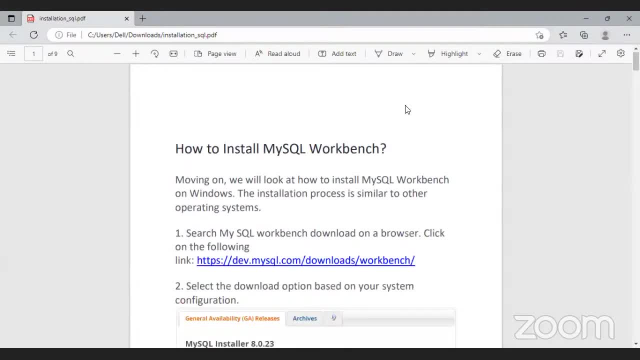 So I'll show you the steps. I want you people to do. it Be a little fast. So we need to install MySQL Workbench. So, moving on, we'll look like how to install MySQL Workbench on Windows. Okay, so I hope everyone are using Windows. 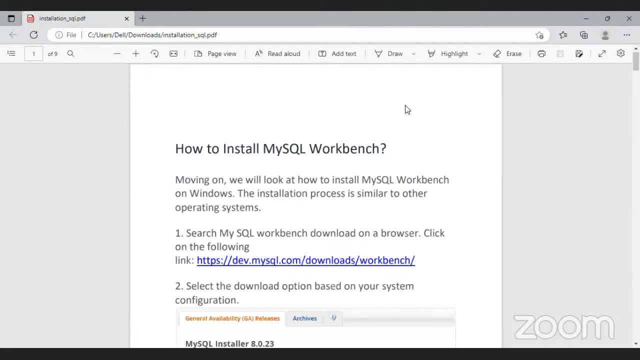 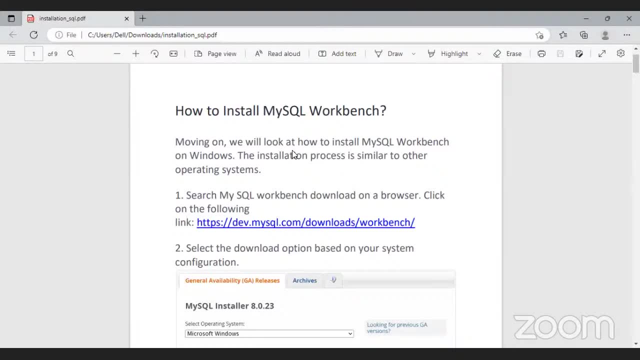 So installation process is very similar to other operating systems as well. So just go to Google search or else just open this link, Copy link and let me share it with you So you can see there is a link there. you can see that it's windows. 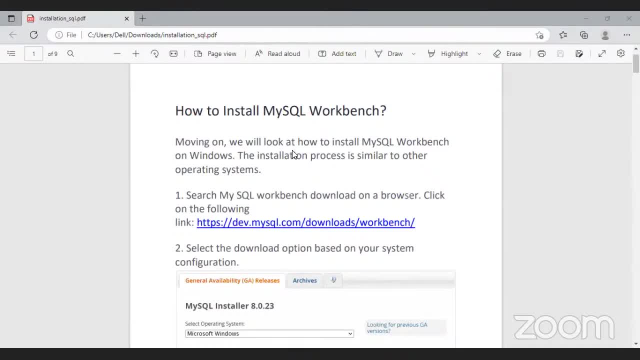 it's Mac. just go over there. So if you see it's windows, you can see that it's the app. it's the Windows from windows. So you just click on that link. See, Windows is the app from Windows. You can see it's my screen, right. 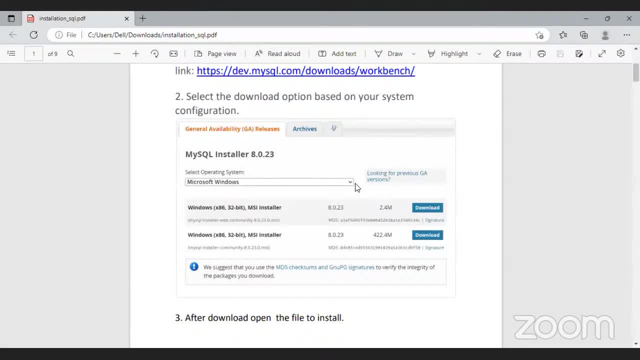 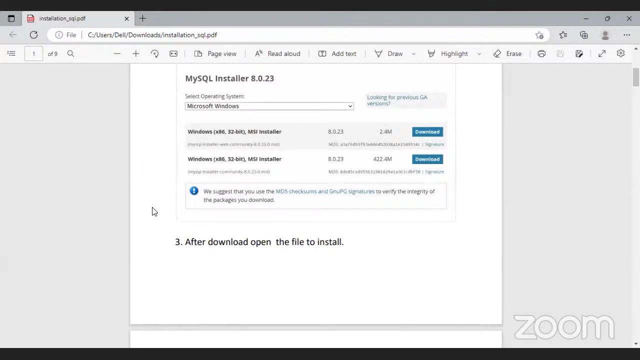 So if you open that link, you'll see some window like this: Can you see it? yes, can i get few confirmations if it's done? okay, that's good. if you are a windows user, just select like based on your configuration. just select that download and start downloading. 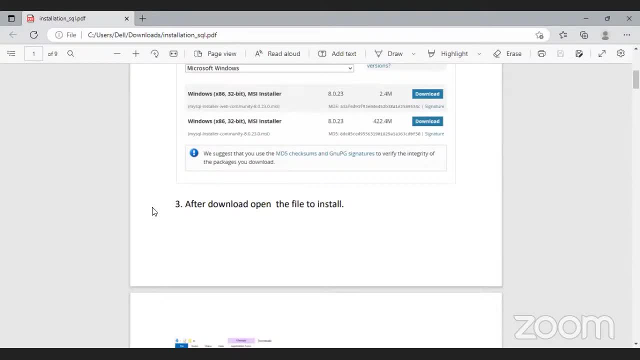 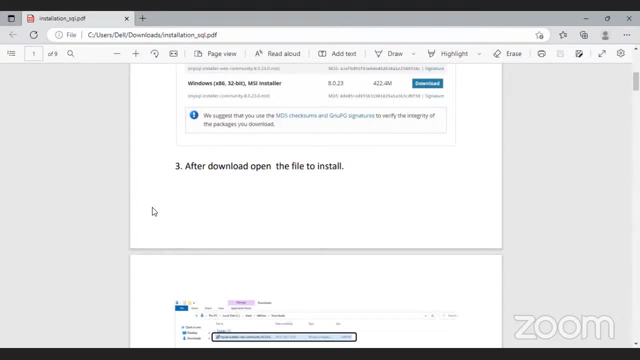 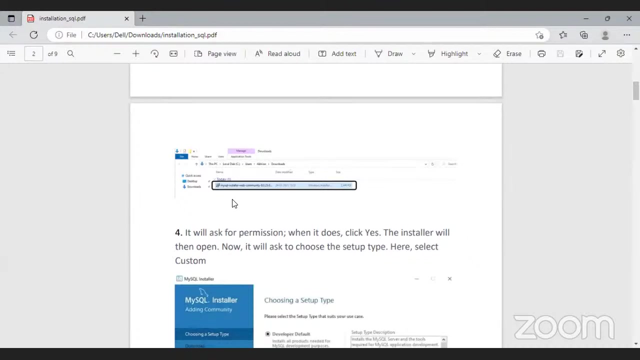 only if you download the mysql workbench, then you can uh log in with username and password, otherwise you can't do it so downloading. so after you download, just open the file to install so you will find your downloaded file on downloads. just click on that so it will take you to this. 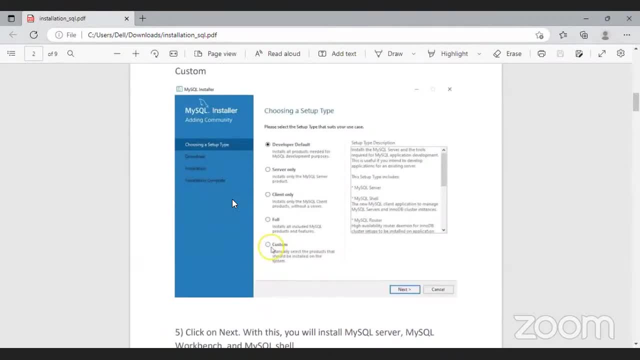 page. yes, with the same thing. just search for uh mysql workbench and select mac there- download for mac. it's a community version. we are using mac, so just select the mac that you want to use and then go into the community section and you will find that this is the inside of the mac, which is a 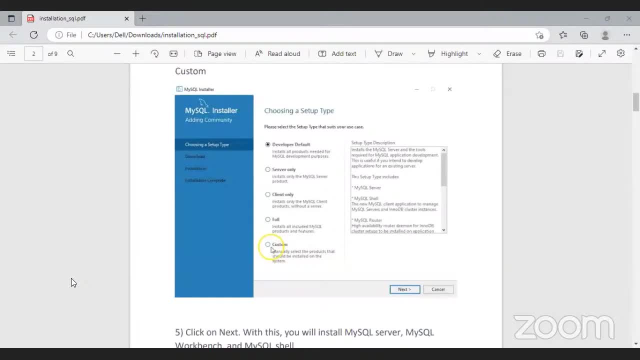 c, apt-get, install mac. so i'll set it to mac-edit-luxure and it will take you to mac-edit-luxure and you'll see right here that the mac is compatible with this mac. i'll just go ahead and click on install mac and that's it. you'll see that the mac is. 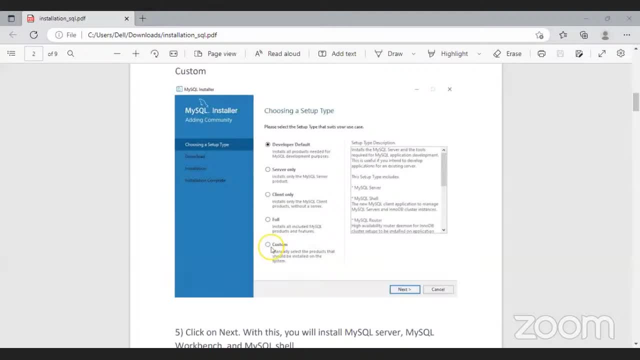 It depends if you're 64,, but just select 64,, if not, select 32.. To download for Mac: just select the Mac option. No, no, login is not required. So see, this is what we've found Now if you click on the login button. 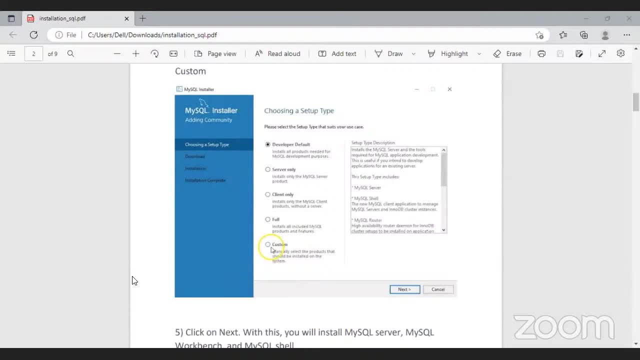 this is what we're going to do, And then, when you click on the login button, you can see what the browser has created. So open the browser and you're done, And then you're going to see this screen here. That's called login. 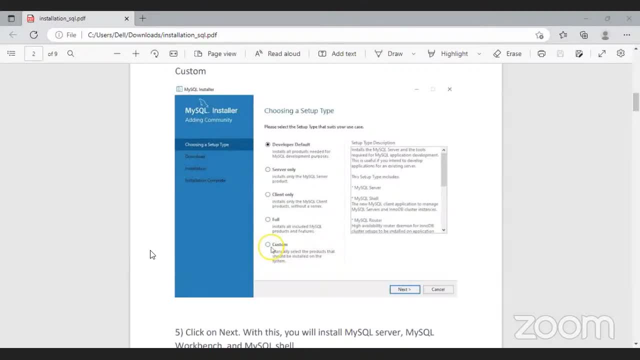 so done with installing. so people have installed it. that's good, that's great. no, no, just select that custom, select custom. okay. so once you have downloaded it, just select custom, open that link so it sees like custom. once you click on that, once you check on custom, just come. 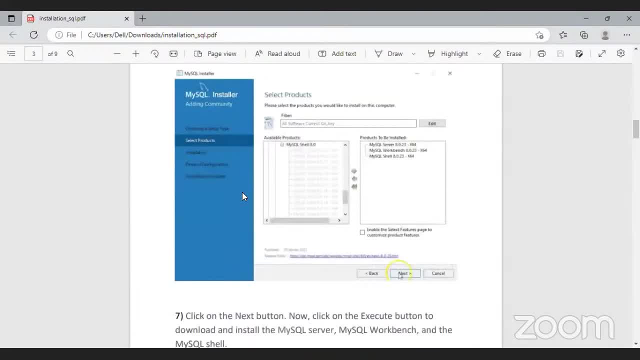 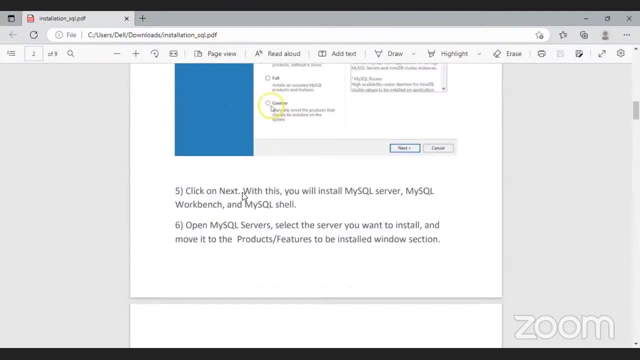 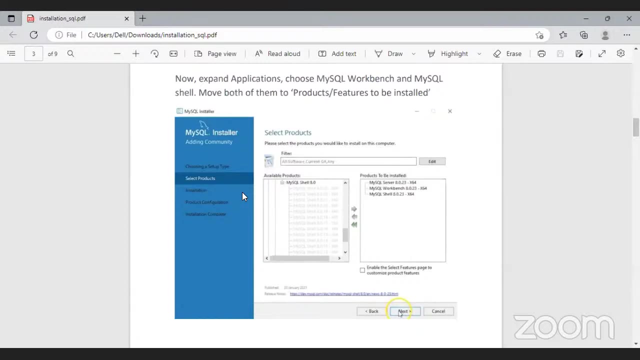 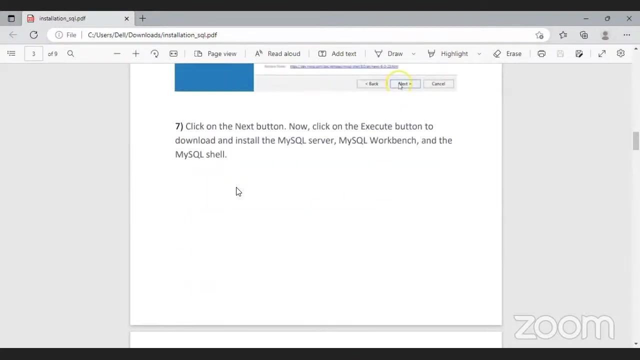 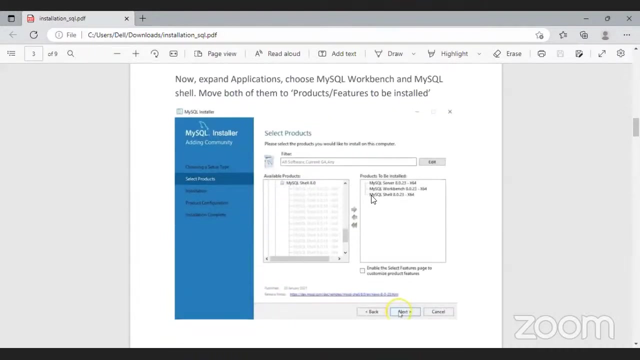 to next. so done with that. so once that is done, it will take you to this. you need to select the products. oh, oh yeah, that should be a visual c++ in order to install this. just skip sign in. so once you select your custom, you can come here in mysql shell, like you can select these things. 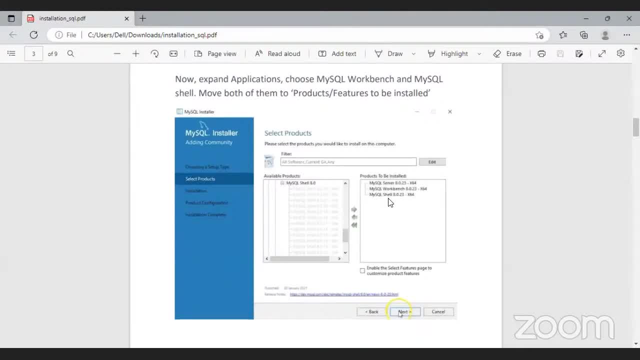 mysql server, mysql workbench and mysql or shell. so these are the three things that we are using: one is server, one is workbench and one is shell. so we'll be doing things in workbench. so, yeah, if it's yes, rita, or download virtual c++, it's okay, don't worry, if it's not possible to. 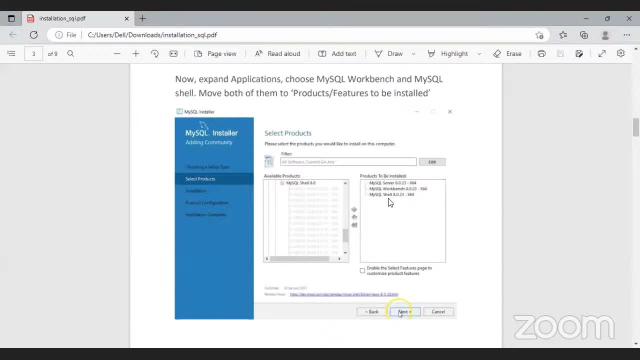 download. so today basically i'm showing you like how to create database and creating table and basic stuff. so from tomorrow i'll be starting with sql comments so you can start practicing from tomorrow if. if it's not working downloading things, okay, but try to download it. it's working for adush. 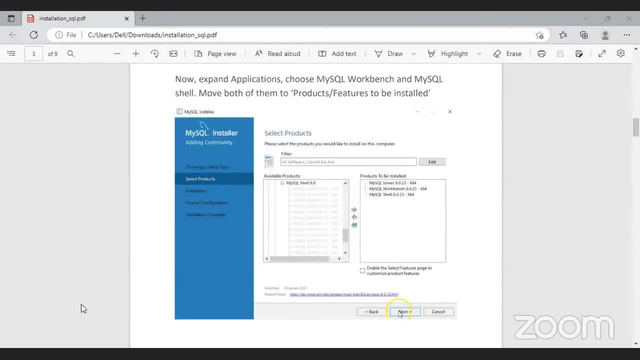 yes, that's good installed. that's good installed. that's good installed. that's good done with the installation still doing. let me give five more minutes, so till then, if you have any questions, you can just post it in our q and a section so that they can answer you. 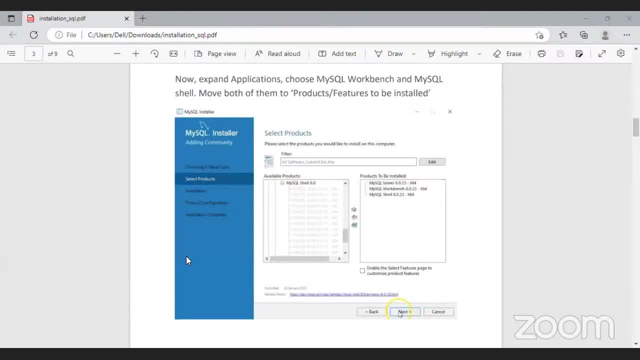 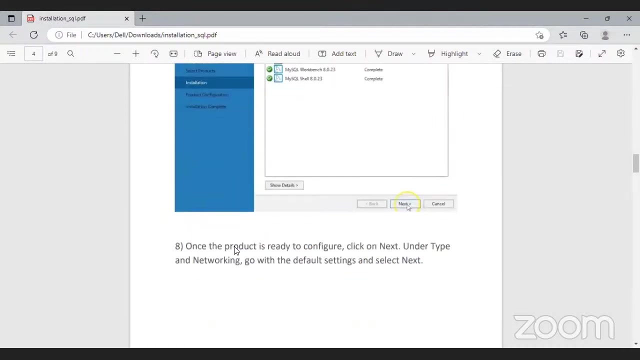 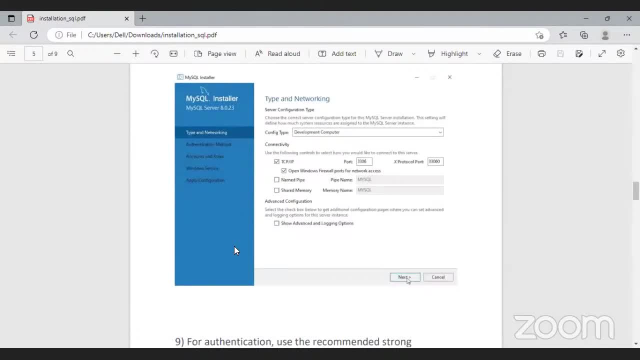 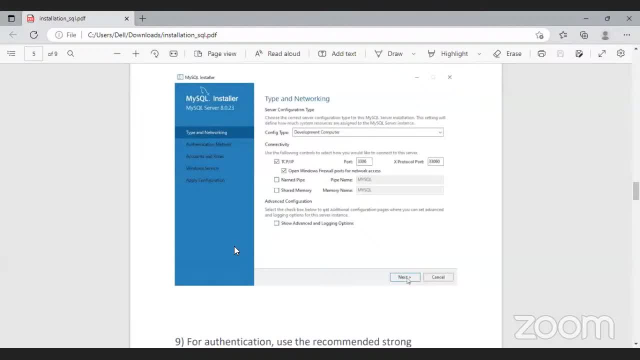 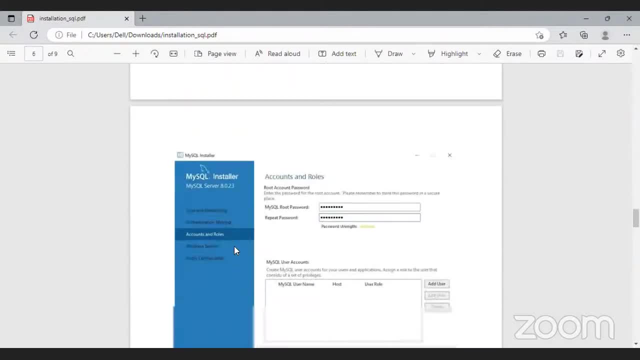 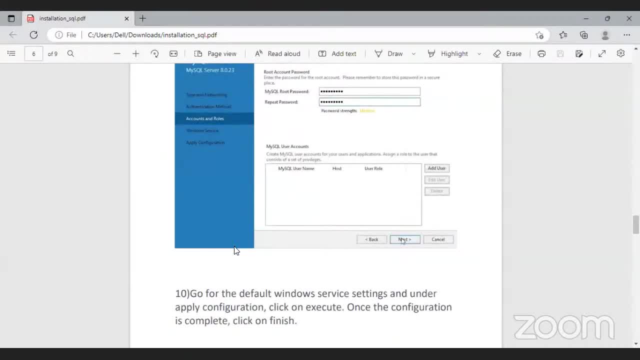 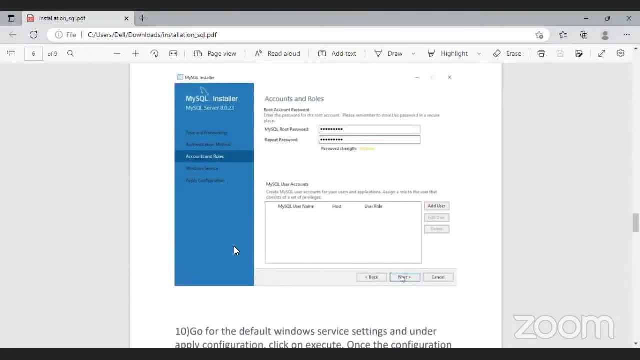 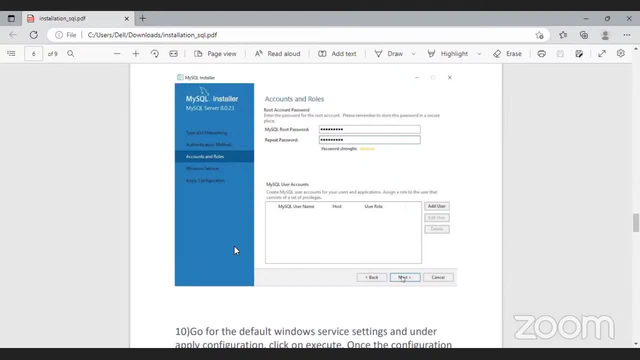 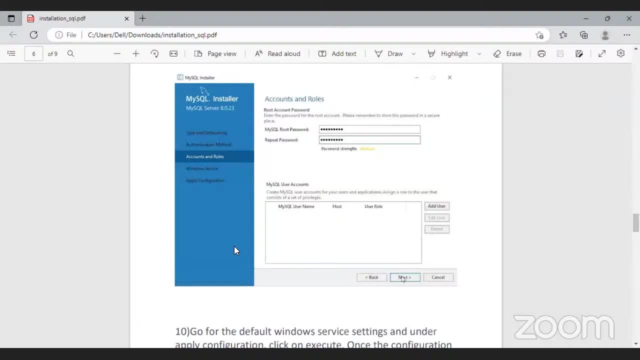 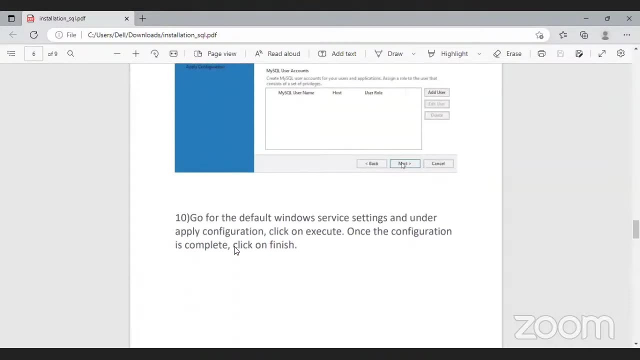 school, which is a very good platform to learn sql. if you are a fresher, things are very clear in that you can follow that, even in w3 schools. you can practice code there and there and there. done with the installation, have you created like whatever username and whatever? 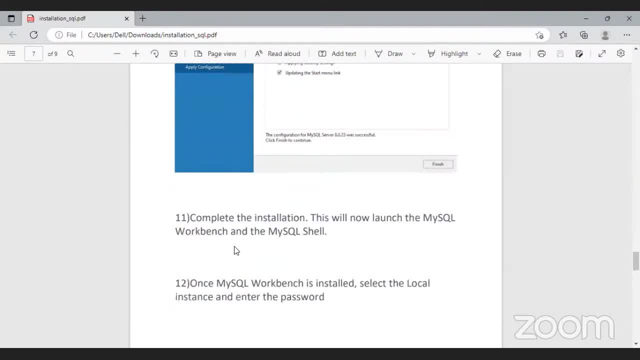 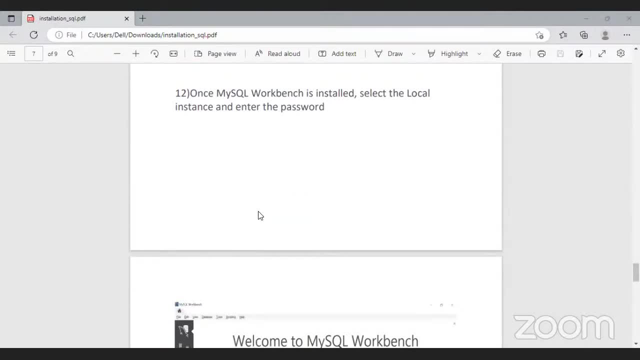 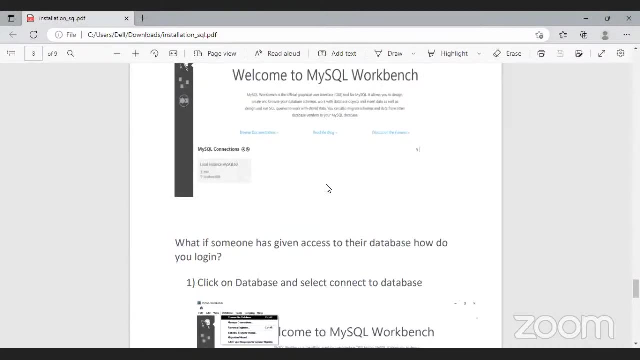 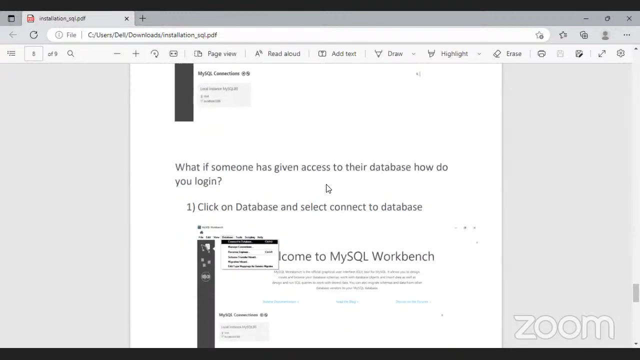 uh, password. you say that will be like a local host. okay, I think I will see if I cooked it and save it. local host meat. it's basically used by you. it's for your usage. that document. just a minute. I have a drive link let me share. I forgot to do that. yeah, so this is it, res, employment services Data that we came up with in onions meeting for us all. that's there's on the county foravillage area office officinhabitat, VIP maverick area crown…". China cav숙in. 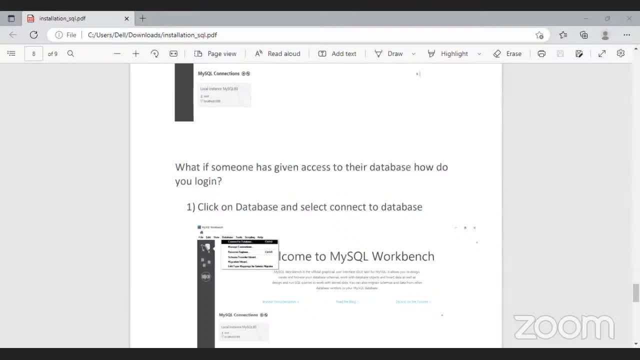 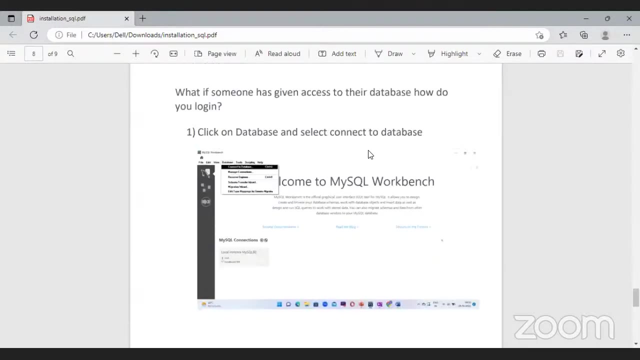 where you find this pdf, like whatever i'm showing right now, that is, which has installation things and also i have given username, password and also the local host. so when you want to connect to that company's database or just you have to do a like. initially you will see a page like this once you. 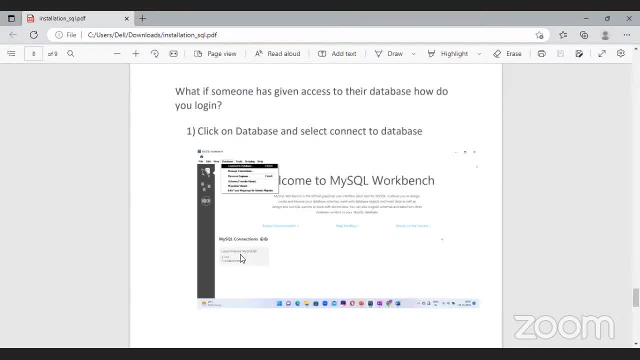 install things. okay, like, if you are using local host, then you have to click on this local. you can see local instance. if you click on that, you have to use the username and the password that you have created. it okay, because that will be an instance for you which is created by you and you. 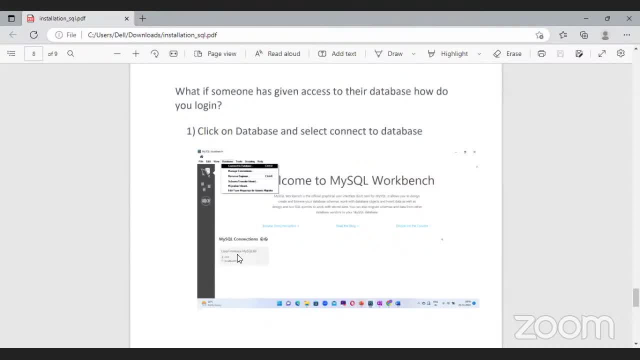 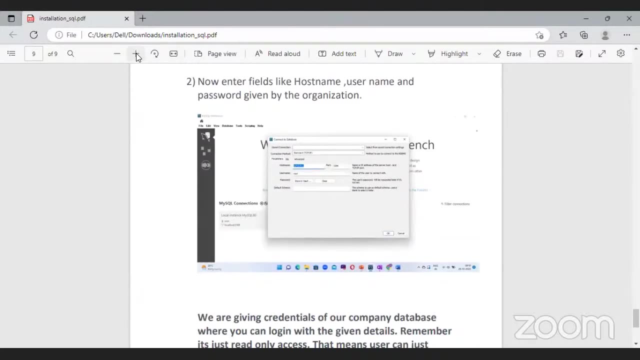 can do things there if you want to join with, if you want to connect with a company or some other database, just go to this database and here you can see the first option, that is, connect to database. click on that. you will get something like this: let me zoom it out, can you see? it's basically. 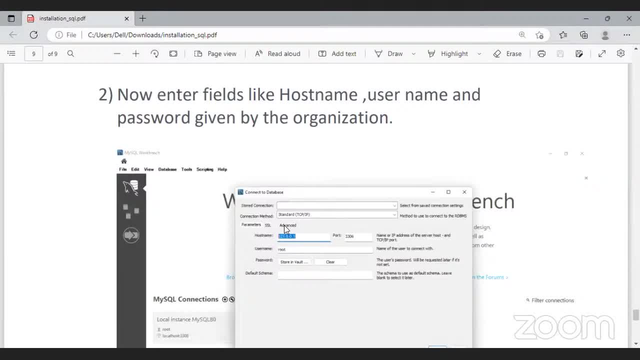 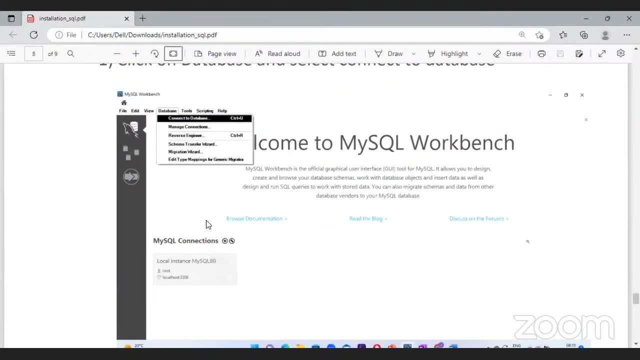 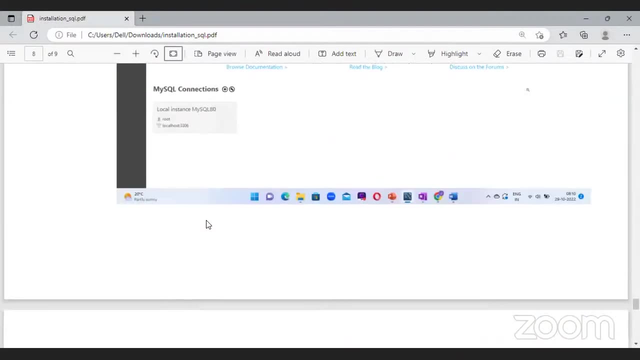 asking you for host name, username and password. so you need to enter it. like, once you do the installation part, you will get a screen, something like this, let me repeat it again: and and you have to click on database, where you get a first option like connect to database, and just click on that and it will take you to something like this, a new. 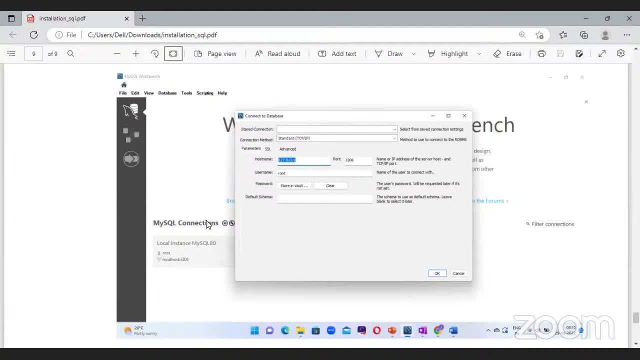 window will be created where you have to paste that host name. remember, don't copy that host link. instead of that, just select the entire text and paste it. if you copy link address and if you paste it here, it will not work. remember that. so select the text and then paste it here in the place of host name, and make sure no. 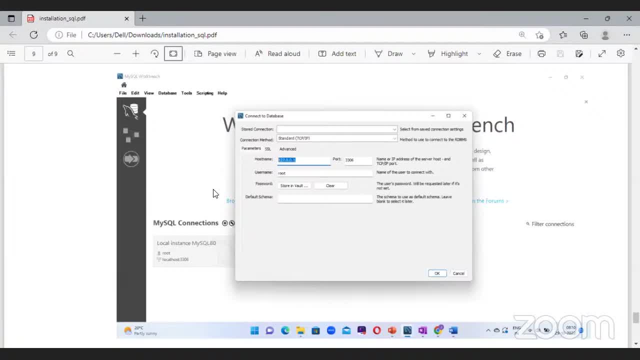 spaces before or or in between that link. okay, so whatever link i have given host name, same thing has to be copied. copy the text, not a link address. copy the text and paste it on host name and username. you can see, even i have given like data mites 3 as something and password you can just type your. 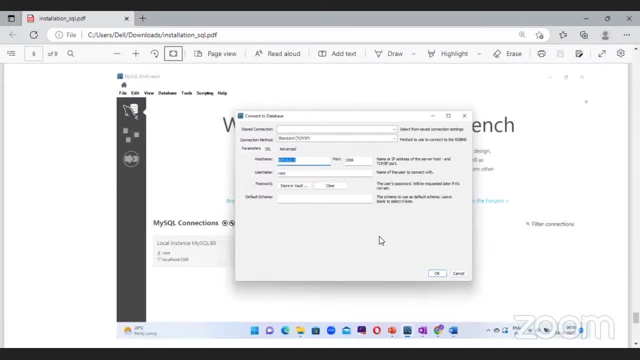 password here and click okay, it will connect you to the company's database where you can see our database name, practice data and also you can see, like: whatever i do, i need to share drive in q and a. okay, yes, i'm sharing it. someone is saying like: why sql when you store data in ms excel? 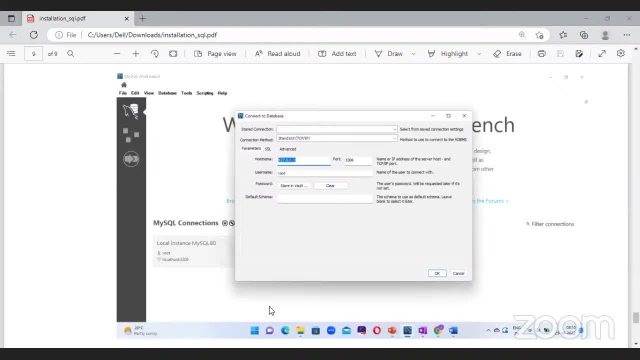 so ms excel, like there is a problem with security, safety and all. so it's kind of advancement, and also you can't share everything but you can't give access to multiple users and also do you do queries in excel? i think it's not possible, so it's basically done using sql. 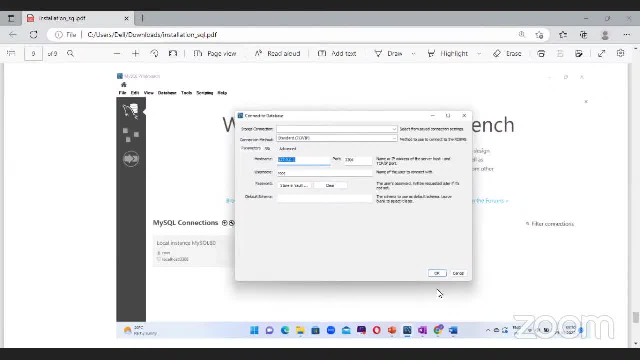 so it's kind of like a. so did you receive the drive link in q and a host team is basically a link. can you see that link? i have given it here. so did you receive the drive link in q and a host team is basically a link. can you see that link? i have given it here. 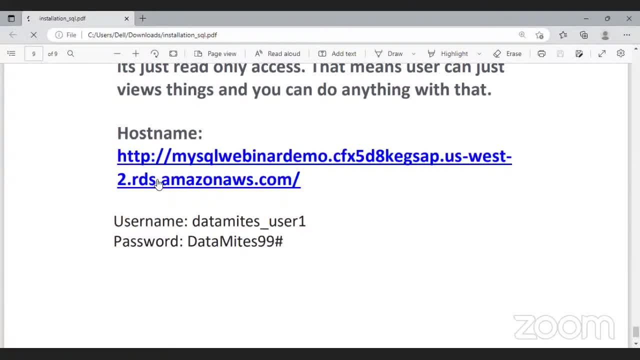 copy this link, okay, oh, you can't cop. you can't copy it in, it's just open, right, can't copy. i need to share a word. then just a minute, let me share word, word document. then all right, shall i share it in chat, only for just now. i'll share it in chat and i'll just upload that word document and, yeah, i'll send it. 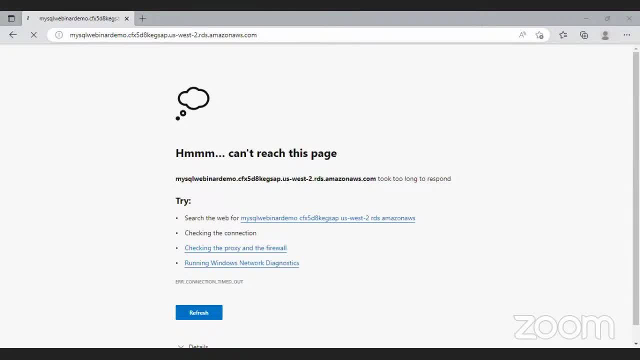 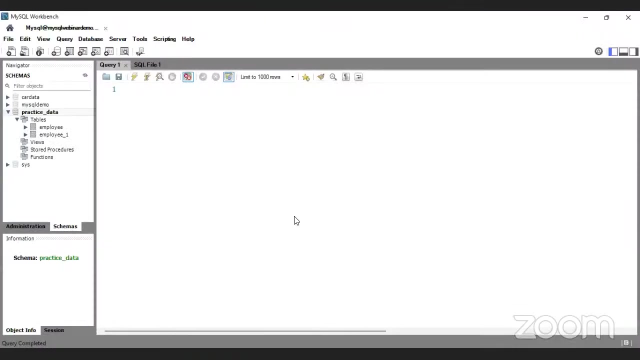 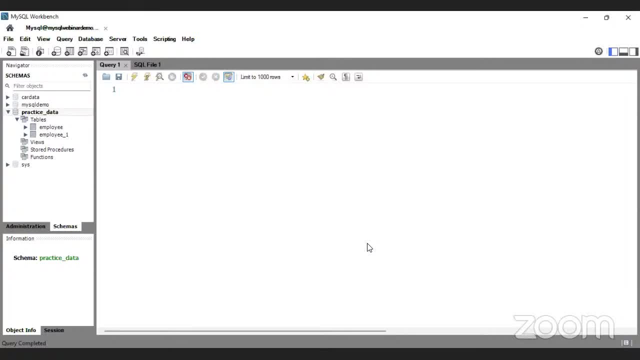 it later and you can just practice it. okay, just listen to the things like how it works. so this is basically your mysql workbench, okay, where you can do, where you can create database, where you can create table. it's not taking the password, why, or is she make sure when you enter that host name, don't? 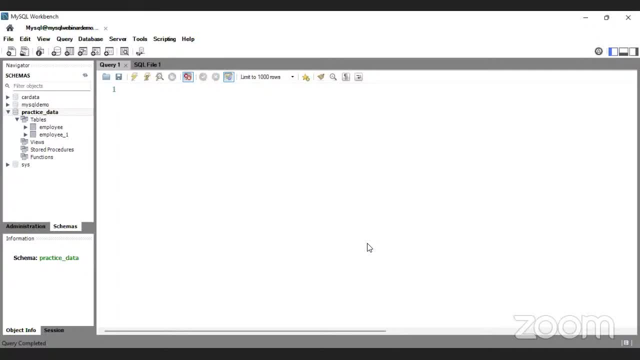 copy that link. copy the entire text like normal copy thing and make sure you don't have slash after that. com dot com and those who have- yeah, those who were able to log in with the given credential. you can see something like this and you can see practice data there. you can see only one data, or because the access 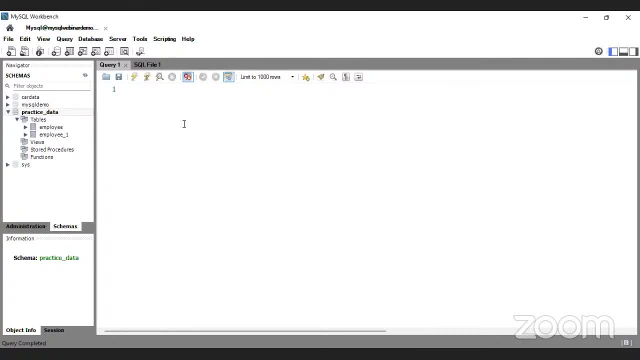 is given only for that. we have restricted it just for one database, okay, okay, let's begin the session now again. so this is a38. started my sql workbench where you can write query. you can see here, um, because this is a schemas where you will see all databases. 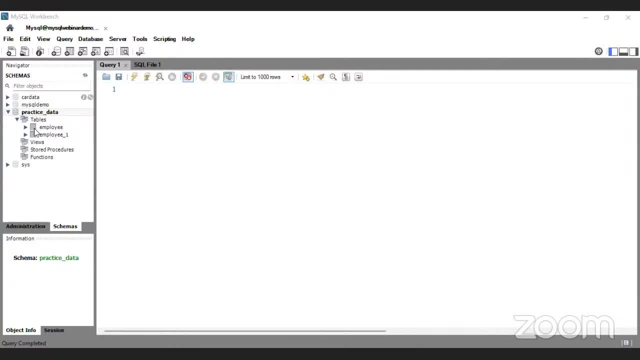 tables, waves, stored procedures, functions. so we'll be focusing only on our database and the tables. okay, so we call this our schemas and you have a file. suppose, if you want to a new query or tab, you just have to click on this new query tab, so it will create a new page for you. 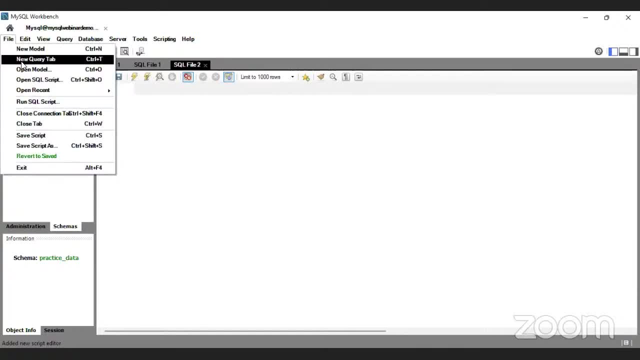 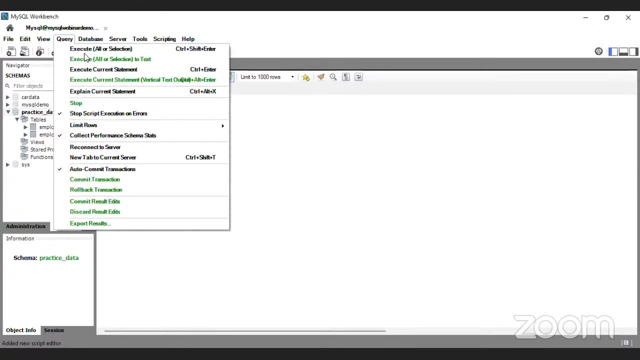 where you can write your query. okay, go to file and you have to click on new query tab. so the next one is edit. it's for cut copy paste thing, and also you can find a text for selecting that basic one. so view, not required, your query. basically, you can. in order to execute everything, the shortcut is: 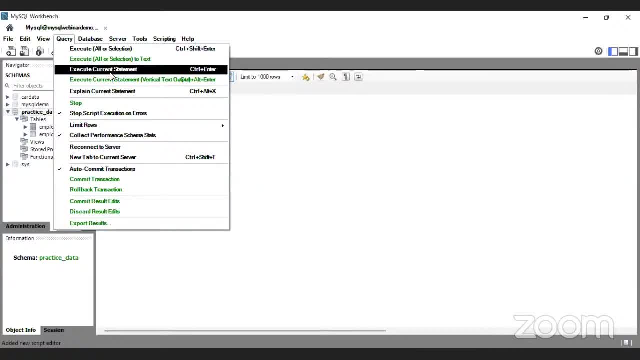 shift, control, shift enter. okay, if you want to execute the current statement, it's just control enter and i think that's sufficient. okay, that is a shortcut. and if you want to do it manually? so this is for executing the selected portion of the script or everything, if there is no. if there, 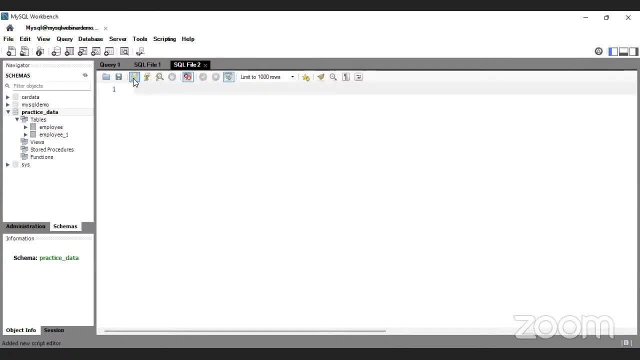 is no selection. that means when you write some program or some queries, it will execute the entire page. when you don't select a specific thing- and this is this- basically execute the statement and then you can execute the entire page. and then you can execute the entire page, and then you can. 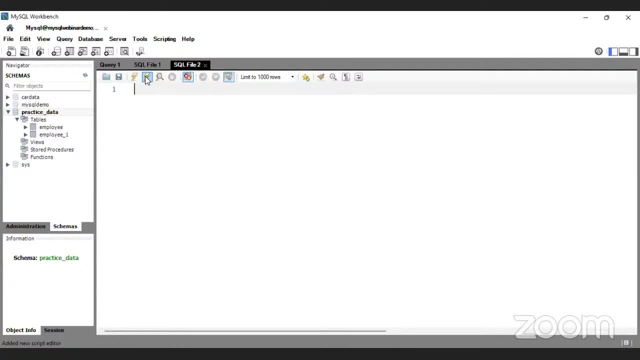 do the keyboard cursor. okay, wherever you have your keyboard. i mean cursor, only that particular line will be executed. okay, make sure you you copy that host host name text. don't copy the link. copy that entire text and paste it in the host name. that might be the issue. 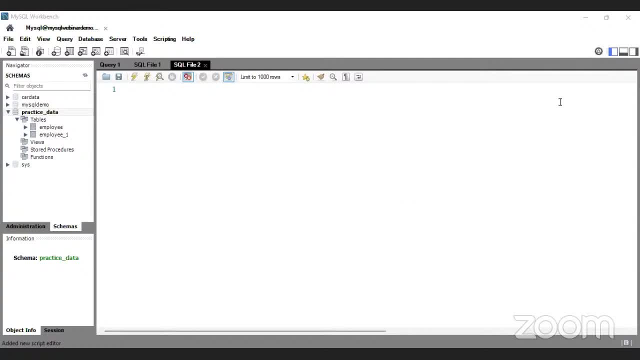 yeah, so understood. so this: basically, if you click on this, it will execute the query for that entire page, and this is just for a selected line. that means wherever you have a cursor, that particular query will be executed, and and also you can limit number of rules, like 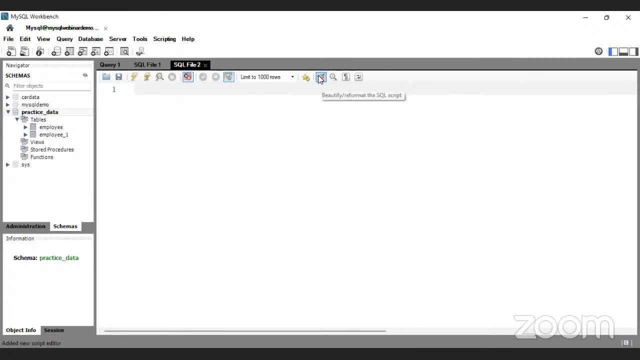 whatever, like how many numbers you want to fetch, and then yeah, that's it. if you know so much, that is sufficient. and also, here you have a different things like if you want just the right side, that is, navigator and the screen you can click on this, okay, it gives you navigator and the sql editor thing, okay. and if you want to see a terminal. 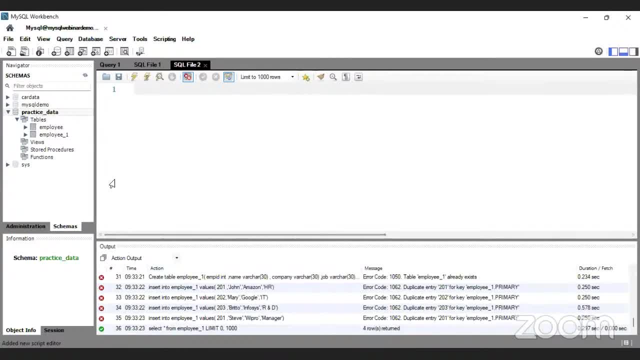 like, like output panel. so it basically gives something like this: you'll get one more thing in the terminal here where you will find your data table. like when you execute a query, you will see your data table and your even you can select this- where you can see like: 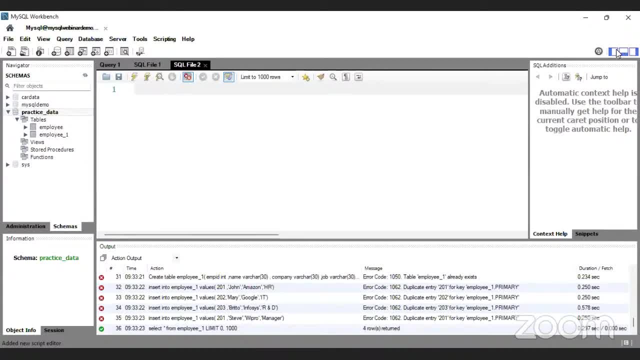 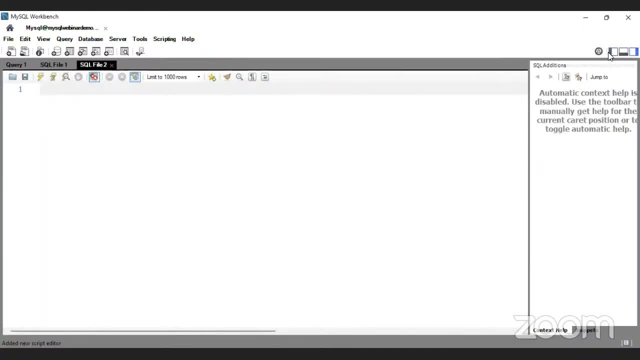 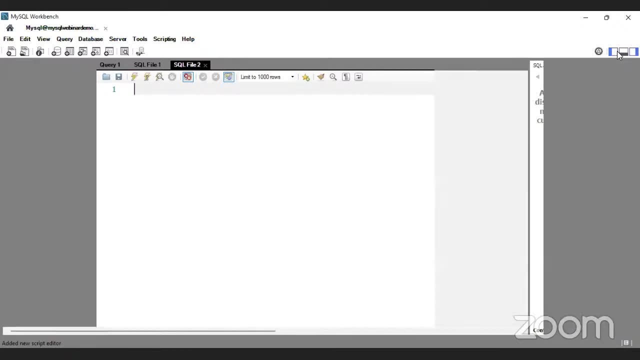 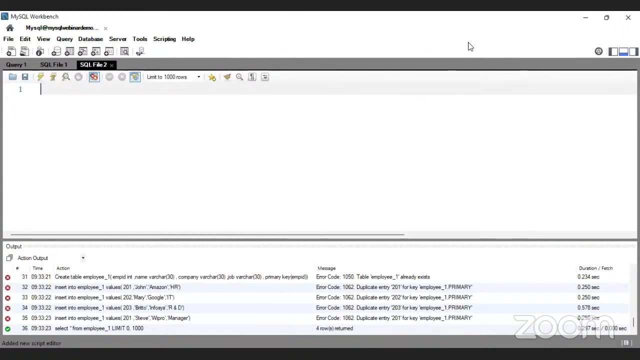 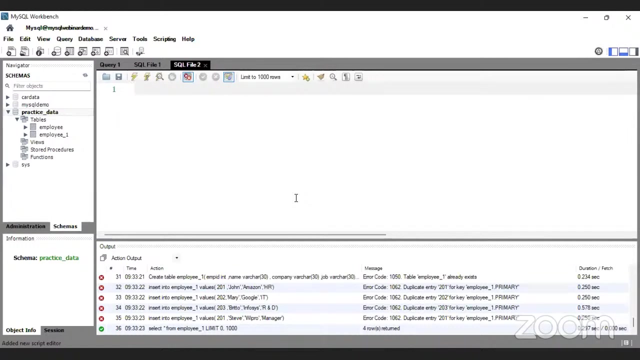 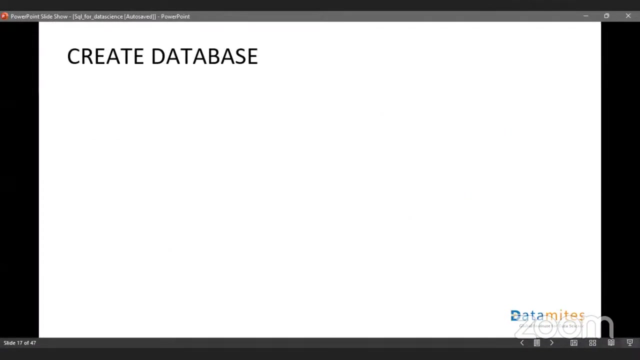 sql additions, like something will be there here, so that's not required for us. so our focus is only on this. okay, so let's see like how to create a database, shall we? can you see a powerpoint sharing? so let me show, like how to create a database. so we study. 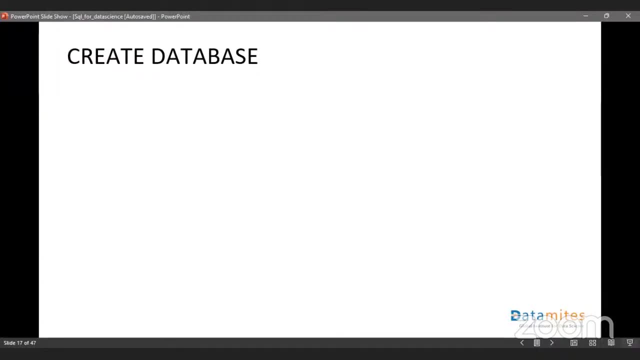 things like: what is database, what is data model, idbms, mysql database and also sql language. so now we are at all so right time and the right right thing. like we are basically into sql, now we are jumping into a sql, so from now onwards, we'll be just focusing on queries like how- how we interact. 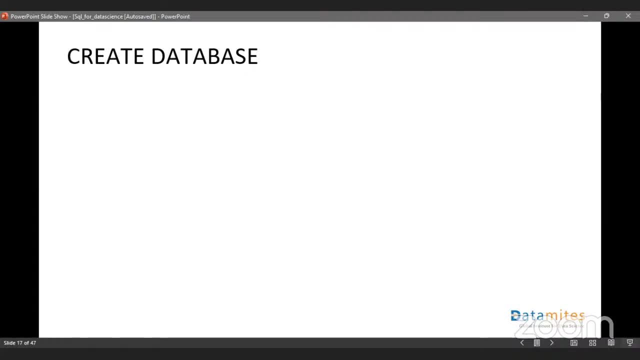 with the database using sql language. okay, the first thing, very basic thing, you need to learn how to create a database. so we have a general syntax. that is, you have to write a keyword as create database. i think you can see that in a bold letters. so that is a standard word. that is, create database, general word and whatever. 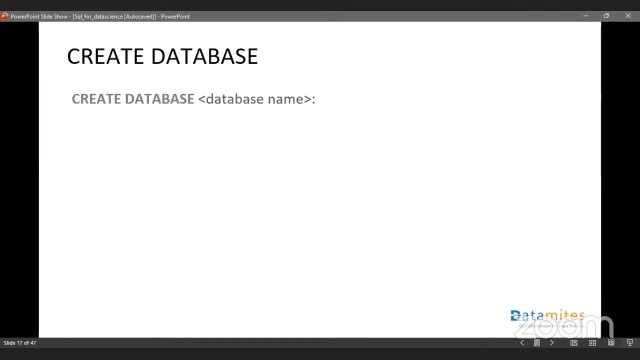 you have it within. you know less than and greater than that keyword. that is basically a database name which can be changed. let's say, for example, i want to create a database name as i want to create a database with name- employee details. so you just have to use a. 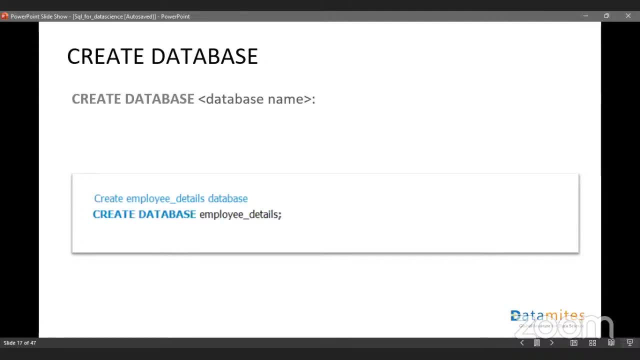 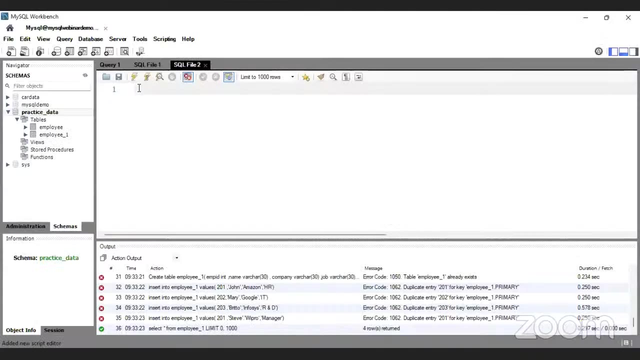 keyword: create database. they are the fixed ones, okay, and you have to write a database name which is employee details. okay, shall we do this? okay, so let's go ahead and let's do that. so let me go back to the mysql workbench. so it's here. i'm showing you how to create. 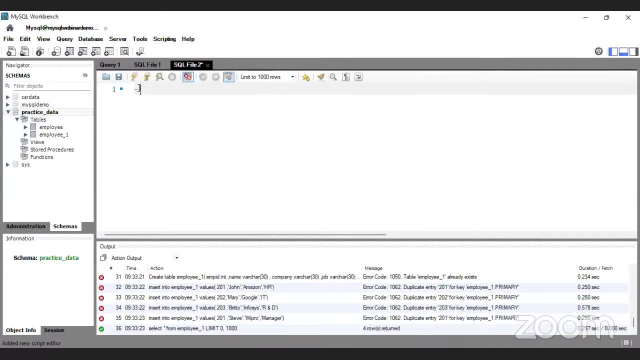 database and how do you comment it? like, if i want to, you might have learned about commenting right, like, if you want to give a description, like what you are doing, so you can just use two iphones. that is a shortcut for comments. so so we are trying to create a database, what? 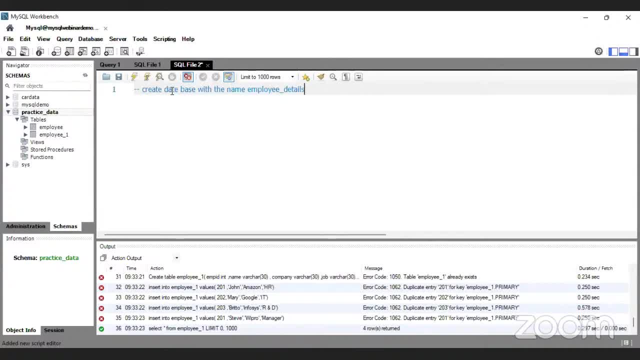 is a database name. so i want to create a database. so how do you create it? you know the syntax, right? so what is the general syntax for creating database? let's create. it doesn't mean that you have to give a capital, only it's a case. it's not case sensitive. so you: 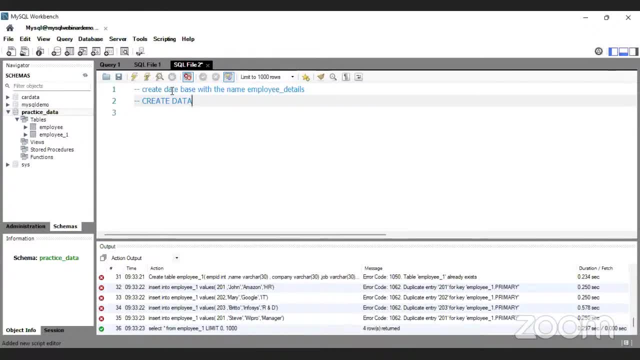 can use. you can use, uh, either a small letter or a capital letter. it's left to you. all, right, so? so this is basically a general syntax to create a database. let's just create database and we need to specify your database name. okay, this is basically a general syntax. now let me show you the actual one. now let's create. 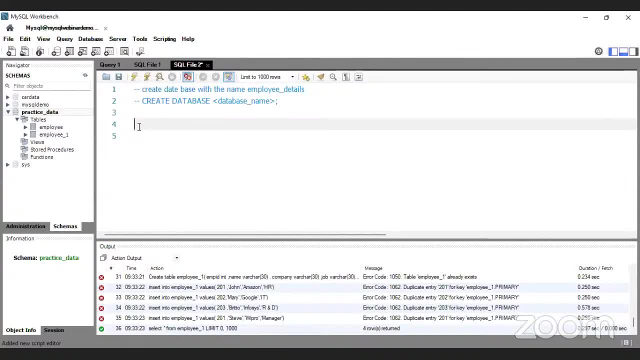 our database okay. so, yeah, let's create it. so create database and i need to specify the database name. so i have given a question like you need to create a database name, okay, so i have given a query, a database with employee details, so let me take it as employee underscore. it's going to be details. 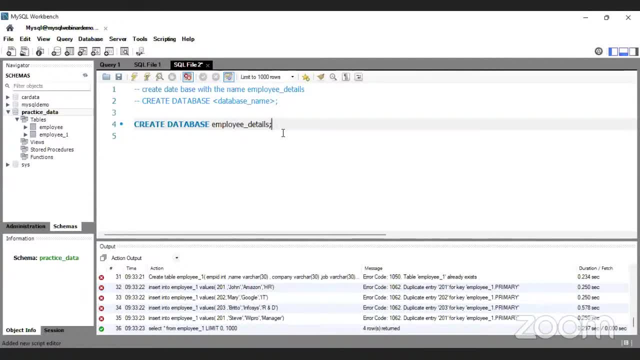 and let's close it with semicolon. it's not mandatory, but still let's go to close it with semicolon whenever you use multiple statements. okay, so what i'm doing? i'm creating a database with a name- employee details you can see here, so you have a database, just like car data, mysql. 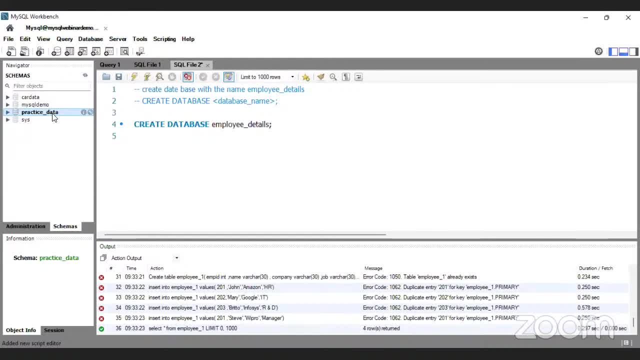 demo practice data answers the people who log in with a credential that i've given. you can see. i think you can see just practice data. yes, so we have restricted you to just that practice data. that's why showing you just that database name, okay, so basically, here i'm trying to create a 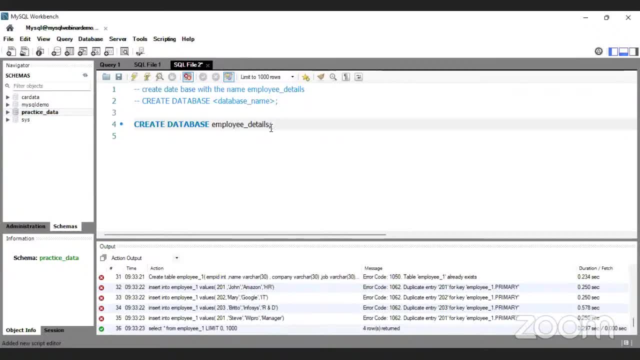 database. create database is a keyword and i have given our database name as employee details. let's run this. so there are two ways. you can use either this or this. so this basically execute the statement under the key cursor: keyboard cursor. okay, let me run this so can you see, in the bottom it sees like create database. 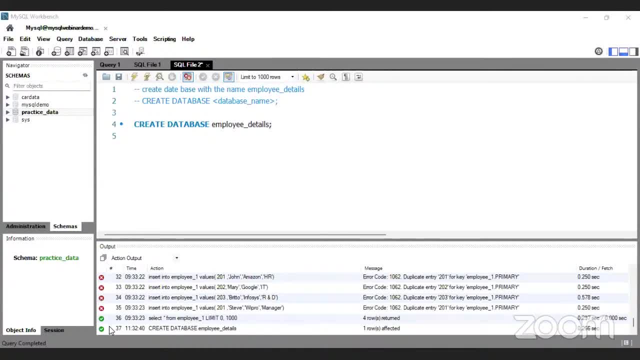 if it's in a green color right mark, it sees like no error or no mistake in your code. if it gives like into mark, like in a red color, it sees like there is some error that needs to be sorted out. okay, so create database and i have specified a database. 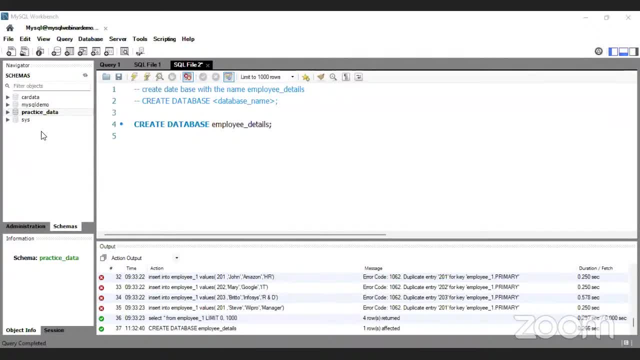 name, but, but still, i can see just four databases. so what you have to do? very simple: you have to refresh it. in order to refresh, just click on this. you can see an option here: a pyro and a down arrow. if you click on that, it will create a new database for you. can you see employee details? curators? yes, 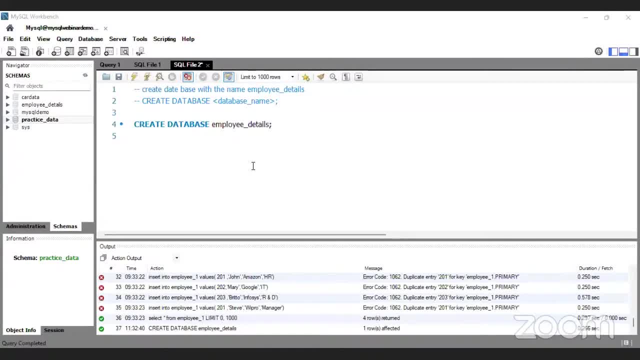 so now you can see it is a very simple database for you to use. so if we take this and you want to create a database, a database name, we have to make it so that it will be sorted through your data data. the first step is now: if you want to create a database, you just go to. 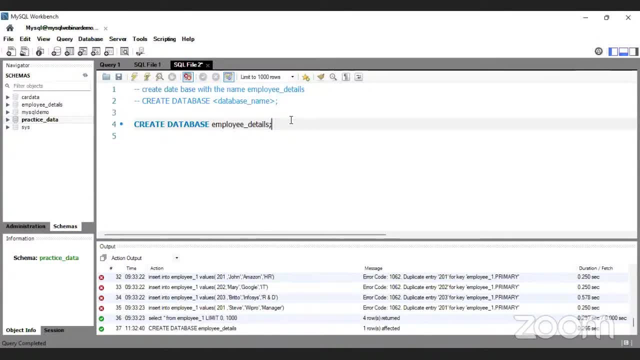 the database category and that's where you have to go to create a database and then go to your database. wise, that is where you have to go to to create a database, and i'm gonna do it in a few slides here. so just see that we've created the database name and then create the database and 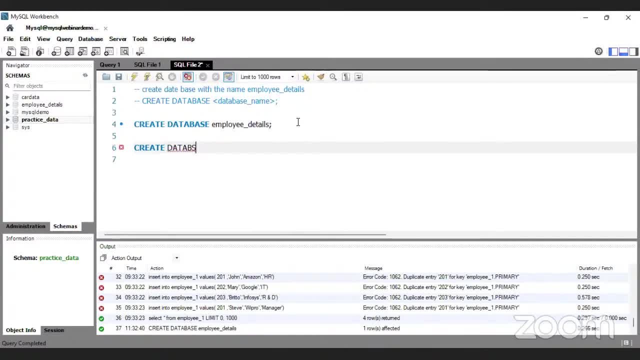 So create database? Yes, Devashush. basically the access is given only for the practice data, like whatever databases I'm creating. that you can't see that, Okay, only the database creation will not be seen. rest of the things will be seen there, Okay. 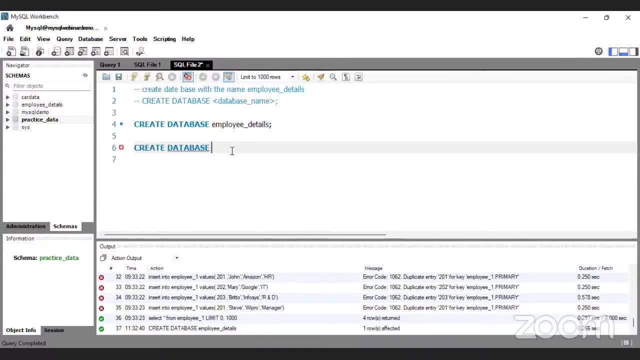 Yeah, these queries will work in online SQL compilers. you can just try with that as well. So let's create one more database with a name, Let me say student, Let me say student details. So you will create a keyword as the create database and choose the name. 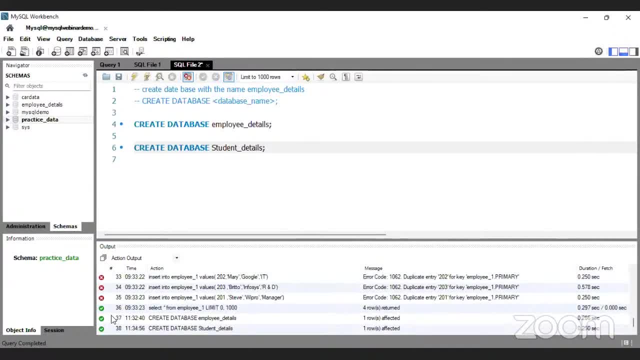 And let's run this. So it gave a green color. what that means: the query is executed And in order to see that database, you just need to refresh it So you can see Student details here. So this is how you create database. you know my SQL workbench. 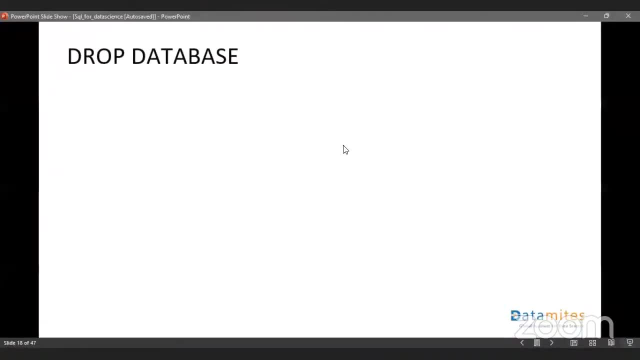 So now let's move on to the next slide. So this is how you create a database. Now do you want to drop a database? you can also drop, but you can't change the name. So whatever database you have created, that can also be dropped. that can be removed completely. 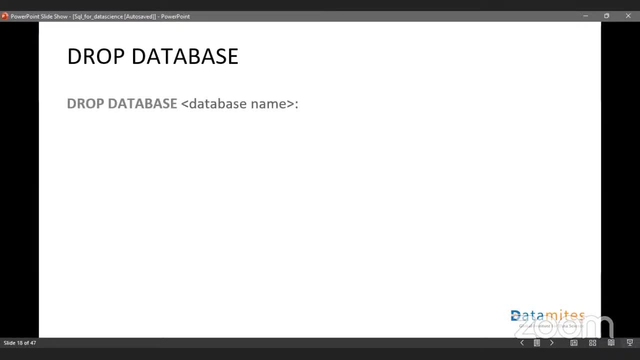 So it's just a drop database. that is a keyword and you just need to specify your database name. So here is an example. So we have created employee details table And now let's just drop it. Let's just drop the employee details. Okay, let's do that. 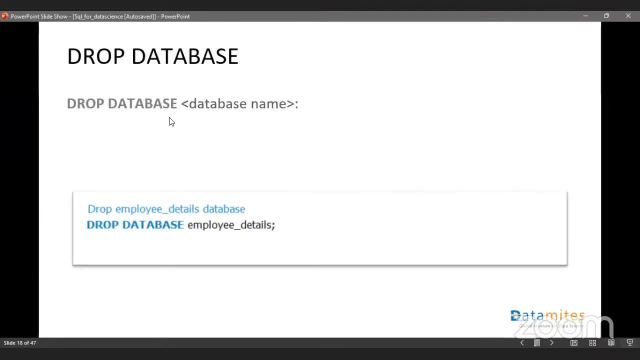 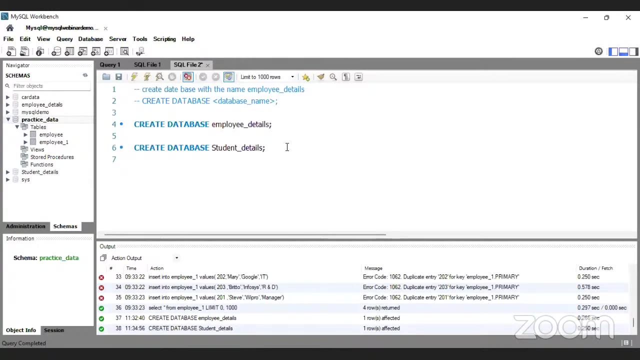 Drop database is a keyword and you just need to specify the database name. Let me move on to my SQL workbench. Just understand, like, how keywords are working. Okay, don't worry if things are not working, focus here. So I need to drop, so it's drop database. 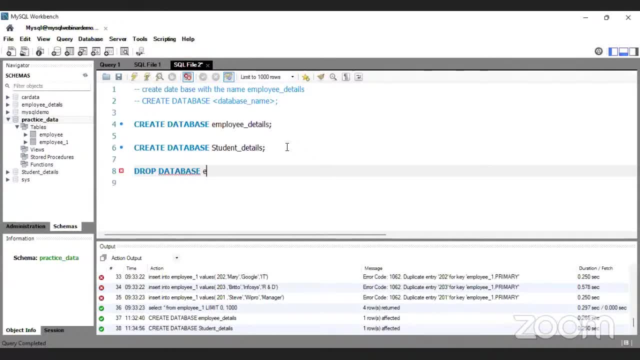 Drop. database is a keyword and you just need to specify the database name versus. I'm basically trying to remove. you can remove employee details. I'll remove our student details. Okay, so let's see, I'll remove student details. Yeah, So here you use a same thing. like whatever you you have created, database name should be seen, Otherwise it just gives you an error. 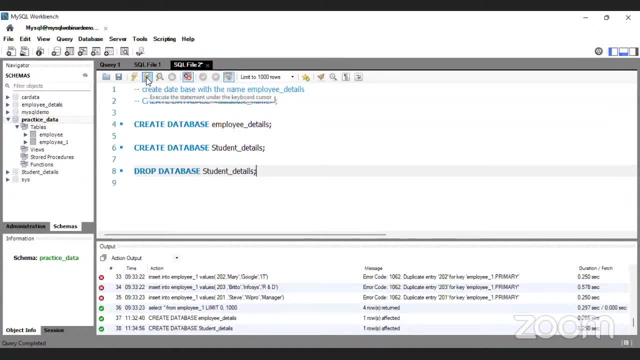 So let me run this and let's see whether it works or not. Basically, we are trying to remove the database. If we run this And let me refresh So you can see there is no database here. There is no student details database. It's removed. 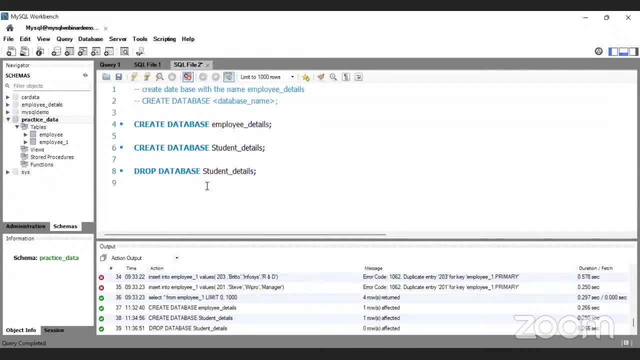 So for creating: let's create database. Database name. for dropping: Let's drop database and database name Done. Truncate basically removes all the records from the table. Drop will remove the entire database. Truncate comes on the table, So this is how you drop. The next one is: do you want to see all the existing databases? 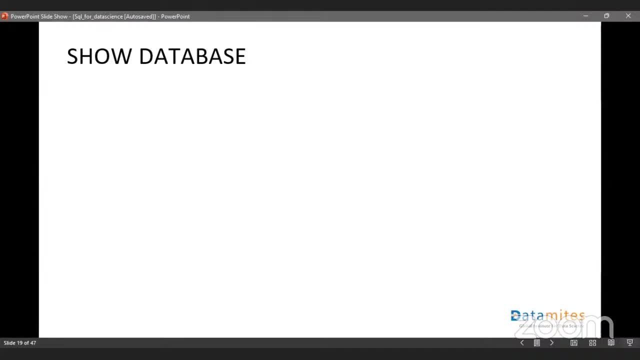 That you have it in a MySQL workbench. It's very simple. You just have to take a keyword, show databases, which is going to rate it- all the databases that are available in MySQL. Okay, So you can just write a code as show databases. 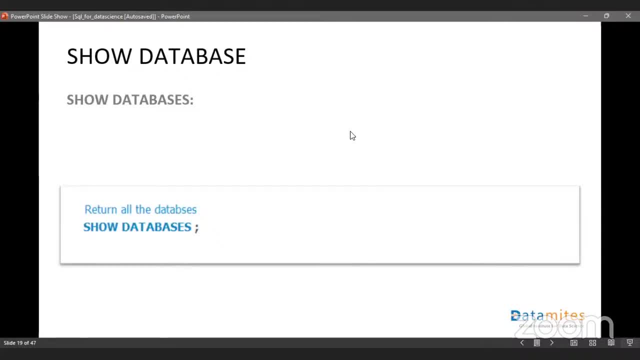 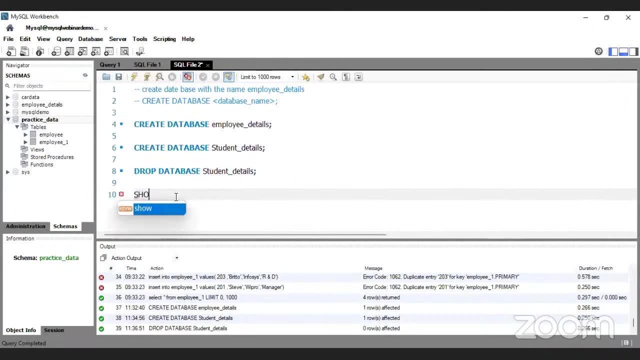 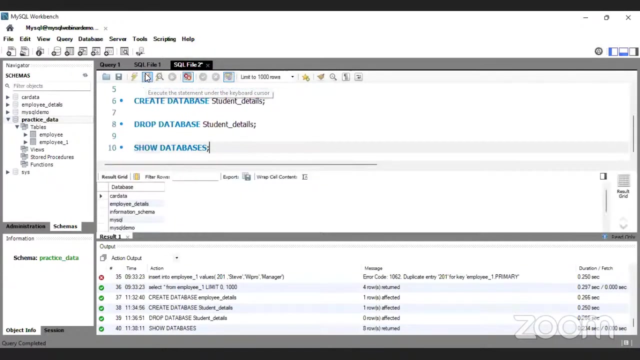 This will be a query in order to see all the existing databases in a MySQL workbench. So let's print. It's going to be show databases. So it's show Databases. Let's run this. Yes, it's going to fetch. 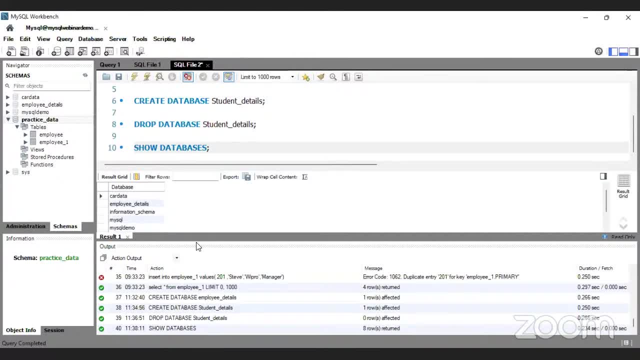 It's going to retain you all the databases that are available in MySQL workbench. Can you see? So it's car data, employee details, information, schema, MySQL, MySQL demo. Okay, And there is no student details because we have dropped it. 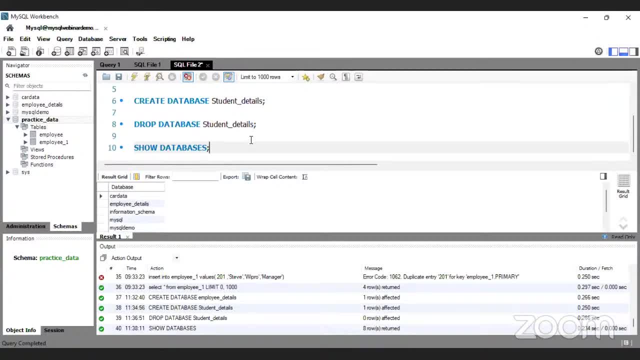 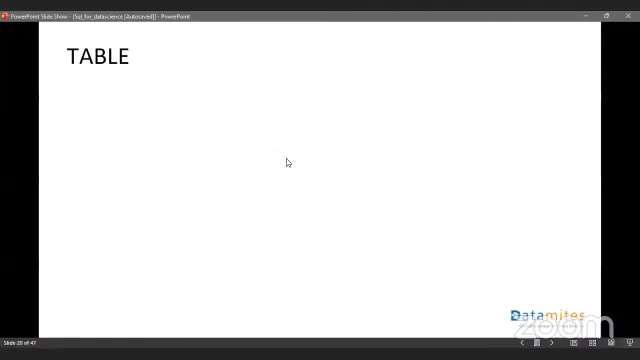 Getting things. Let me move on to the next one. So, done with showing databases. Now let's move on to the table: Table creation. So what is table? So SQL table is basically a collection of data Which is organized in rows and columns. 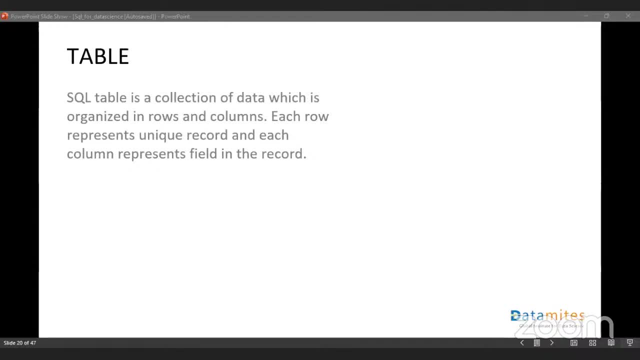 Because we are dealing with a relational model. That means, obviously, data has to be in a table. So this basically gives you an explanation of table. Each row basically uniquely represents a record and each column is represented as fields. Okay, Or else you can call it as attributes as well. 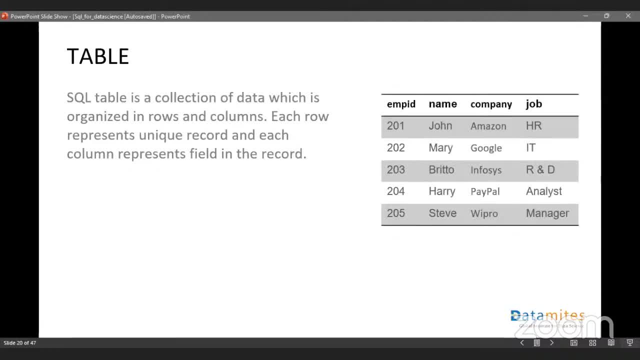 And here is a table: Employee ID, name, company, job. This table basically gives you an information related to an employee, Like employee ID, employee name, company and what they are working And also the designation, So you can see. 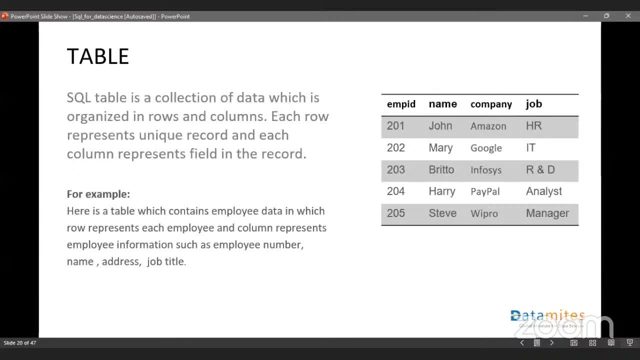 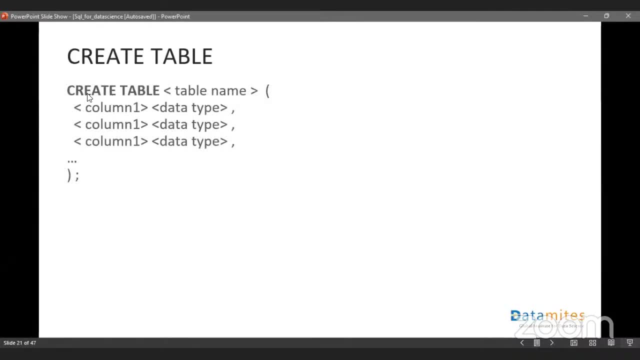 Okay, This is basically a table, which is in the form of rows and columns. Now we need to create a table. How do you create a table? So, in order to create a table, first you have to specify your keyword as create table. 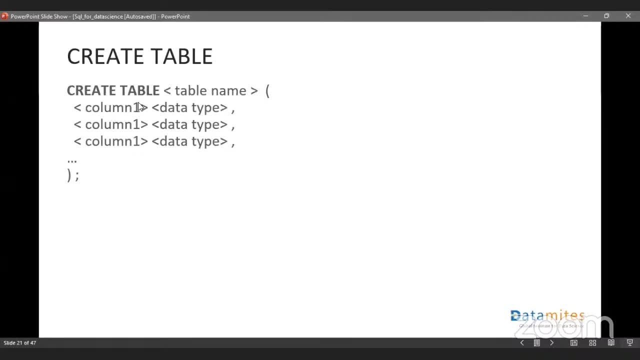 And then you need to specify a table name And then column name. Along with that column name You just need to specify the data type that particular column is taking. Similarly, you can try with column two, column three and so on, And you can see an example here. 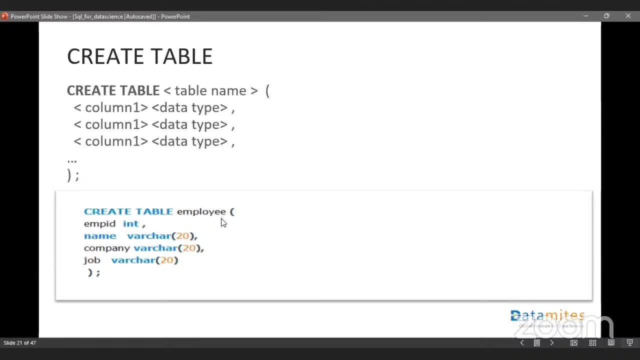 Create a table employee. Basically let's try to create an employee table with a column name such as employee ID, Employee ID is numbers, So obviously the data type has to be in teacher And name is a string kind or a character. So you have to take worker and company. 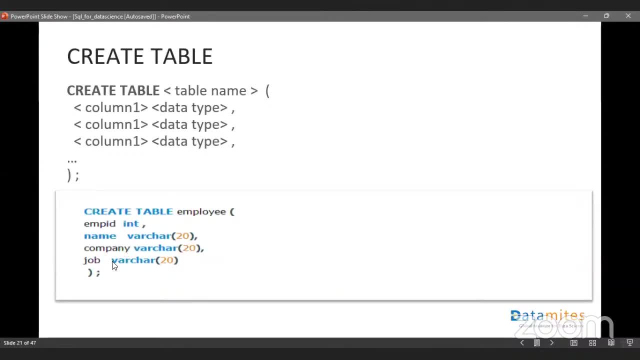 Even that is a text kind of data, So it has to be worker and job is also worker. That means variable characters. So before creating a table, let's see what are the different data types And let's come back to this: create table. 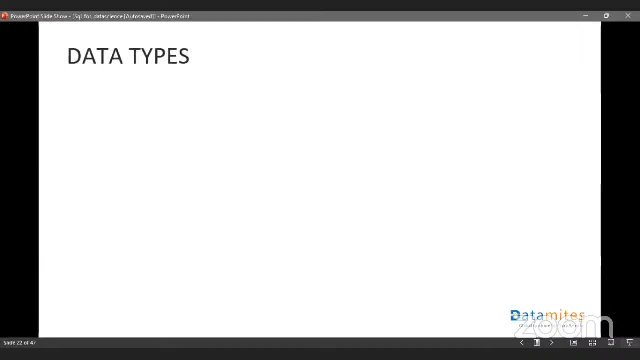 All right, Yeah, So we have different data types, right? You might have studied these data types in your Python as well. So data type of a column basically defines, like what sort of data an object can store, Such as a data can be in teacher. 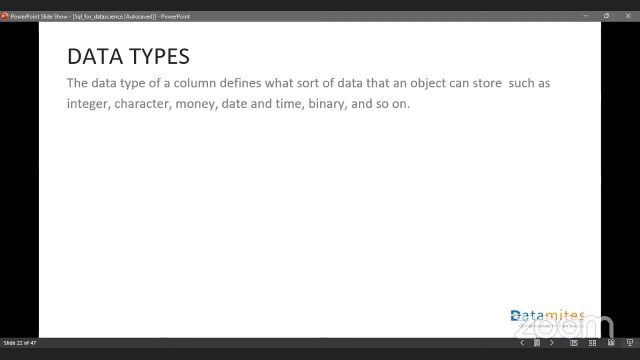 It can be character, It can be money, It can be data in time, It can also be binary and so on. Yes, Data types can be of different types. It can be numeric, where you see teachers float and data, character, Character, in the sense it's a string data or a text kind of data. 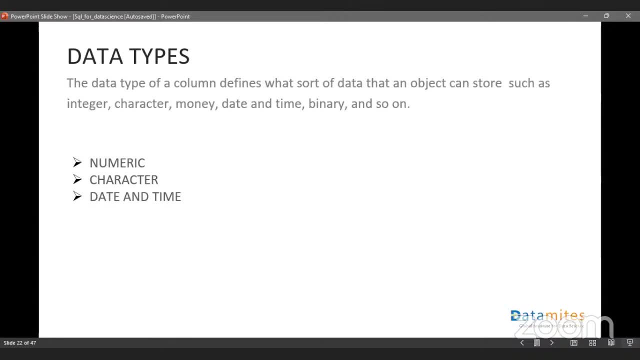 And then it's data in time. So you know probably when you deal with, when you take a data set So it might contain data in time kind of data as well. Like if you take a superstore sales it will mention like order. 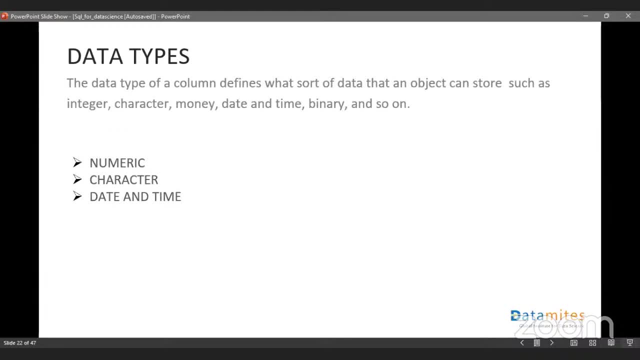 Date, shipping date, everything. So, in order to deal with data type, So we have these data types, So these are the basic and major data types that will be seen in SQL. Yeah, So numeric means So we have a different data types in numeric, like big integer which takes a range, like 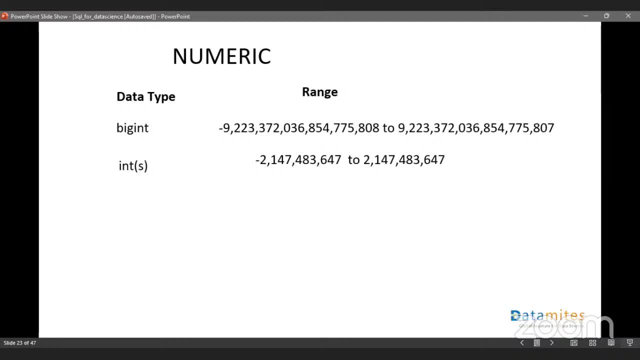 minus nine. It's very hard to count, but I can see it. And then you can just imagine it in 10 powers and integer- It's a small word like S- basically stands for size. It takes values from Two, one, four, seven, four, eight, three, six, four, seven, two. 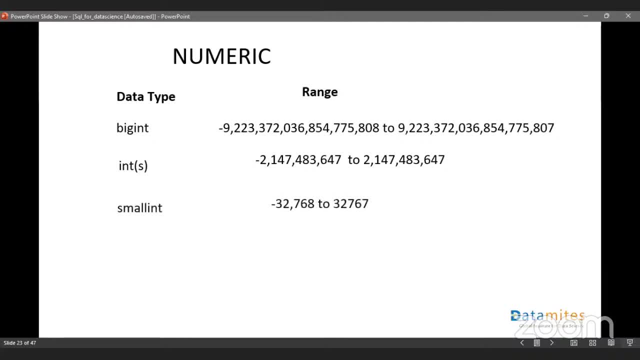 That's a certain range for a teacher And for small integer it's just like minus 32,000, seven 60 to 32,000, seven 67, 67 bites. This is a range, Range of bites that it's taking. 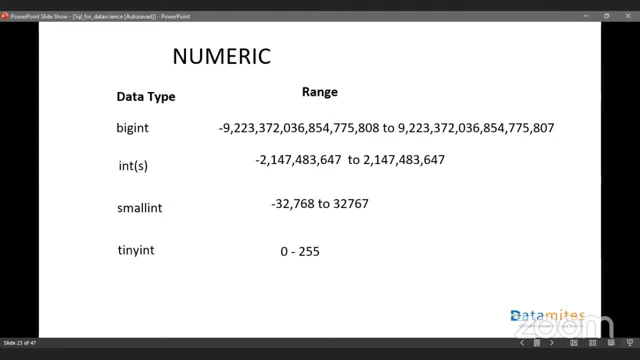 It's taking. Okay, Tiny integer meets. It just takes values like zero to two, 55. And if it's a float, you can specify. you can use a data type as a decimal and you can specify your size Size, Okay. 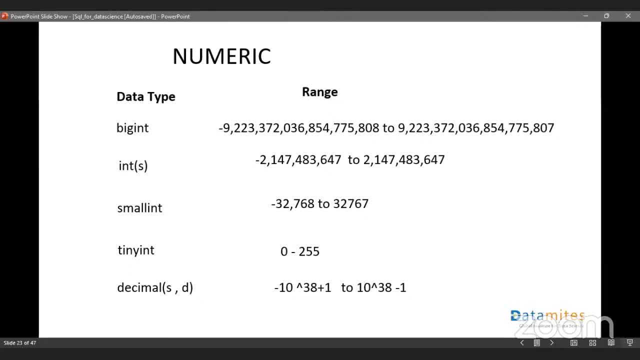 If it's zero to 25, like whatever size you want. If you want the 30, 30 bites, you can see 30 comma. You can specify the number of decimal points. These stands for number of decimal points. Okay. 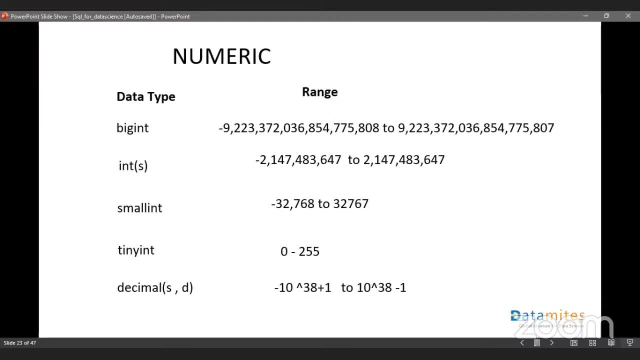 Usually, when it's an integer, we go with INT And we don't specify the size, It's okay. Even if you don't specify, you can just say INT, And when it's a flow, you can go with decimals, Okay. 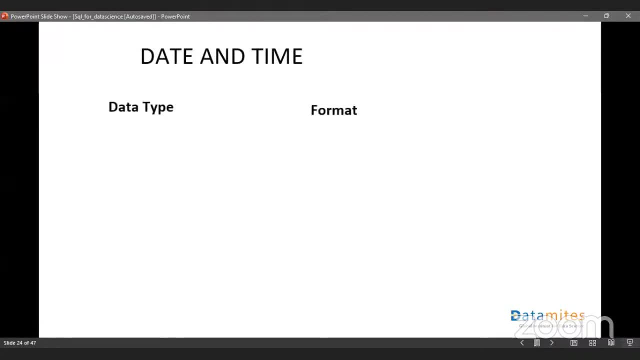 These are the different numeric data types And the next one is date and time, So there are different dates, Like data is. basically it will have a format like first it's an year and then month and then date, So this will be a format for date. 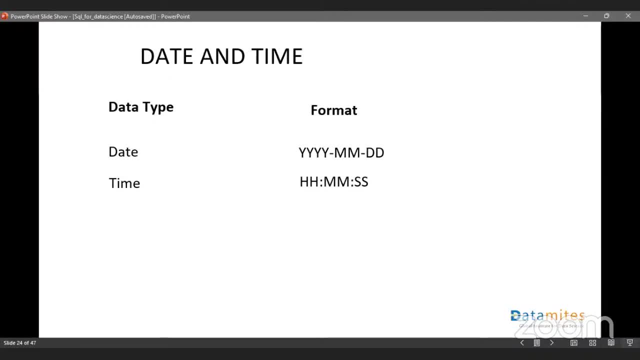 Standard format And for time it's going to be first hour minutes and then seconds, And for year it's going to be y y y. Okay, So this is about date and time, And the next one is character. 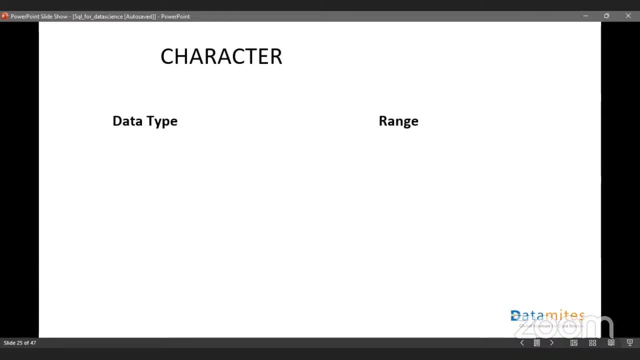 Character means it's a string kind of data, So var. You'll be dealing with that text kind of data. So we have character kind of short form. It's char, Which basically takes characters between 0 to 225.. This is a range. 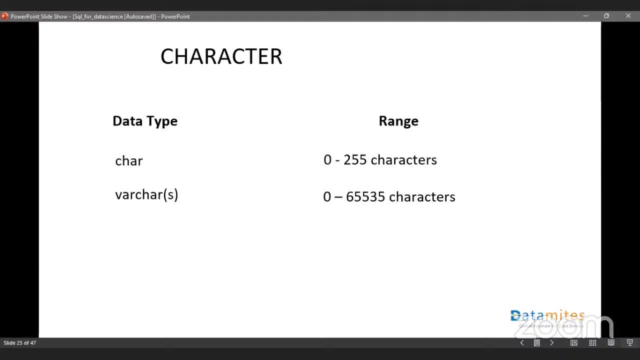 And var char. You can just specify your size there. It takes huge amounts, like 0 to 65,535 characters, And even text it doesn't take a range Like it can include a huge number of characters. So that's how a text works. 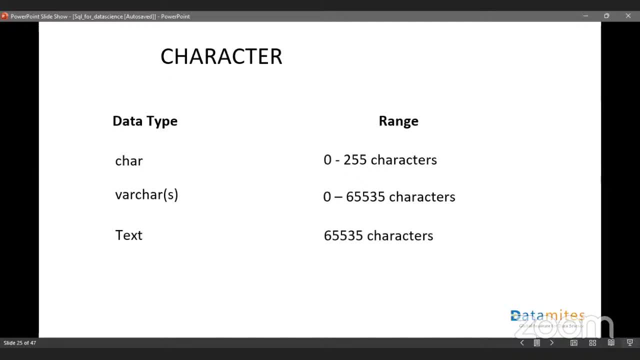 So these are the different characters that we use. Basically we use char for a specific text And for a small text, like for name, company and all, And also you can use var char, So for integers, like, we use int there. 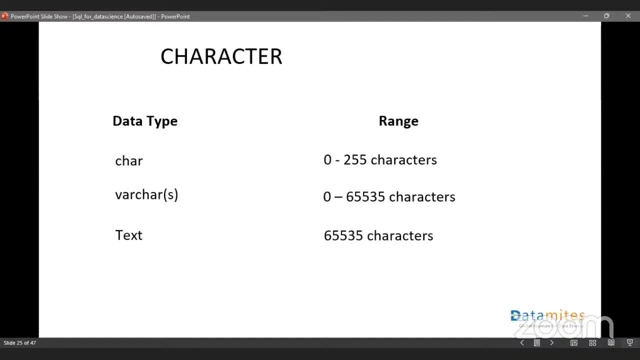 And for character we use var, char, Yep. So these are the different things about data types, And also we have SQL constraints. So what are these constraints? So we call them as DBMS keys. They are basically an attribute which help you in identifying a unique record. 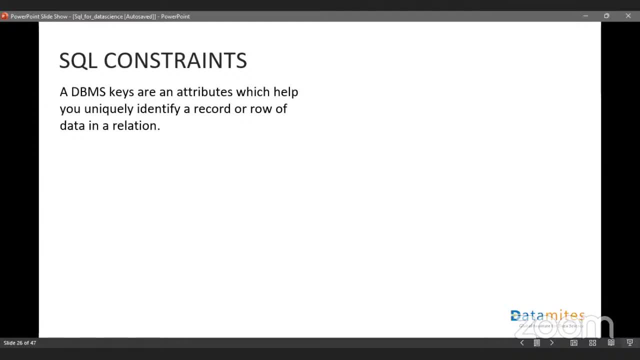 Or a row of data in a relation. So what do you mean by that? I'll come back to that. So we have different keys, like not null, unique primary key, foreign key, check and default. So these are the different SQL constraints. 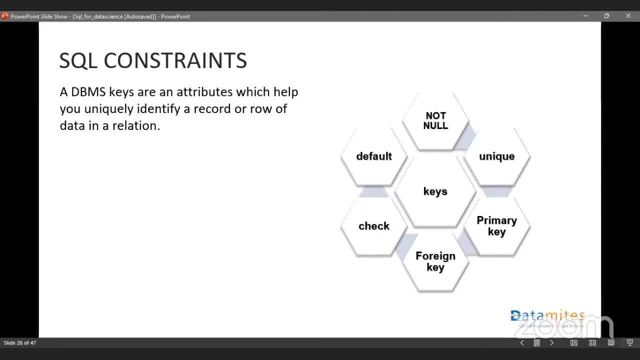 So you can specify these constraints when you create a table, So that these constraints are basically a set of instructions that we are providing for a particular column. So let's see one by one. First let's see the definitions of each one, And then I'll show you how to create it. 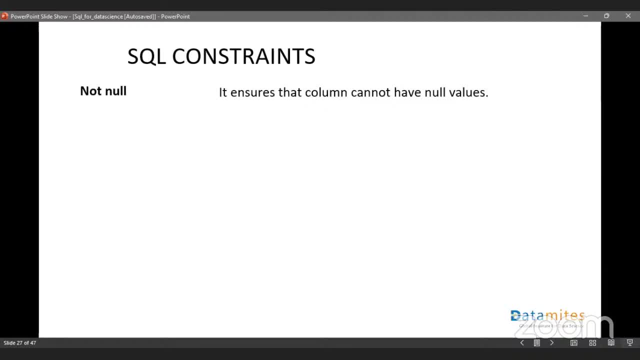 OK, So we are basically speaking about a SQL constraint. So the first SQL constraint is not null. You might have studied about a null concept. When you consider data, data can include empty values. We call them as null values. Yes, So when people start collecting data, so let's say, I'll generate one Google form for you and I'll ask you to fill. 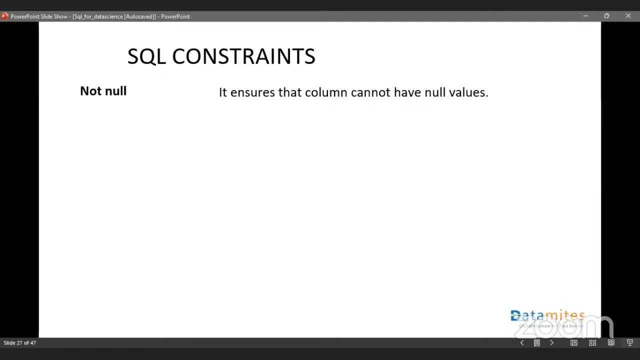 OK, I'll give a different fields, like name, age And also like, yeah, Work experience and your background, like what you have done, what is your graduation and what's your job designation. So I'll create one form for you like this and I'll share it with you. 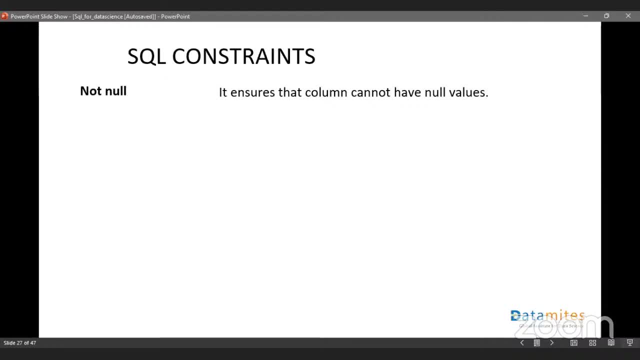 You have to fill that form and you have to submit it to me. So when you fill, when everyone fills that form, I'll get our data. Yes, no, that's how we collect our data. Now the question is, when I create those fields, what I do in the place of name. 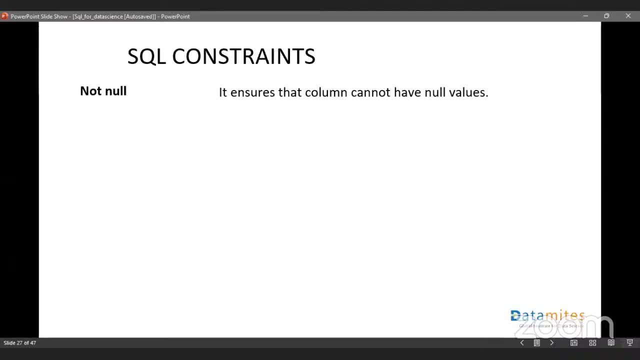 OK, So you'll have a name, phone number, everything What I do, I specify For whatever that column I have created, like phone number, column or phone number, block or entry, for that I specify it as not null. That means when you start entering values, some people, what they do, they don't like to give them phone numbers. 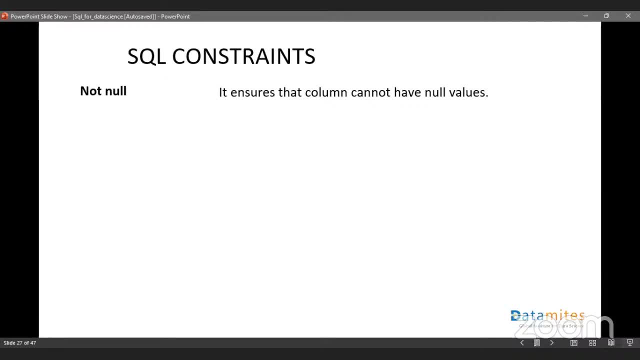 So what they do, they'll just keep that OK When I specify it like not null. if you don't fill that block like phone number block or a phone number cell, it won't accept the form OK When you click on done, it will not consider. 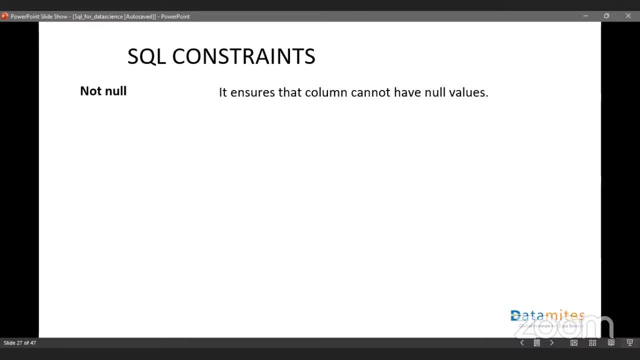 I have specified the condition like not null, And you have to specify some number that you have to either write your phone number or some numbers like, which takes a format. Only then you will be able to upload or you will be able to submit that form. 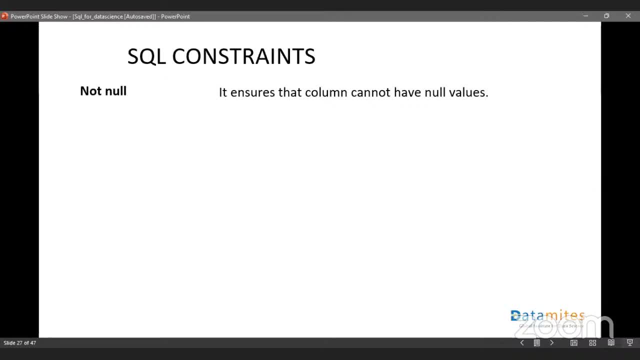 You might have experienced this, but you know, when you log into some websites, like when you look for if you come to a data might itself, like if you come to a data, a data might website And if you want to download some course details or course syllabus, you will get some information. 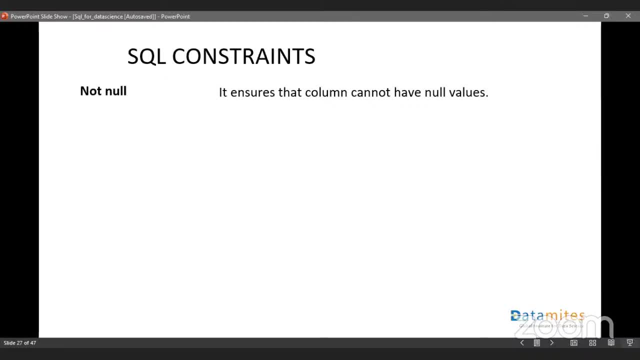 You will get some thing right, Like you will be asked to fill a form. You will get a form like: give you a name, mail ID and the phone number. So if you fill just your name and a mail ID and if you don't fill your form- I mean if you don't fill your phone number- it will not submit and it will not show you the code structure. 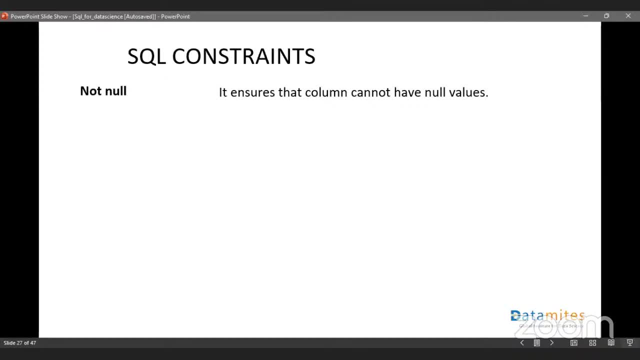 Yes, no, Because someone who has created that form has restricted that condition. They have specified it like not null. Not null means it ensures that column cannot have a number. OK, So you can't leave that column as a blank. If it's not, it will not take. 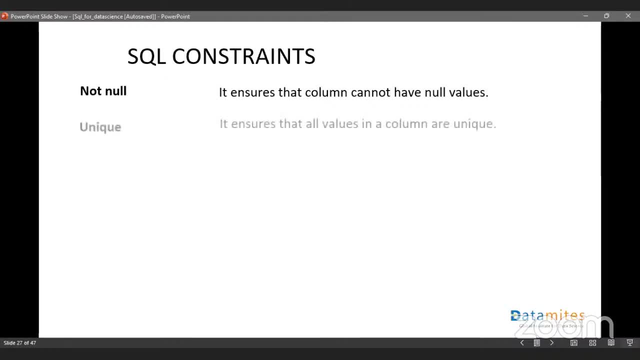 So that's why- that's how you know not null constraint will work Similarly. next one: unique. It ensures that all values in a column are unique. Sometimes IDs can be repeated, So in order to avoid that, we use we use unique constraint and the next one is primary key. 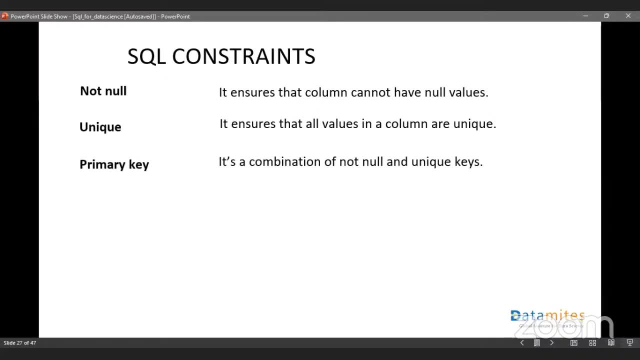 It's just a combination of not null and unique keys, So that means it takes unique values. So, instead of specifying not null And uniqueness for a particular column, what you can do instead of not null and unique, you can just give primary key. 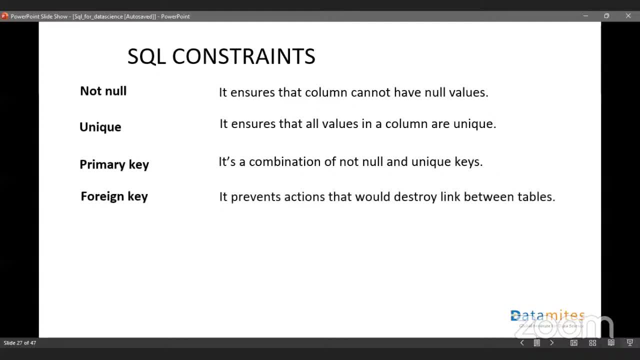 OK, it's a combination of not null and unique keys, So foreign key. it basically prevents actions that would destroy in between tables. So that means this foreign key basically helpful while joining tables. OK, so it prevents, like if someone is joining and if something is happening while joining or while modifying, that could be prevented with this foreign key. 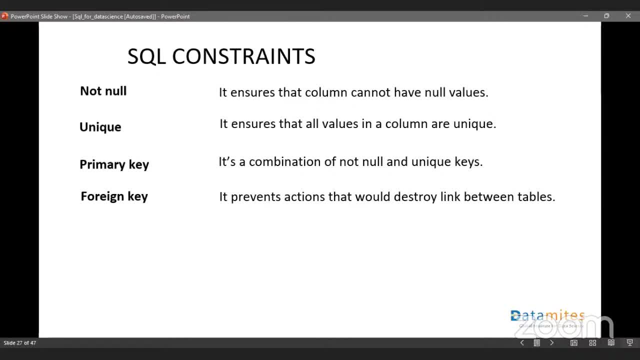 If you specify it as foreign key, It will take care of this, And we have default sets of default value for a column if value is specified. So let's say instead of like: sometimes even you might forget to write things like if it's general or general thing, like, let's see. 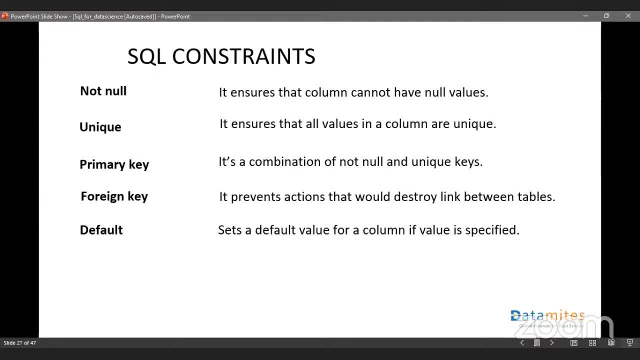 If you are from India. if you are from India, then if data is related to India, what we can do is someone who is collecting information. What he can do is He can just set default value for that particular country as India, Even if you know the person who is filling that form or the place where data is collecting. 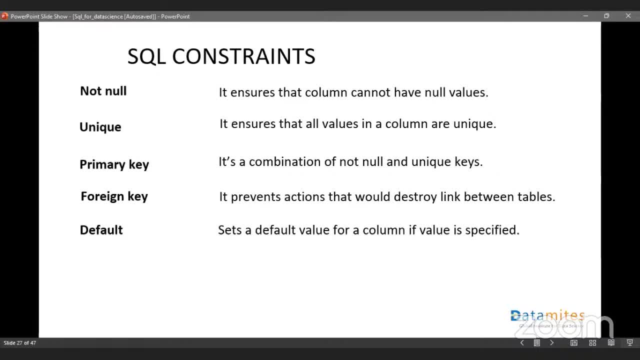 Even if they don't specify the country name by default, it will take it as India. OK, that's how default key is going to work, And check basically ensures that values in a column satisfies the specified condition. So you can specify a condition. 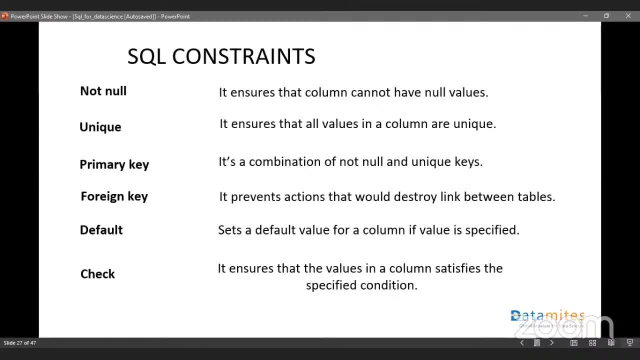 So let's say, like, if you are collecting data related to the people who are less than 30 years, What I can do is I can restrict myself the condition as that age column has to be less than 30. If person is trying to log in that website with the people who are greater, whose age is greater than 30, couldn't log in because we have set a permission or we have set a condition, like it has to collect a field or it has to collect a record only with the people whose age is less than 30. 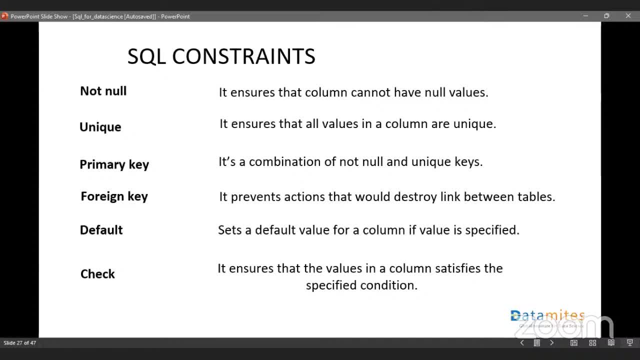 That's how check constraint is going to work. OK, it will ensure that value in a column satisfies the specified condition or not. So these are the different constraints that will be using, So I'm not going in depth about this. So, if you know the knowledge like: why not, why you need, why primary, why foreign default set? 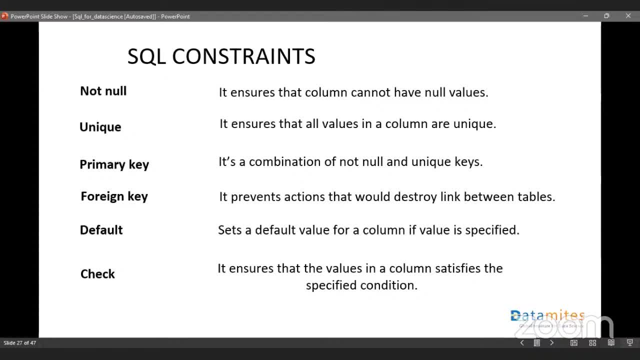 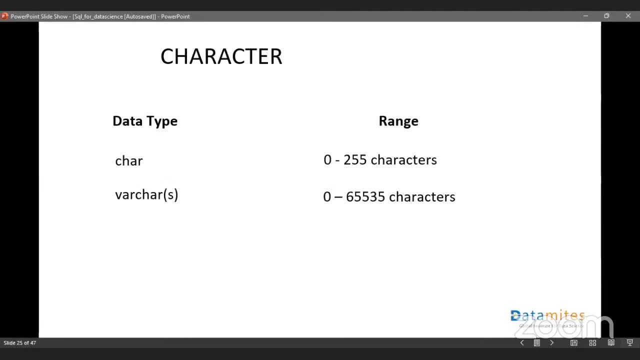 That's more than sufficient. OK, That's what they expect as well. Done Shall. we move on to creating table. Let's go back to this. I need to create this table. Yeah, So I'm basically trying to create a table for this data. 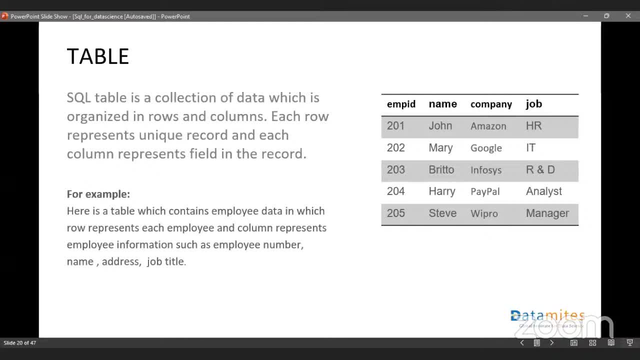 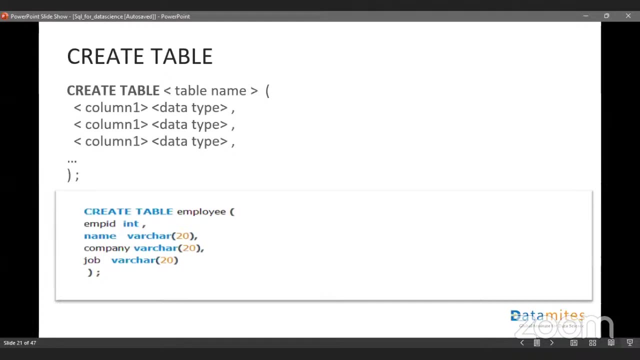 Employee ID name: company: job. So how do you create it? I need to create a table for this. So- and the code is here, Syntax is here- First I need to take a keyword as create table, and then you need to specify table name and then column name. 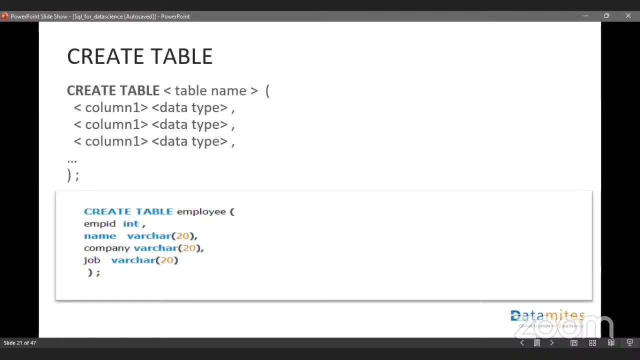 You have to specify data type. If it's required, you can give constraint. Then again second column data type, Then third column data type, fourth column data type, And also you can specify the constraint. OK, Yeah, So let's move on to the MySQL workbench and let's see how to create a table. 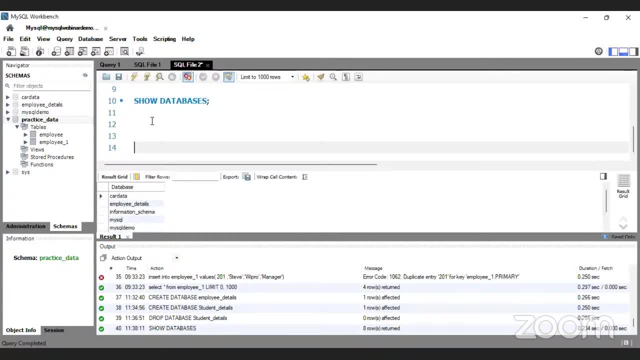 So while I'm here, So basically I'm trying to create my table inside a practice data. OK, So how do you make this practice data as a default database? So basically, when you deal with There are different databases and you should be aware that in which database you are doing. 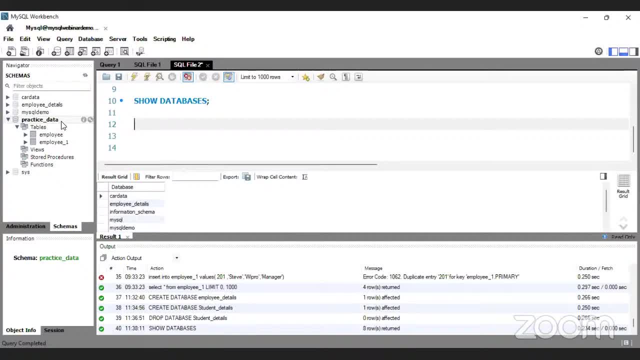 In which database you are creating a table. So you have got an access only for practice data. So what I do, The easiest way, is you can just right click on that practice data and you can see set as default schema. That is the one method. 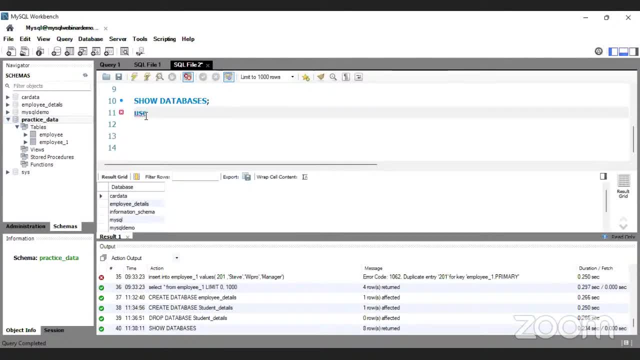 Otherwise you just have to use, like you have to say use, You have to specify your database name like practice data. OK, Without setting it to a default database. It doesn't work. Make sure you use. either use practice data or else you use. 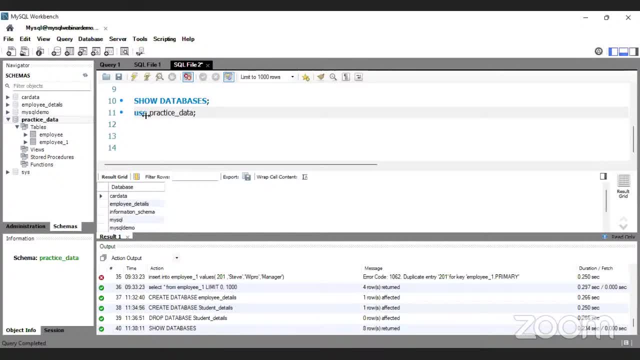 You will right click on the database and you will set it as select default. See, if you click on the select as default schema, So that will be the default one, And whatever operations I do, entire thing will be stored inside that particular database. 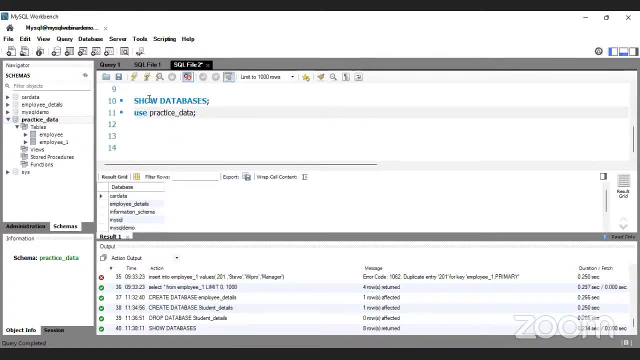 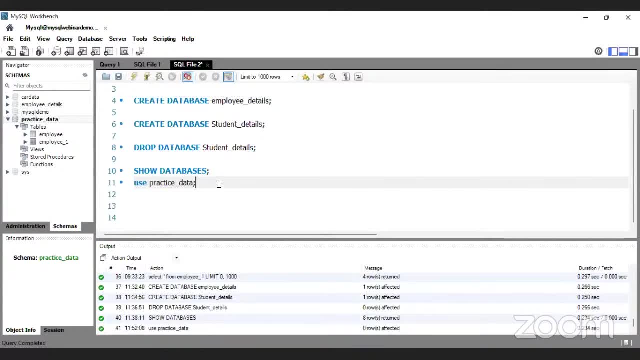 So let's see It's used database. OK, Already, I have made it like I have said that I've started to the default one. It's OK, Let's run this as well. Yeah, So what is our main focus now? 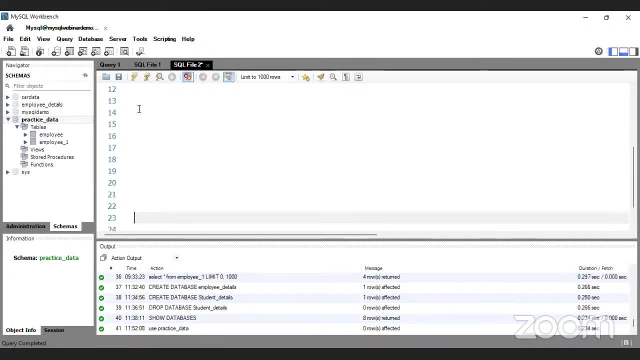 We are basically trying to create a table inside of practice data database. So what is the keyword for that? So I need to create a table. It's going to be So: create table. And I'm trying to create a table as employee. 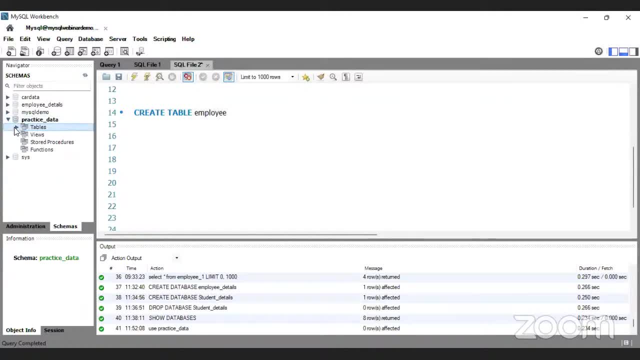 But let's see, Are there any tables inside this? Oh, it's employee one, employee two. All right, So I'm creating a table with, Let's say, employee data. This is my table name. I'm creating a table with a name: employee. 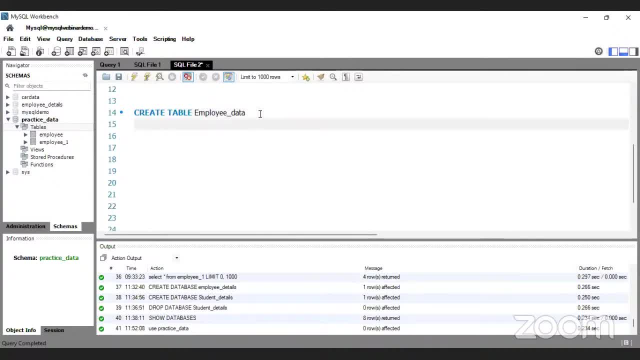 Data. OK, let me close it. Oh, not closing. So done So create table and you need to specify your table name. And now you need to start giving back, You're right. So how do you do that? So just open bracket and inside. 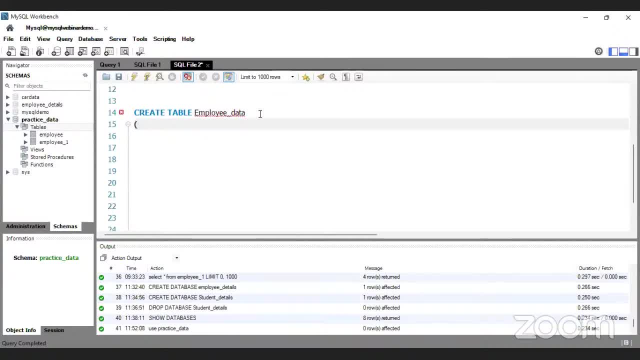 You have to specify the values that you need to do like that, You need to create. So what was your table? Its employee ID was the first column Right And name: company and a job. So let's create it. yeah, so it's going to be creatable employee data, so i need to specify the column name, the 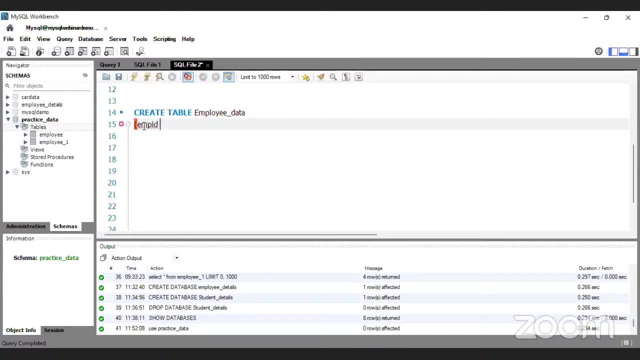 first column name is employee id, okay, and the data type it's basically an t2, let's say int. okay, come on. my second column name is name, so name is basically takes kind of data, so it's name and i'll specify the varchar. data type is character, so varchar of let's see some 30, 30 characters. okay, and then it was a company. 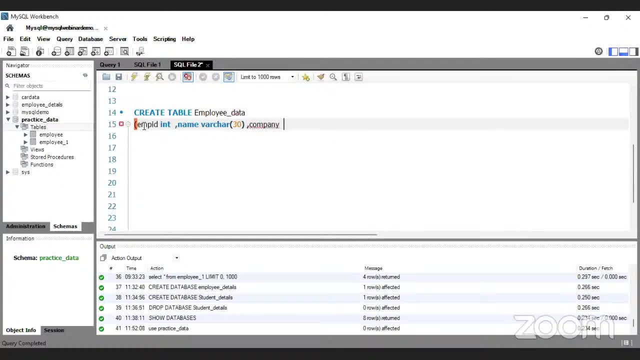 so let me create a column and the one which is company and let me specify the data type that is. even this is a varchar. that is because company name will be in a text, kind of thing. so let's see 30 itself, and the final one was job. 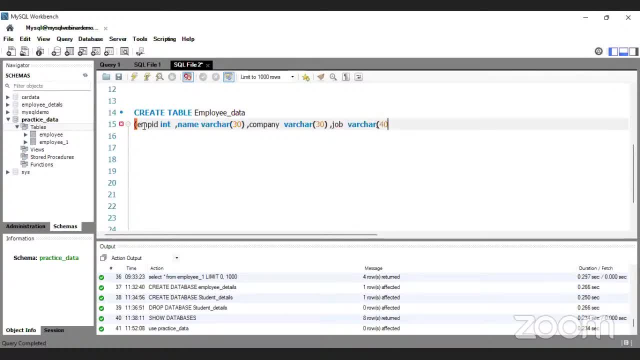 and the data type. even this is varchar. you can also use character as well. okay, yeah, so this is how you will create a table done with it. we started with a create table keyword and then we specified the table name and then i have specified the column now. 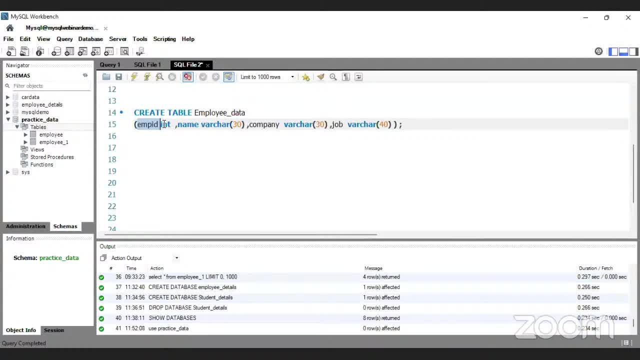 column number one- that is the first column- is employee id. employee employee id takes entry to value, so it is int. and then it's going to be the second column, which is name and the data type is varchar and the company varchar job is also a text kind of data, so i took 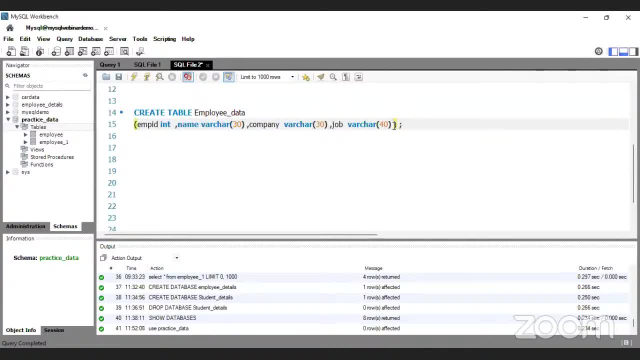 40 and do you want to specify any constraints? let's see, employee id has to be not null and it should be unique, right? so let me give primary key. so it's just a primary key and within a bracket you just need to specify employee id. yeah, and make sure you close the bracket here. 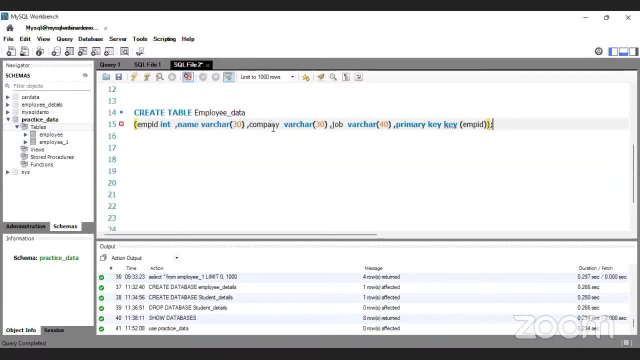 so no error, if it's any, i'll make sure. even this is e, so it's giving many giving me a nearer because the key is repeated twice, so just remove one key. oh, sorry, so you have to remove this key. yeah, now it's perfect, so let's create a table. just run the cell. 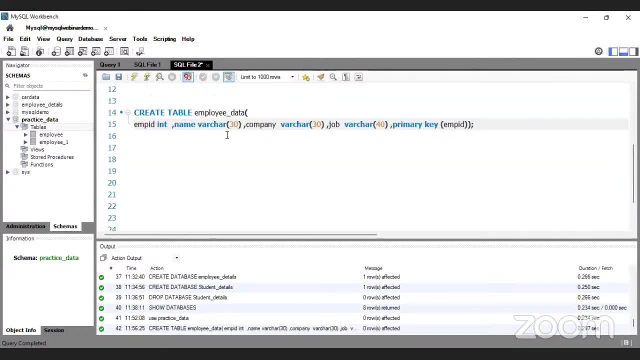 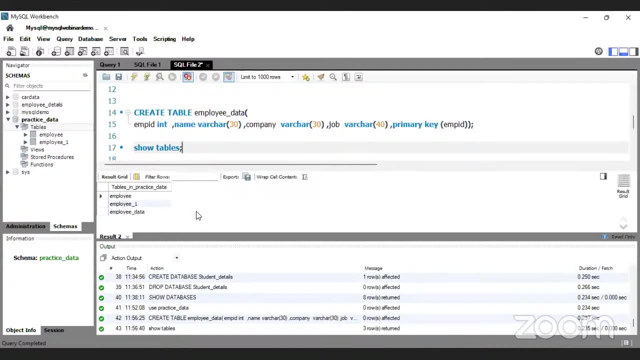 so it seems like table employee data is created. okay, do you want to see, like, how many tables are there in the table? will you have to write a table? this, it's just show tables and let's run it will show you all the existing tables. so right now i have created employee data. 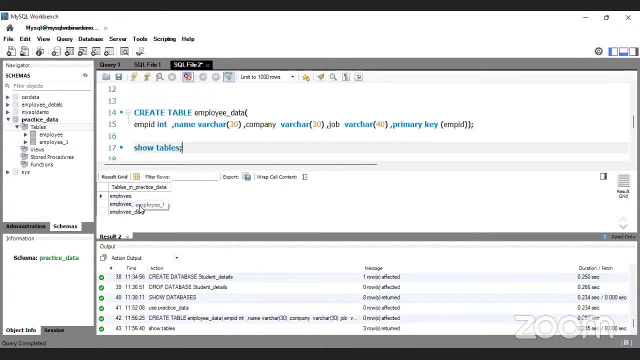 and before that it was like two other tables like employee and employee one. the way you see show databases. same thing has to be applied, even in order to see the tables. so this is how creating table is going to work. so we have created a table. that's it like now. 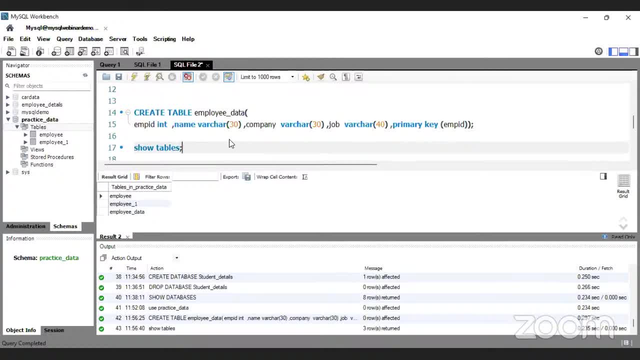 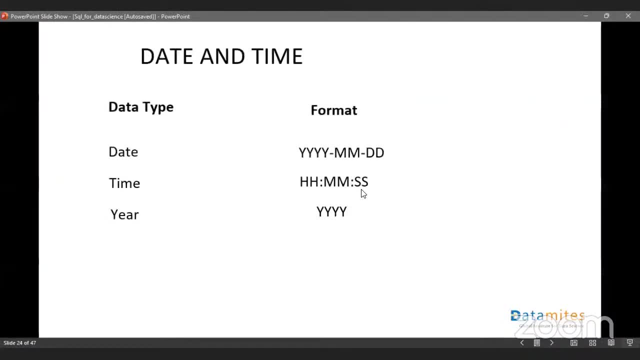 what i want to do is i need to insert values. how do you insert? so for that we have a function called as insert function. let me go back to our prept, so here you can see insert values. i'll come back to the drop later. yeah, let's insert values. insert into is basically used. 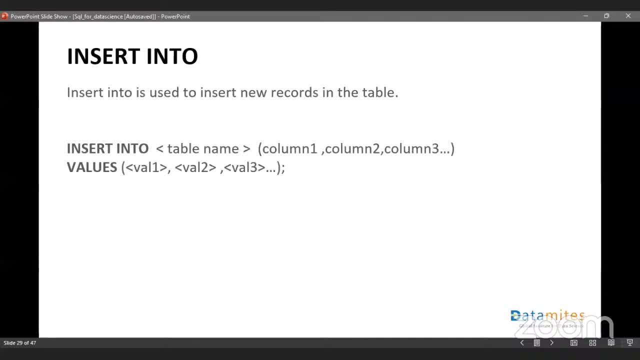 to insert a new records into that table. it's just you have to take insert into and you need to specify a table name. and if you are inserting for all the columns, don't need to specify that column. you can just take employee. that is your table name and you can. 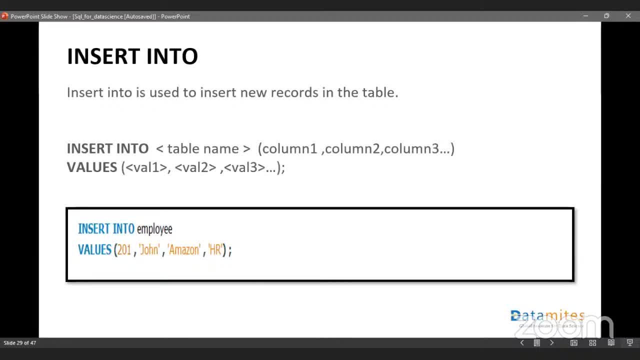 take values inside a couple or inside a parenthesis. you can just pass your values and make sure, if you are passing string data or a character data, that has to be within a single code. so let's see those. let's try to insert values into a table, all right. 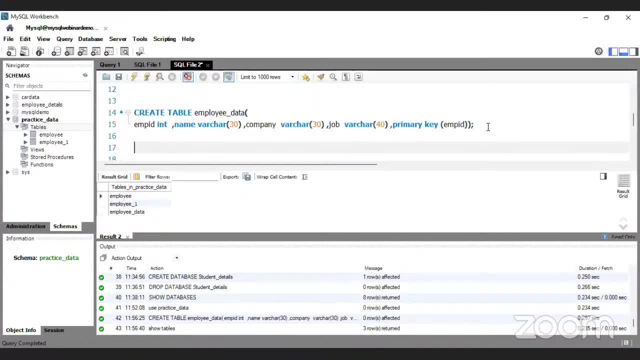 let me go back to our workbench. so i'm basically trying to insert values. so let's say, insert into what i'm basically inserting into our table name called as employee data. this is my table and it has to be values. we need to insert values so value show. so employee id has to be integer, which is 2.1. 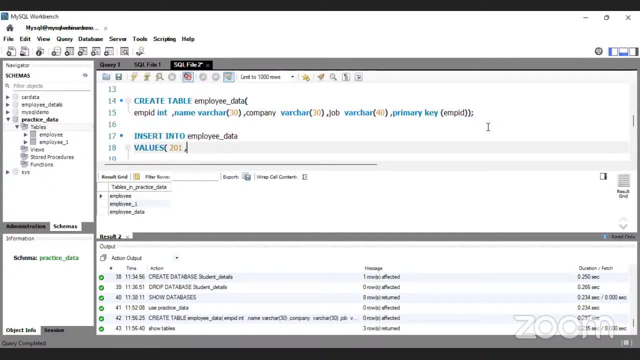 and name. let's say john and company i should give, let's say amazon and i'm going to give it a name. let's say the job, job or the designation is basically: let me see hit chart, just close this and, yeah, let me go. so this is going to insert a record into your table and you want to know like: 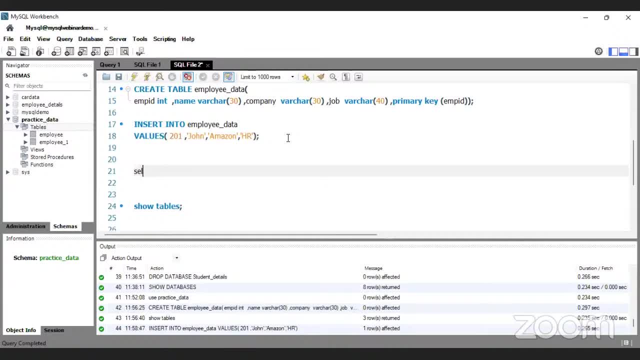 whether it's inserted or not. for that, what we do is we use select statement. okay, we use select statement. it's select. let's return all the columns like whatever it's inside the table. let's select star from employee and then the table from employee. then it's going to insert a record inside the table. 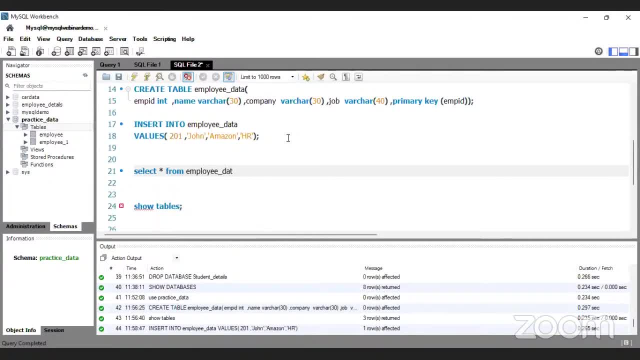 employee table. we'll be discussing about select in tomorrow's class, tomorrow's session. yeah, so it's going to be select star from employee detail. let's run this and let's see whether it has inserted values into it or not, so we don't get any error. it's basically right mark, so it's going to. 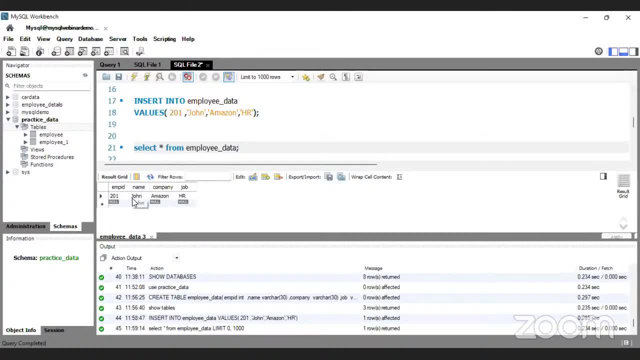 print you the record. clearly you can see. so we have inserted a value like 201 john amazon hr. so the first record has been inserted into our table. let's try one more time. let's insert one more record. so same thing. so it's going to be insert into its employee table, or let's say it's employee. 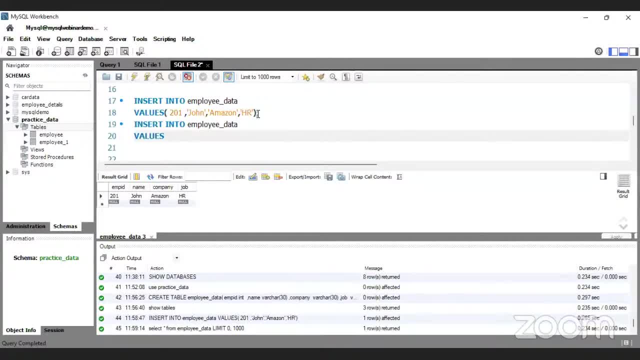 data. that is our table name, and we need to specify the values. and the values are basically, let's take an idea, student or two and name. let's see it's mary, and let's see the company in which she's working is basically google and yeah, and the designation. so let's see which is an id head. 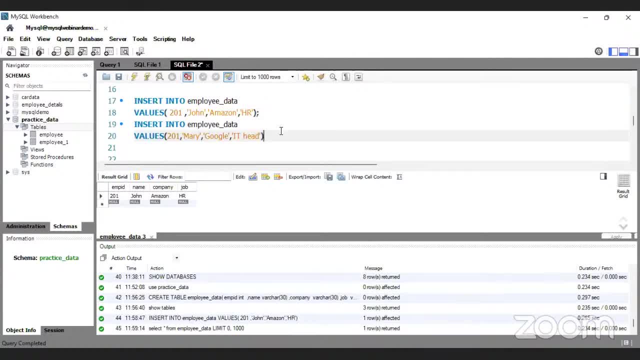 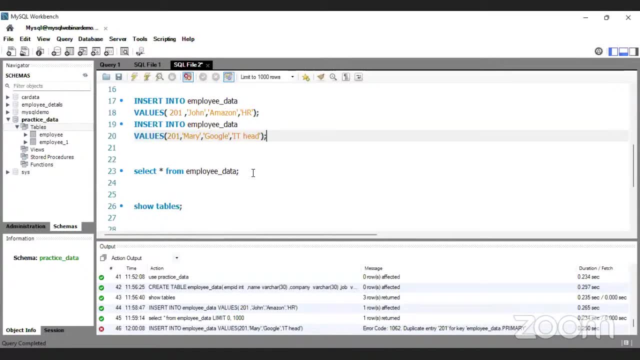 okay, yeah, so let's insert. this is a secondary code that we are trying to insert into our table, so let's run this. so do you want to see whether it's inserted or not? oh, it's giving error. why? no, i wanted to do this, but it's showing an error. can i get a few answers for this? why i'm getting error? 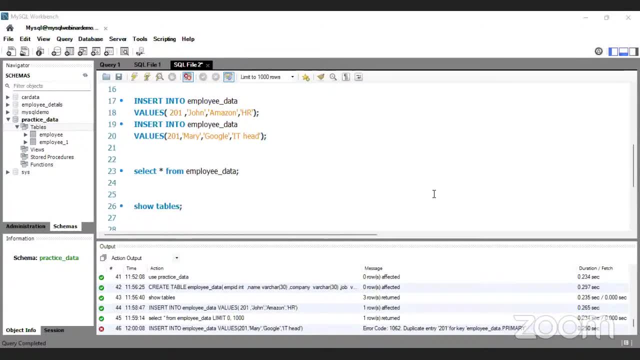 yeah, foreign key declaration has it. yes, so it seems like primary error. so we had given a constraint, like we have restricted, that id has to be not null and it should be unique, but what i did here. so i'm trying to replace or i'm trying to insert record with the same id. that's why it's giving you an error, understood. 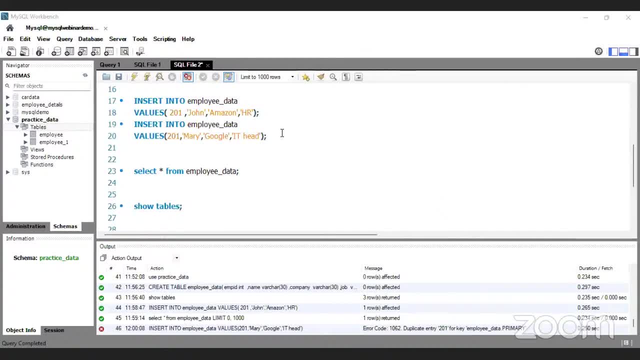 that's how a constraint work. all right, yeah, that's good. so let's run this. okay, let me change the value now. let me change it to two, not three. okay, so let's run this. okay, let me change the value now. let me change it to two, not three. okay, so let's run this. okay, let me change it to two, not 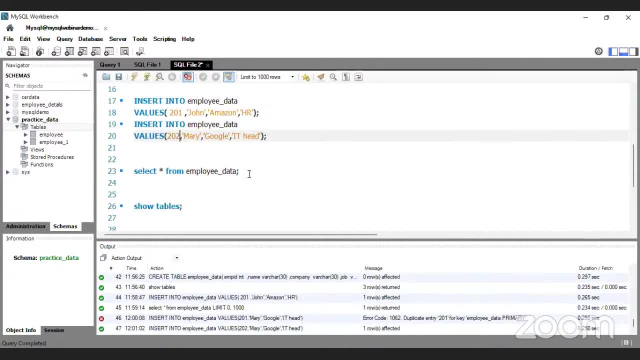 to and let's run this. so now it has to work. yeah, 201 isn't here because it's repeated one and we have specified a constraint as primary key for a employee id. right, that's why. so let's run this and let's see whether it has inserted or not. it's fetching. it's taking time to fetch. yes, so to. 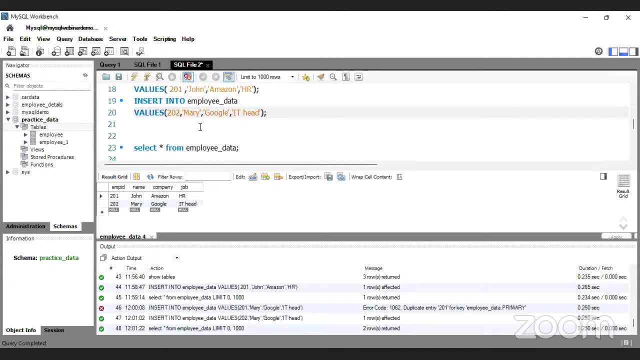 record some inserted clear. so this is how you create a table and you want to know, like, how to drop a table. how do you drop a table? so it just drop. so here is a code. let me show you a code first and then let me come back to this. so insert into is done. so drop the table, just drop table. 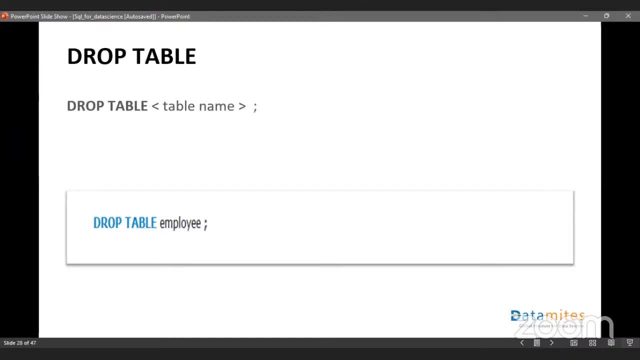 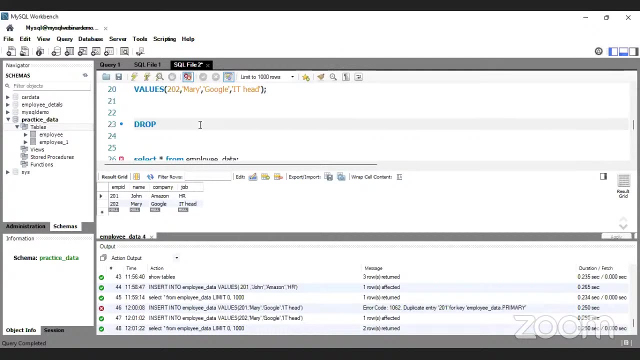 keyword and you just need to specify the table name. okay, so we are not being a data scientist, we are not focusing on creating things, but sometimes you know if you are a data structure, if it's not in a csv format or if it's not in a table structured format. what you have to do is, first you have to create a 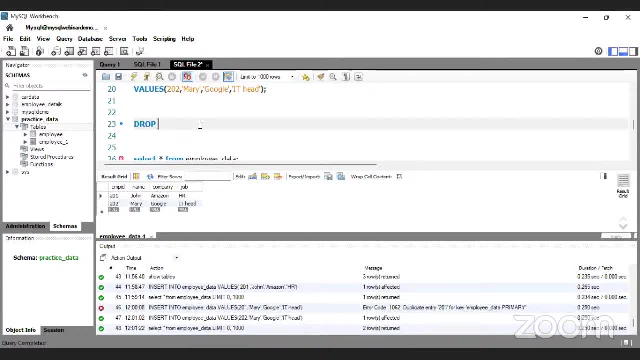 column, you have to create a data type, you have to specify constraint and then you have to dump that table into this database. okay, for that, at least for that knowledge, this is very important. so let's try to drop this employee table. let's drop it. let me drop employee data which we have created. 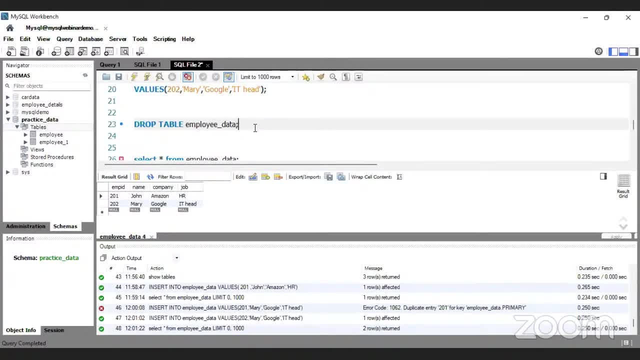 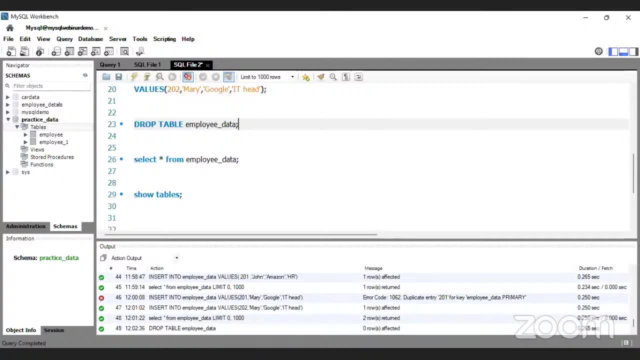 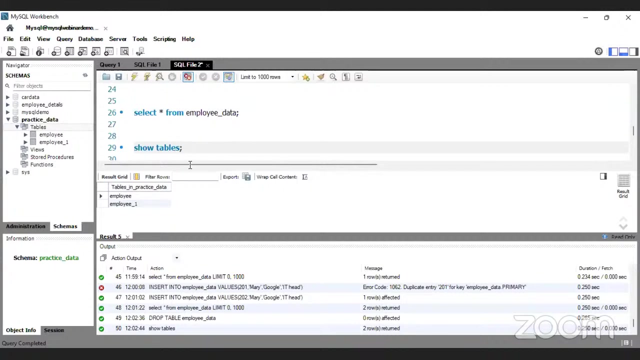 it. yeah, let's drop it. i'm seeing drop table employee data and this is my table. let me run. so, yeah, query has executed. so let's check for the show tables and let's see whether do we have that employee data or not. let's see whether it has remote or not. oh, it's remote, so using drop table. 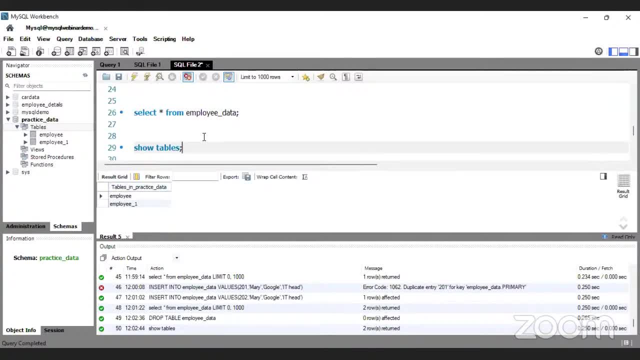 we are going to remove the table here. the database it's drop database for table. let's see how it's going to be drop table and this is show table. so yeah, we are done. we are done for the day. so basically, we did like how to create database, how. 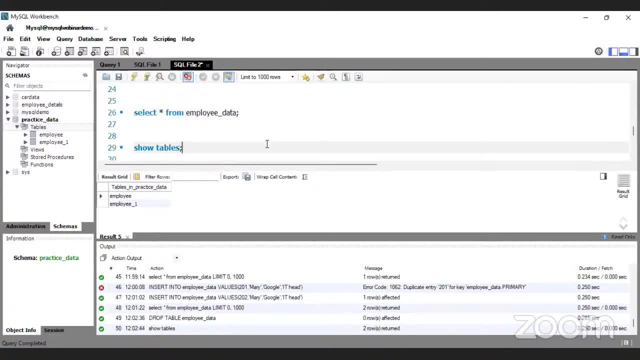 to create a table and also we learned like how to specify data type and also the constraint. so you can explore more on this and from tomorrow onwards- i mean for tomorrow's session- we'll discuss about advanced sql commands such as select, distinct and operator between operator. i'll show you, like how to dump a data set directly into this database. i'll show you and let's take 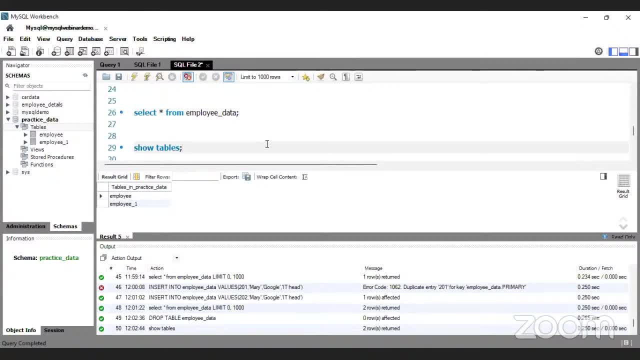 that data set and let's do a querying part. okay, is everything clear for this session and any more questions? if any questions, you can just post it in our q and a so that i can clear it out and then we'll end the session. yeah, or like, if you want to insert a, 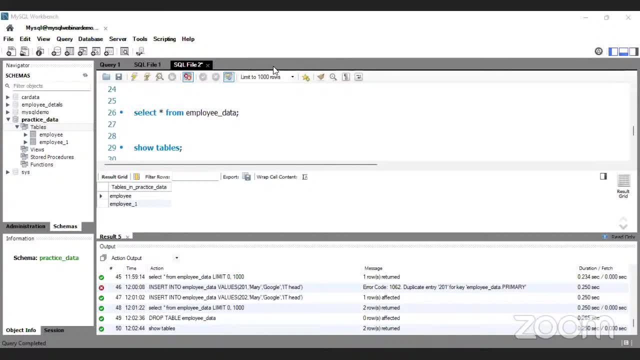 table. like if you want to insert records into a table, you have to write that insert into again and again, so that we don't do, okay, like basically what we do is like we will be having our ready data set. like basically it will be like either csv format or some other format, like what we do. 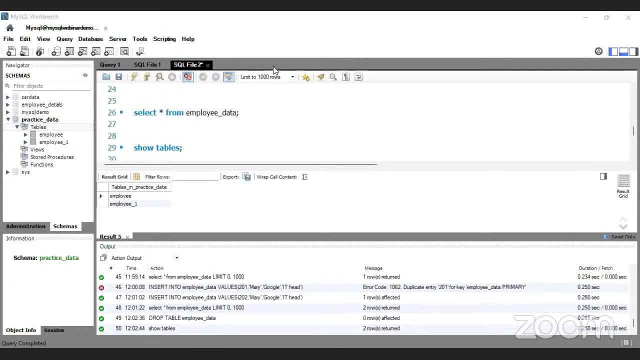 we take that table directly. we uh upload into this. shall i show you today itself, then it will be easy for tomorrow. let me show it again. i'll repeat tomorrow. yeah, so it's very easy uploading a file into this. uh, so this is my database, right? so practice data is my database. 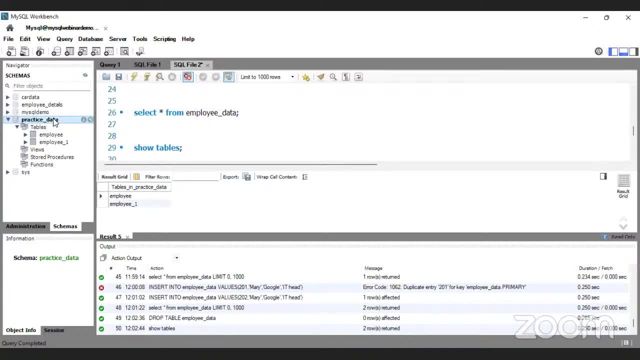 i want to import a data set. okay. so our focus is not basically on creating a database or creating a table. it's just like we basically deal with our data data set and we try to extract things. so what we do is so practice data is my database. just right click on that. okay, just right click on. 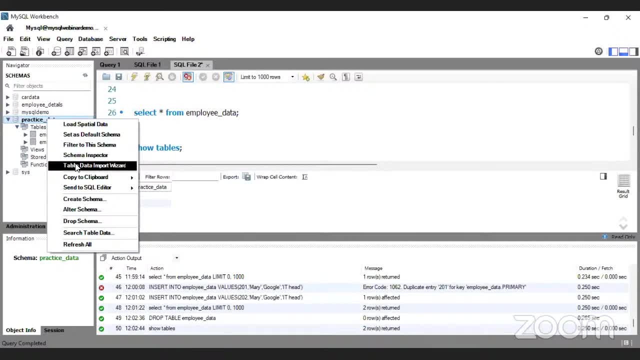 that. what i do is: can you see table data import wizard and select that? this table data import wizard is basically going to help you in importing data set into a mysql workbench. okay, so this is what we do. so let me uh select this so you'll get something like this: you have to select the file path. let's browse from the. 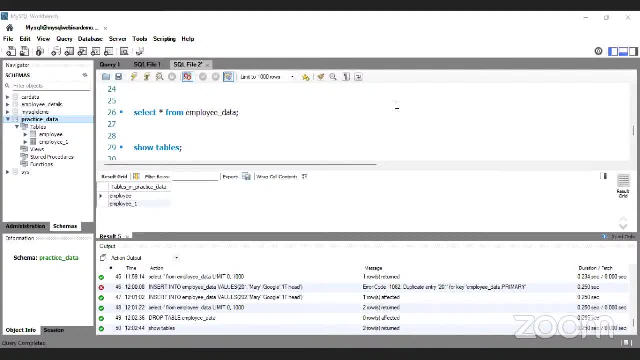 and let's select it from file directory. okay, okay, so, yeah, i have this car data set. probably i'll be using this itself, so let me select this, okay, and let me make sure it's in a csv format and let me open it. okay, so it has selected the path and now you just need to click on next. you can see the steps, right. 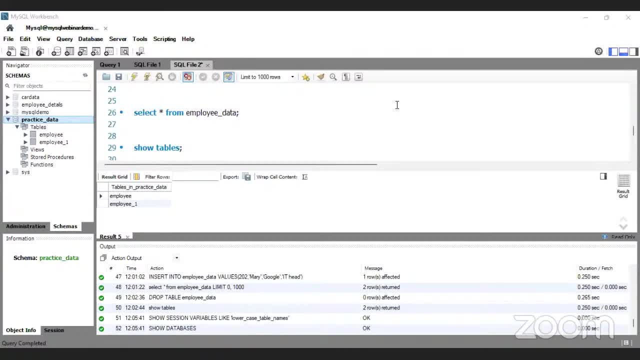 so once this is done, you can just check on. you know, drop table. if exist, so because it's already creating. if if already that you know car data set is existing inside the practice data, so let's drop it. otherwise, like it's, it's already not that. 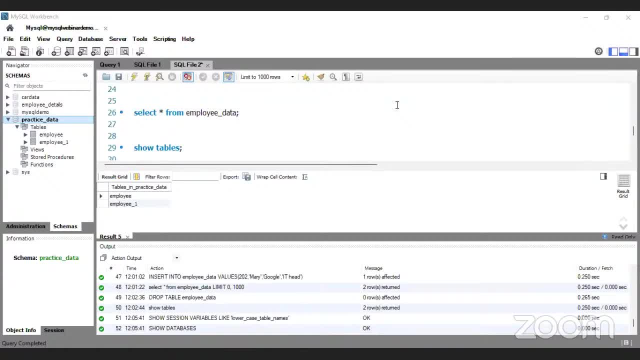 you can just uncheck it, so it's always good to check it now. let me click on next. and yeah, so it will just show you the data type. it's already given. okay, it's in ready data, only like see model. it's text here: it's in teacher price, it's obviously it has to be integer. 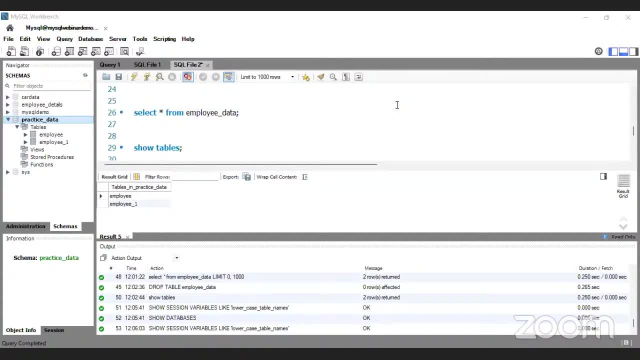 okay, let me click on next. so it will prepare. it will prepare import first and then it will import data file. so just click on next. it will complete these two steps and then it will import a data set into your database. it takes some time, okay, so let's see how it works. 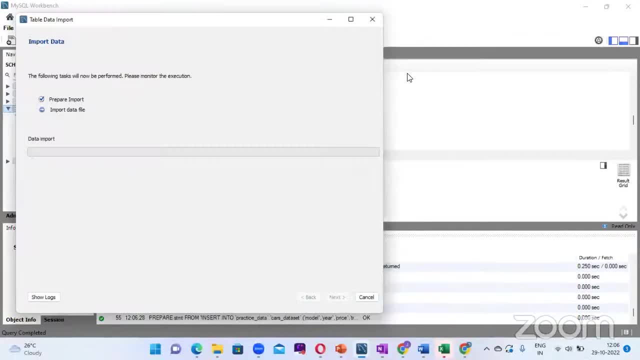 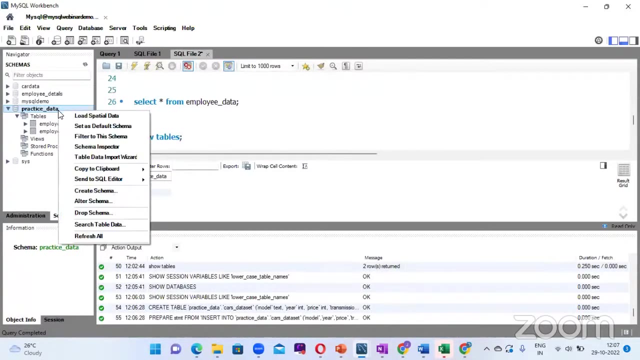 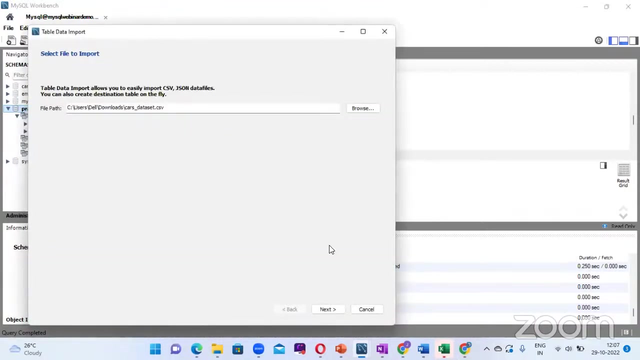 oh, can't see any words, any stuff. oh, sorry, it's one talk. now you can see simple. you just need to select your database, right click, okay, and and you can see a table data import wizard. just click on that, now can you see the screen. you got table data input. 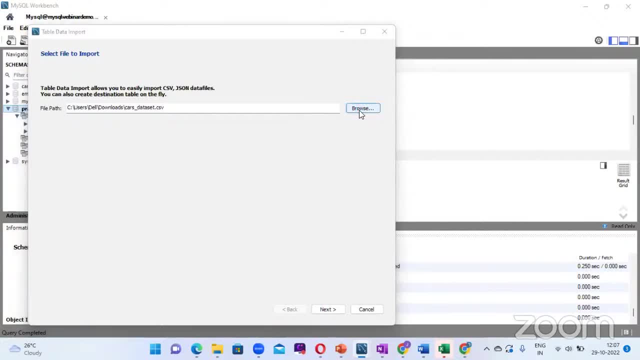 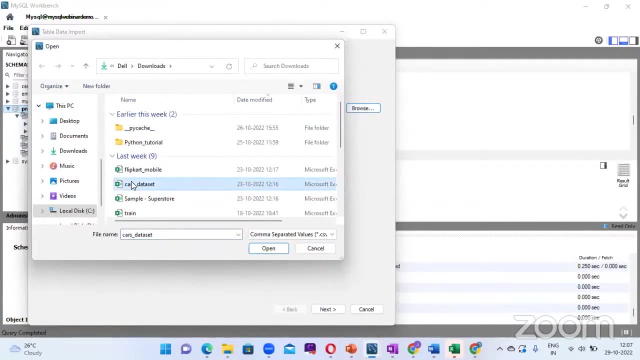 yeah, i think you can see it now, so you just need to browse. if you browse, it will take you to the file directory where you have to select your data set. just click on your data set, okay, like whatever. you have downloaded it, so i'll share this data set prior to tomorrow's session. i'll share the. 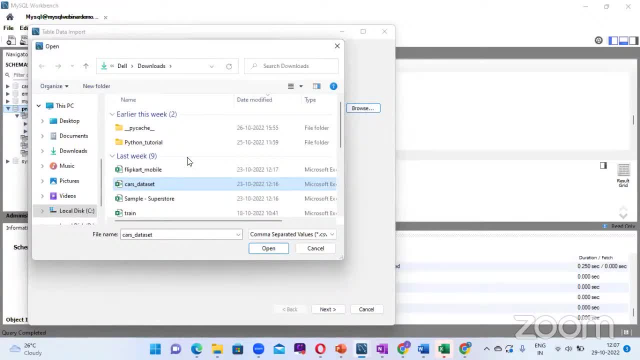 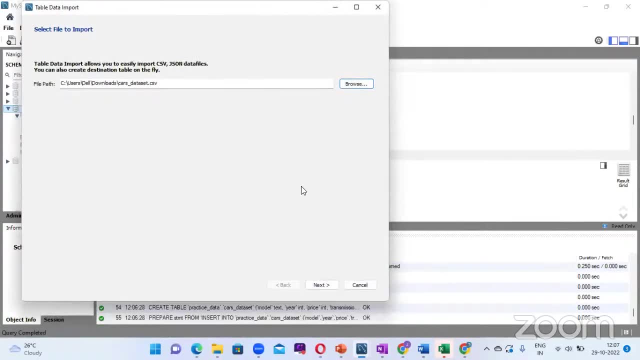 driving, like whatever i've shared right now in the same driving. it will be that, so you can just click on that. click on open and below you can see the next step. just click on next. don't worry, we'll share that data set with you. i'm just showing the steps. 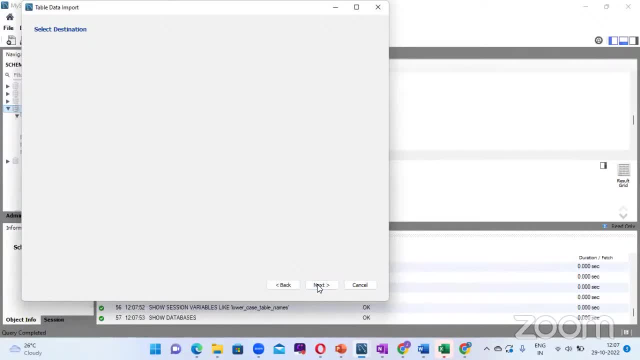 we'll do this tomorrow again- and just click on next. so it's going to show you things like this preview of data set and then, yeah, just click on next. it's going to do the execution for you. it's preparing import, so it has begun import. once it has imported, you will see that car data set inside a practice data set. 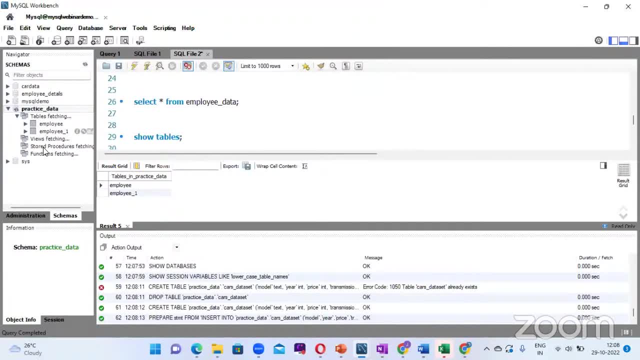 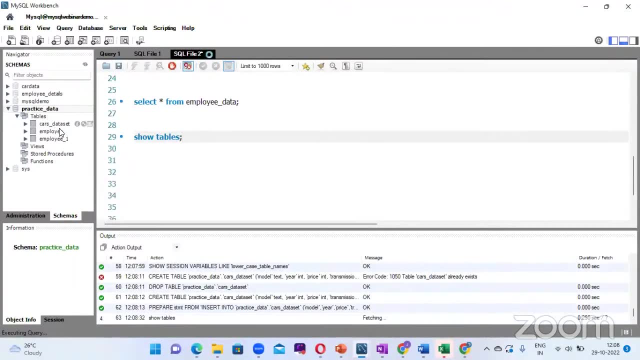 okay, just refresh it. it's still doing okay. once you do this and see it's like, it will show you that table. oh, it has imported it, so we have, can you see? so we try to import the car data sets into our practice database. so we got the things. so car data- the car data set was successfully uploaded into this practice. 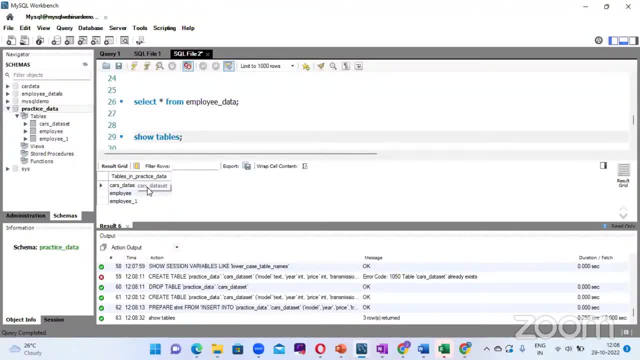 database. so i'll upload that car data set. you can just try uploading. otherwise we'll do it tomorrow in tomorrow's session. so these are the basic things i hope you got to. things like i hope you got the chance to learn like what is database, what are the different data models and would it like what are the different? 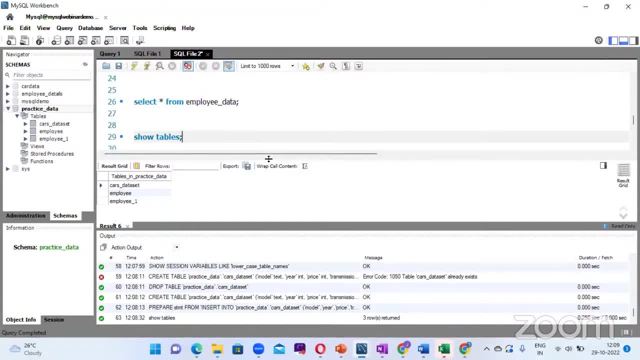 uh, dbms and also databases, and also we discussed things like what is my sql writers and sql sql language, and also we discuss things like mysql workbench and i request you to download mysql workbench before you come for the next session. it's good to do because we'll be doing with sql queries from tomorrow's session, so it's. 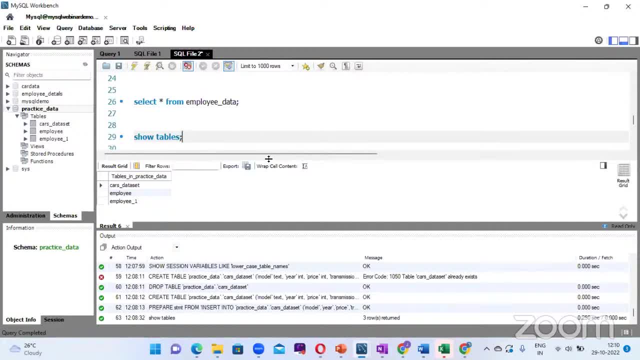 good to have that and also i showed you like how to create a database, how to create a table, and also i showed you like how to import or how to connect data set into a database. so i hope everything is clear for the session and everything is clear for the day. 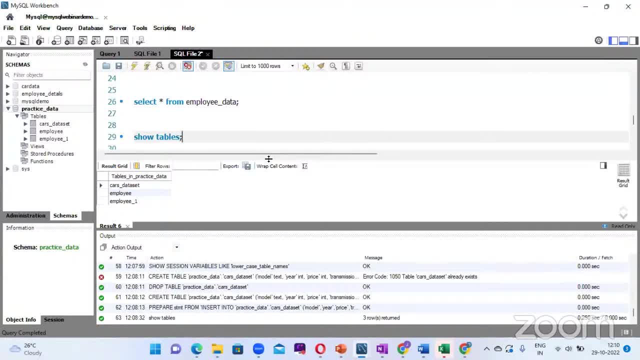 and thank you for coming for the session and let's meet tomorrow. even tomorrow, the same timing is going to happen, with 10 to 12, and the session is going to repeat even for the next week: saturday, friday, saturday and sunday it's for 10 to 12 timing, okay? so thank you so much, jivita, for the wonderful session.